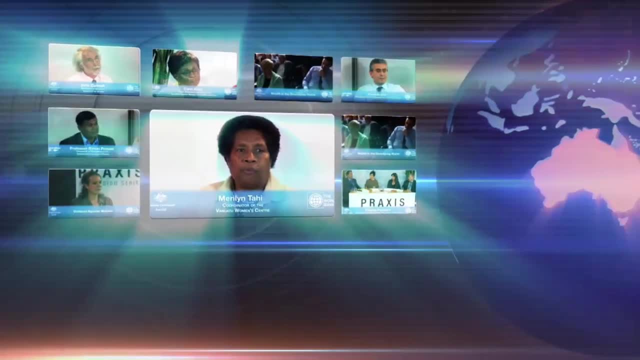 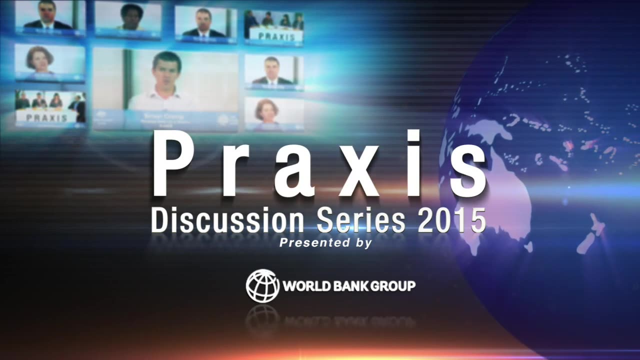 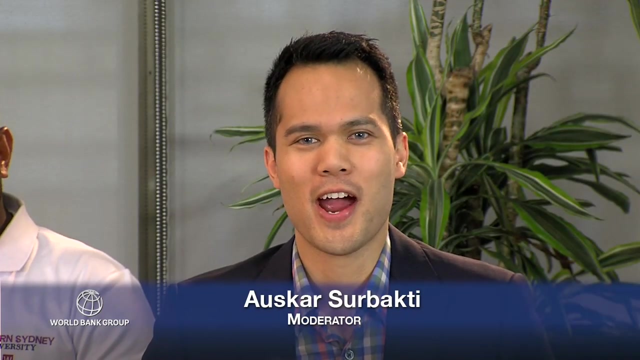 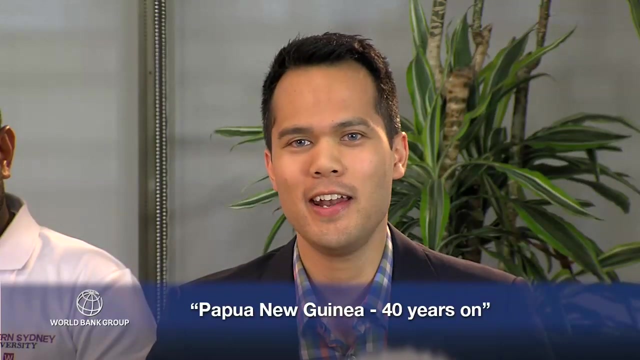 Welcome to the World Bank Praxis discussion series. I'm Oskar Sabakti. I'd like to welcome our audience here in Sydney and those watching on APAC online and listening on radio, and with everyone watching in Dili, Honiara and Port Moresby. And don't forget, you can follow. 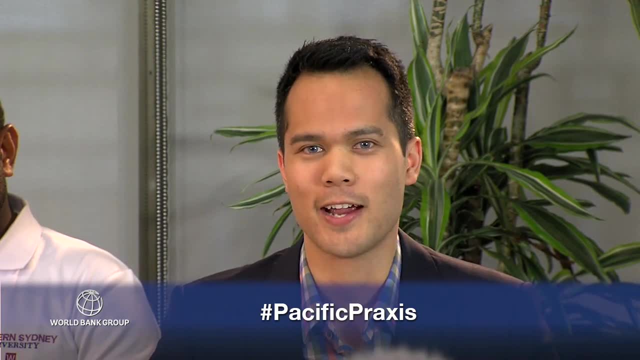 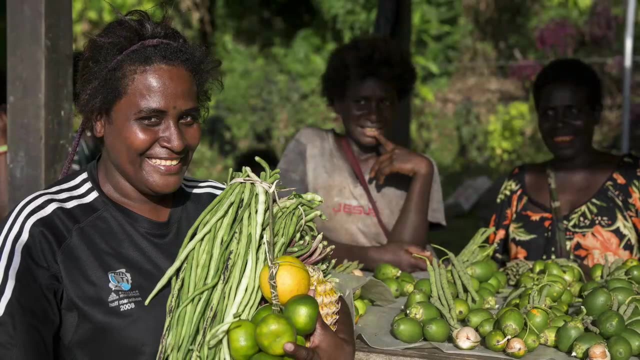 the discussion on Twitter using the PacificPraxis hashtag. Well, this month, Papua New Guinea celebrated 40 years of independence, providing an opportunity to reflect on how far the nation has come and to consider the challenges that lay ahead As the Pacific's largest country. 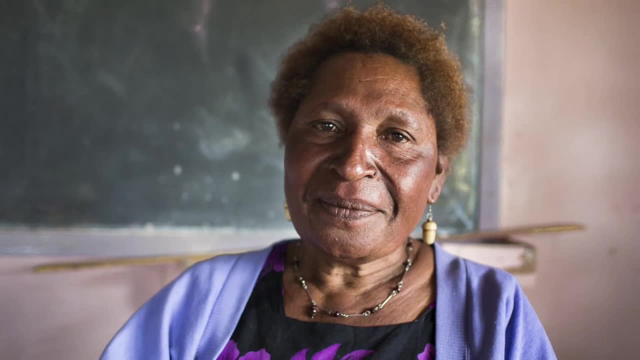 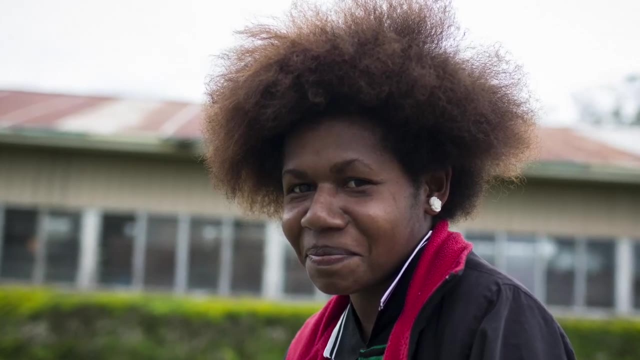 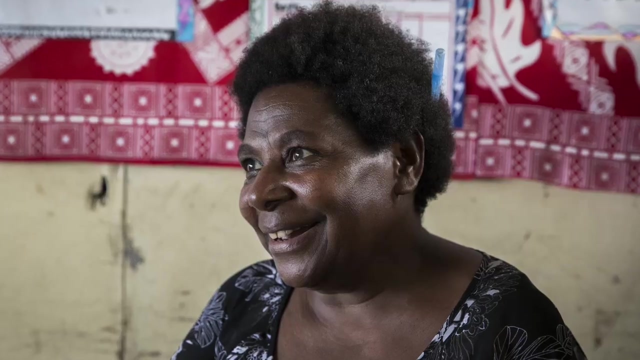 in size, population and economy. Prime Minister Peter O'Neill believes PNG is entering a period of change never experienced before. Papua New Guinea is also securing its role in the region as not just an economic leader, but as a driver of the broader regional policy agenda which will be on display when the nation hosts the APEC Forum in 2018.. The nation 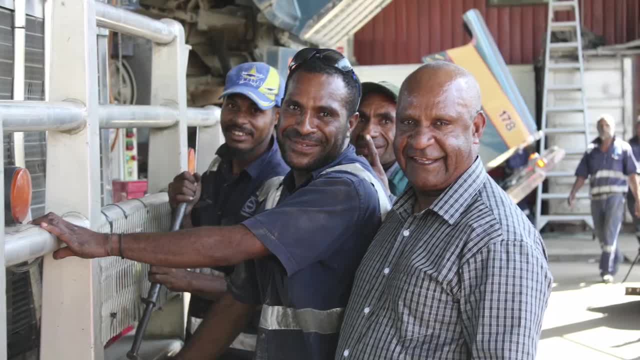 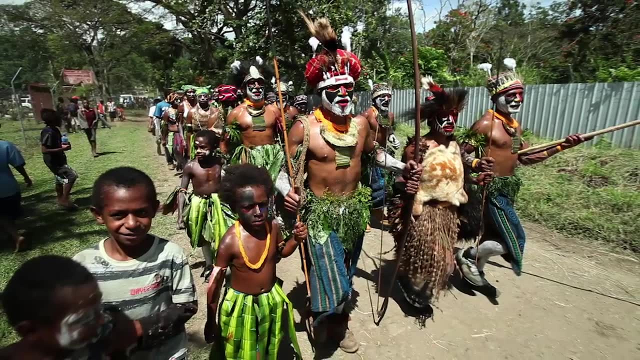 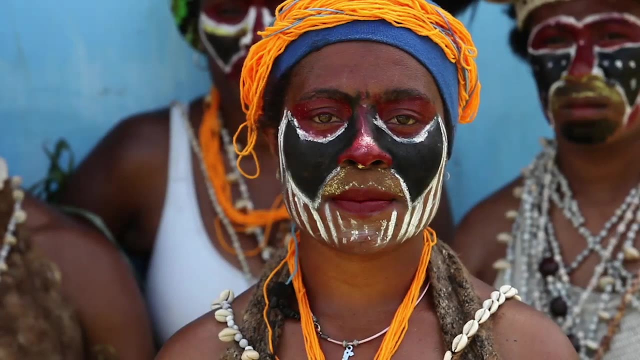 also recently hosted the successful Pacific Islands Games and the Pacific Islands Forum, which is now chaired by Prime Minister O'Neill. So what lies ahead for PNG? Will the government's 2050 vision plan take PNG forward And how will the nation continue to cement its position? 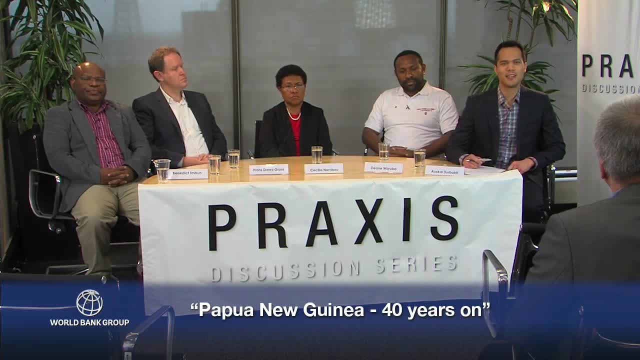 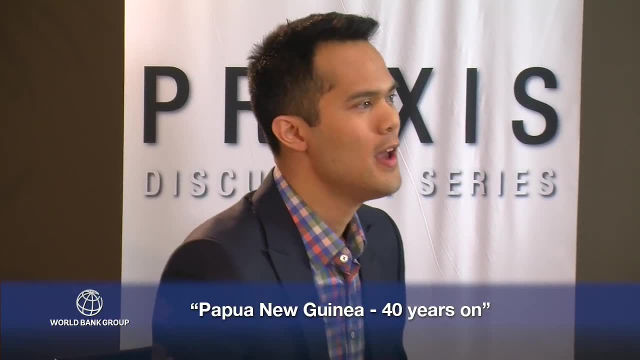 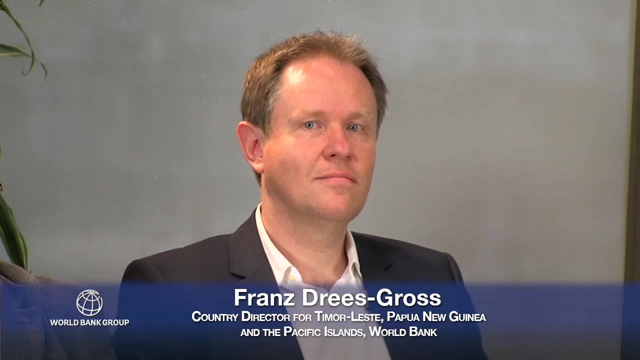 as a regional leader. Well, joining us to discuss these issues and more are: Benedict Imbun, Senior Lecturer at Western Sydney University. Franz Dees Gross, the World Bank Country Director for Timor-Leste, Papua New Guinea and the Pacific Islands. Cecilia Nembu, Associate Professor. 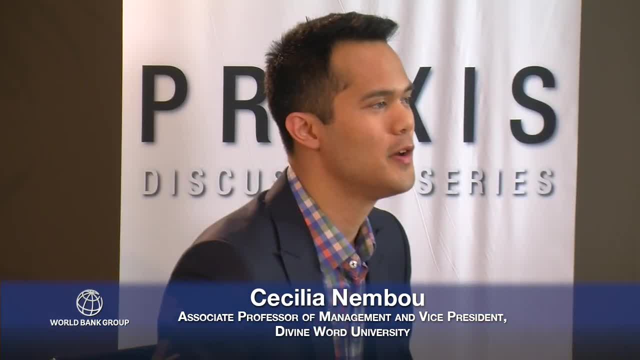 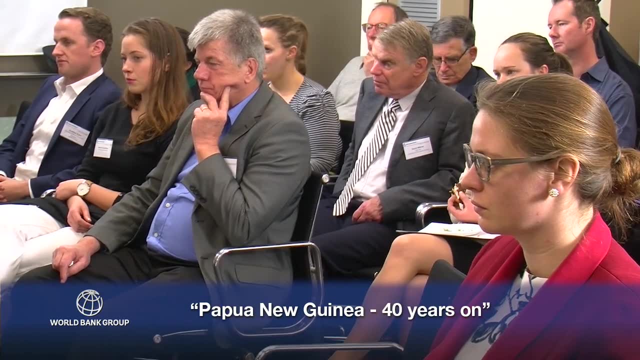 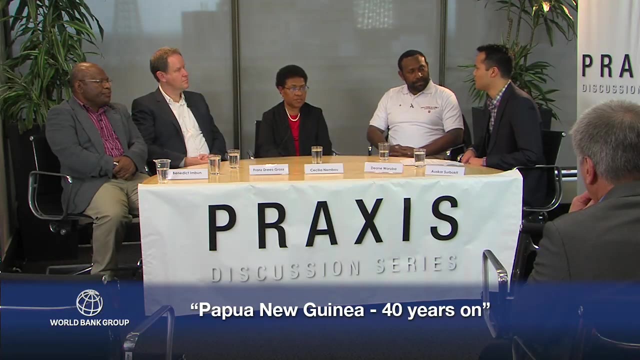 of Management and Vice President at PNG, And Dean Woruba, PhD Candidate at Western Sydney University. Thank you all for joining us. So, as we all know, PNG has celebrated 40 years since it became independent from Australia. Some of you went back home to witness the celebrations for yourself, Cecilia, if 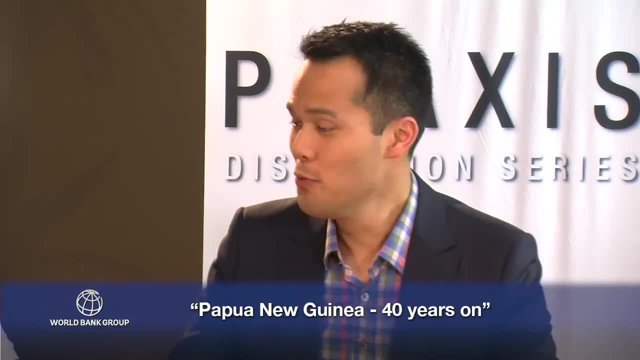 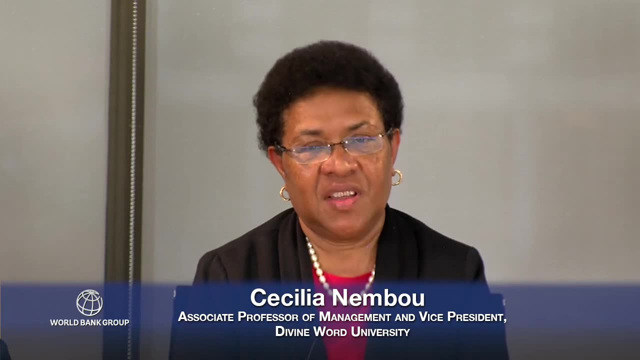 I could start with you. You were there, you lived there, obviously. How were the celebrations? The celebrations were exciting. It was a very special time for me. It was a very special time Exciting, in the sense that everyone was engaged in it, from the little children. 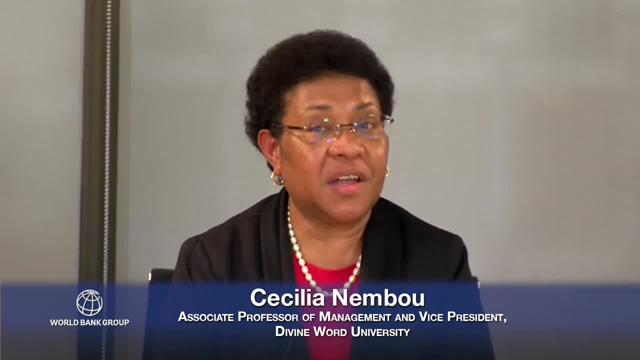 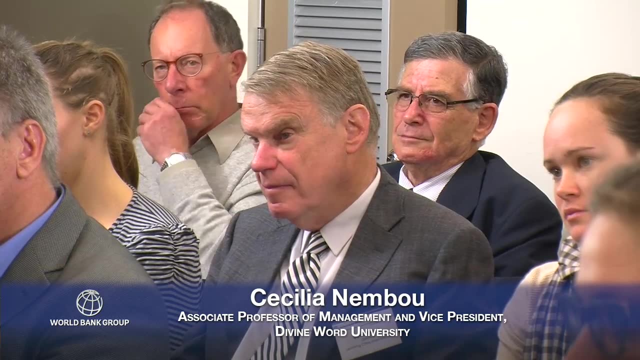 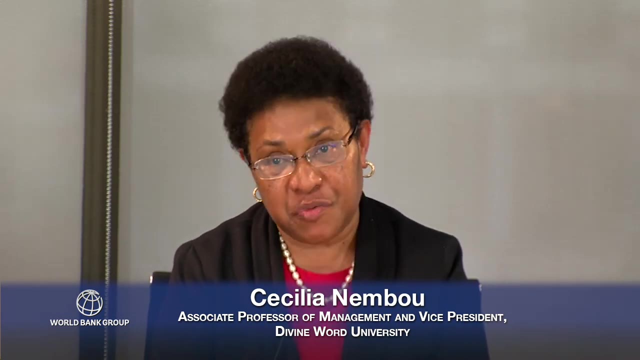 up to the adults. I think you know we have come to a stage where the people actually are together. When it comes to big celebrations like the Pacific Games and the independence, the people are together. They actually show this sense of unity We pride ourselves on. 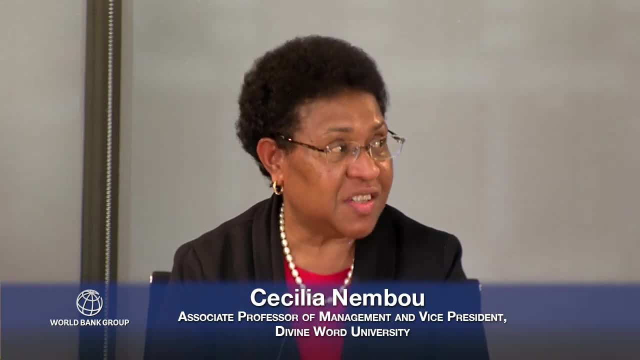 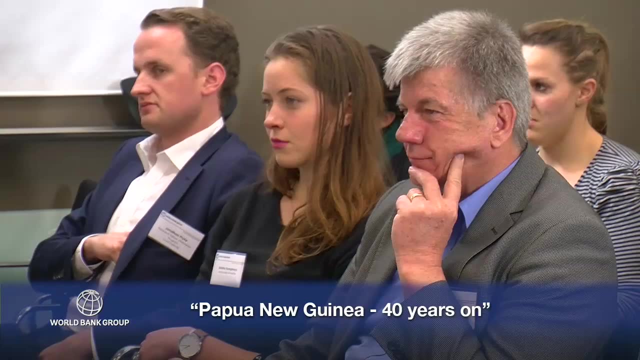 unity and diversity. You feel that during our major celebrations. So I think it was everyone was involved. I'm particularly impressed with the school children. The schools actually get the children to dress up in their traditional costumes And the day before independence. 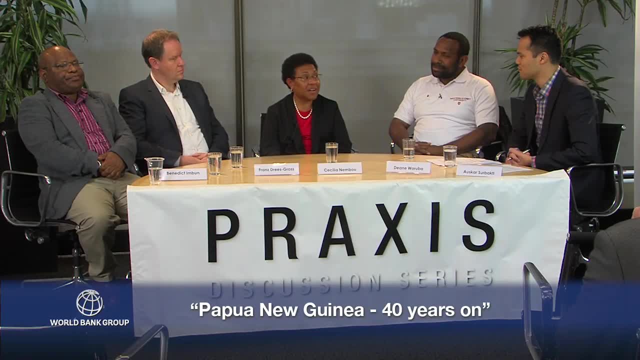 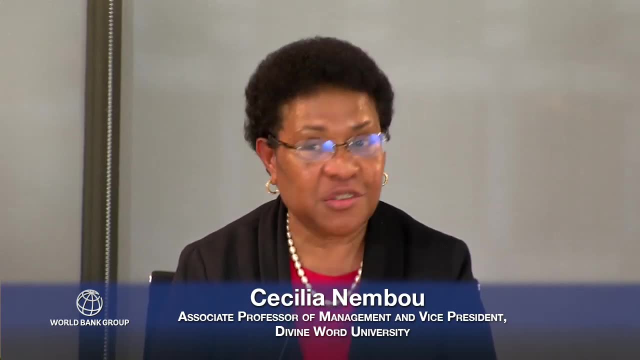 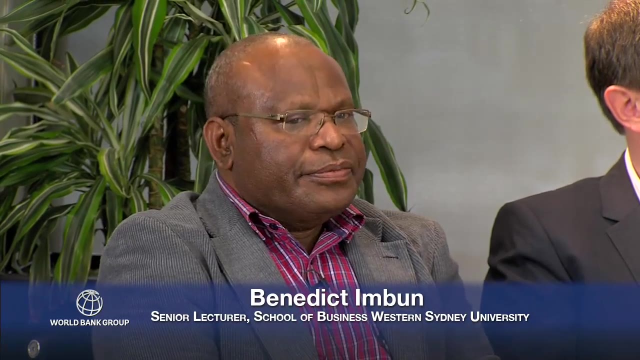 that day is not, you know. it's actually taken up for cultural activities and displaying their national pride in dressing up in their traditional costumes. So it was great, Excellent, Benedict. you and Cecilia are among, I guess, the first generation of those who 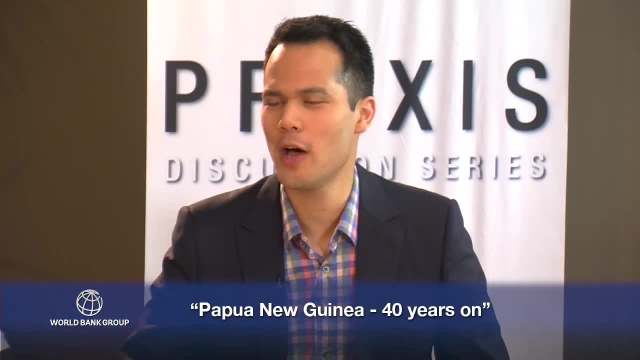 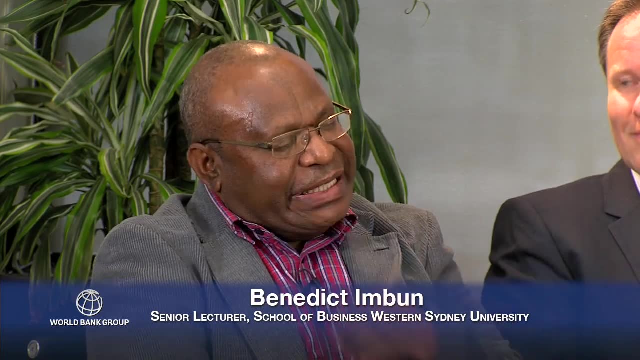 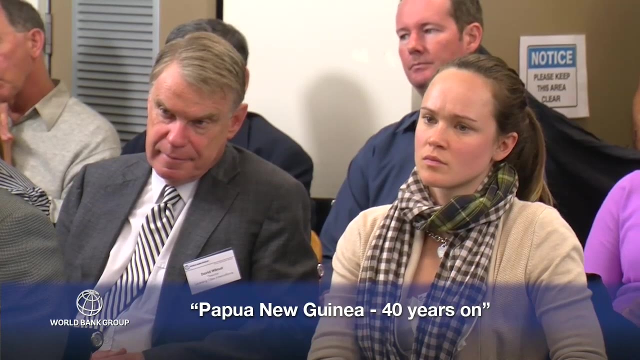 are around since independence, Forty years on, paint us a picture of how the country is at the moment. Well, I can relate to myself. I mean 1975, I was 10 years, 11 years old, doing grade five or six, five or four around that time, And you know, there was excitement, euphoria. 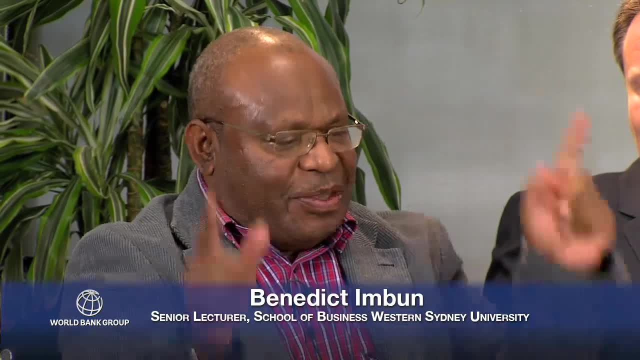 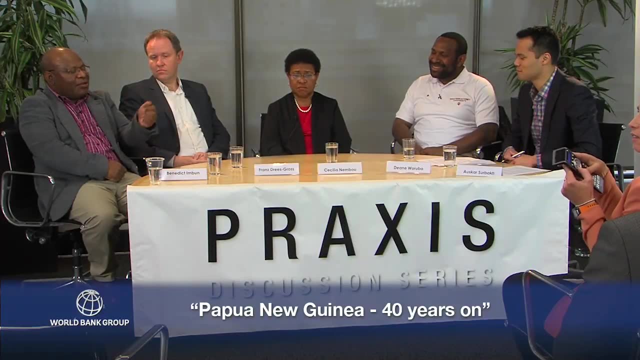 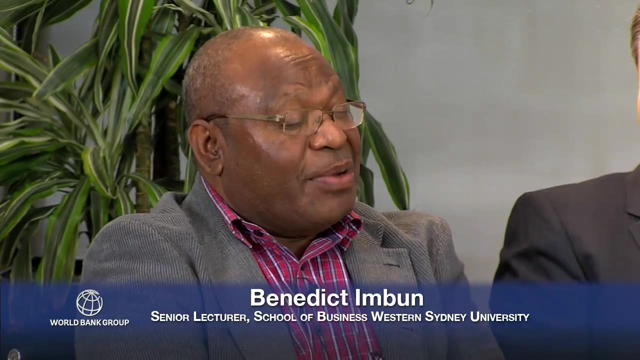 but very little communication. We were getting independence, some of them we were getting underpants from Australia. So there wasn't that excitement in a sense that we were looking forward to something, but that something was utterly. you know could be explained, But I went to high school. 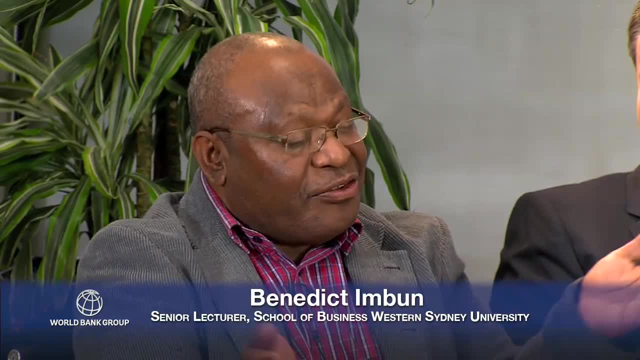 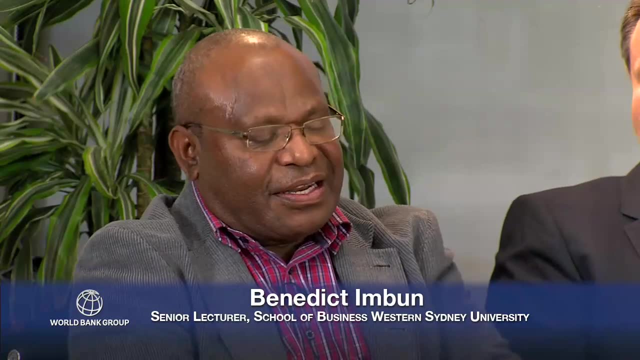 if I can relate it all along, Things became clearer. high school, too, I could get a job because I came from a village. attended a missing school, came to the university, then started university and then became an academic. in the process, came to Australia, attended. 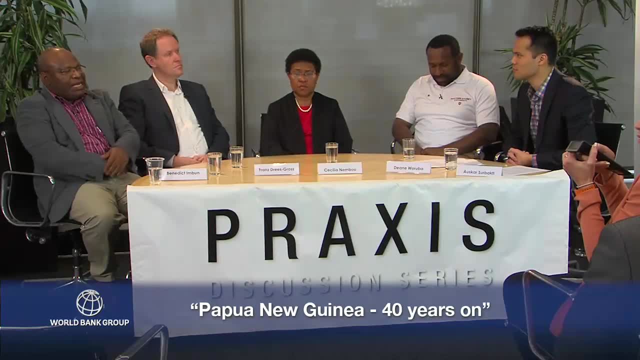 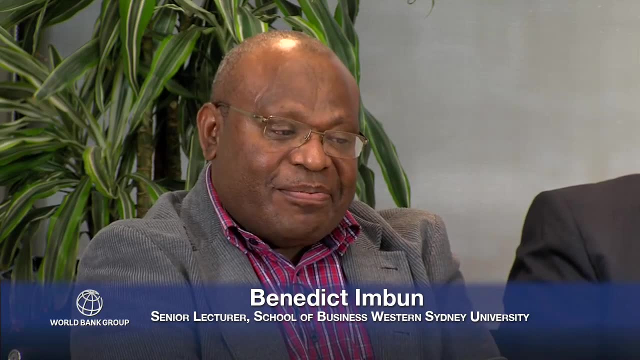 a few universities this year and went back. So in that short span of time I mean I could see we have achieved, I mean, if I'm a testimony to that- 40 years, you know, from a village level coming, acquiring education. 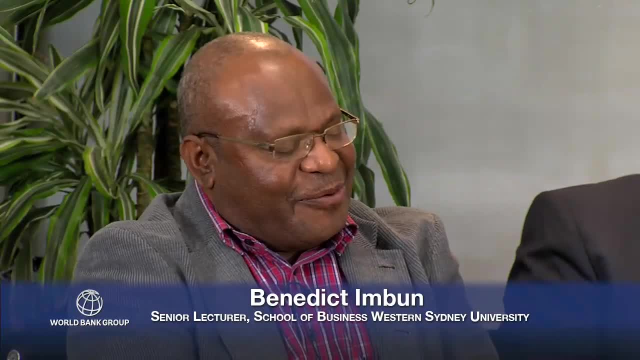 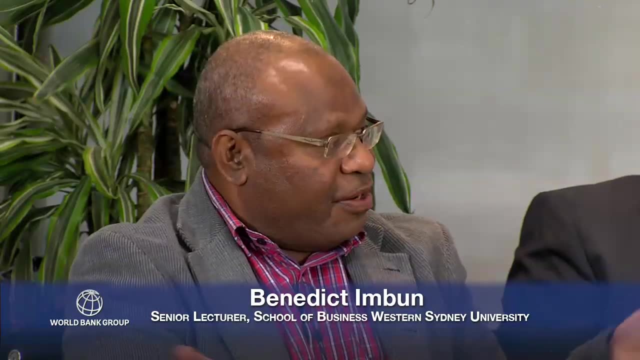 along the years and then teaching here, teaching Australians, for that matter. you know the subject. they like industrial relations. You could see we have achieved a lot, I mean with that, But still we have a lot to do. I mean as the discussion goes on. I mean 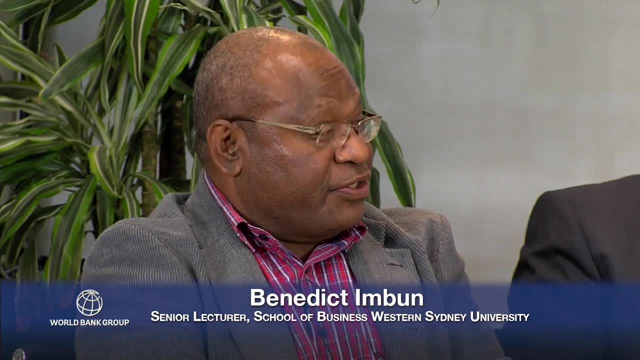 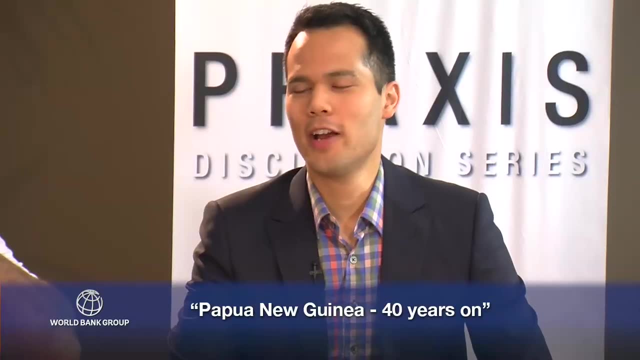 surely others can explain and we can talk more. We have achieved Excellent In terms of human resource development, yeah, But there's more work to be done. That's right, And we will look into those challenges a little later in the discussion. 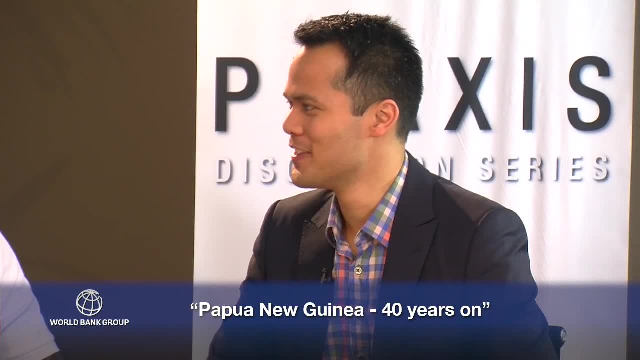 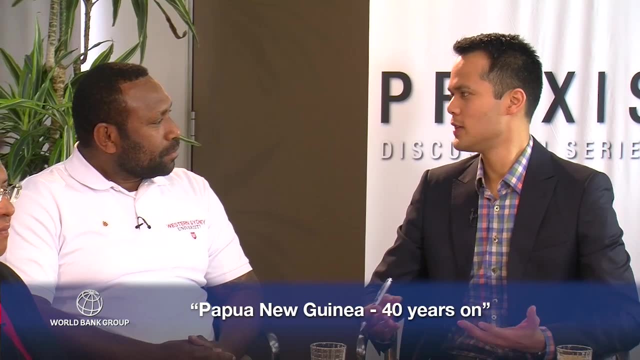 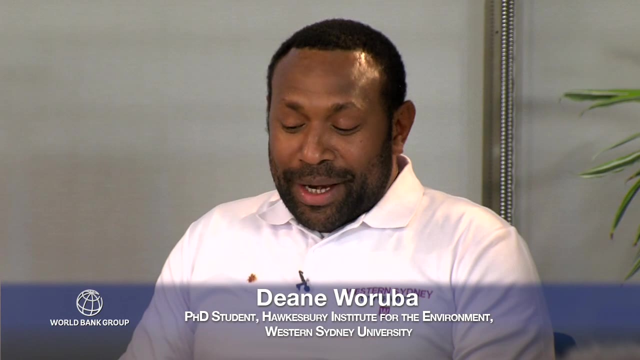 But, Dean, you weren't around, obviously, when PNG gained independence. But from when you were born and from your experience in the country, how have you seen PNG develop since it did become independent on its own? When I was born, we had already been independent. 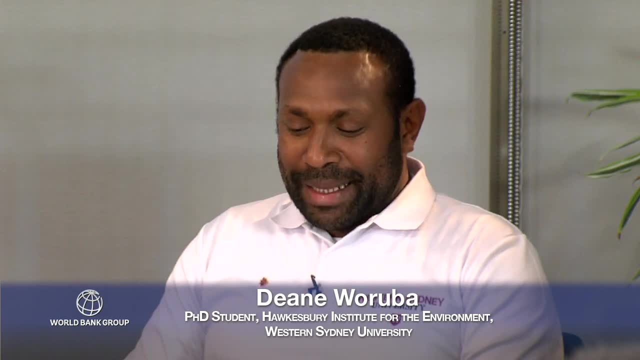 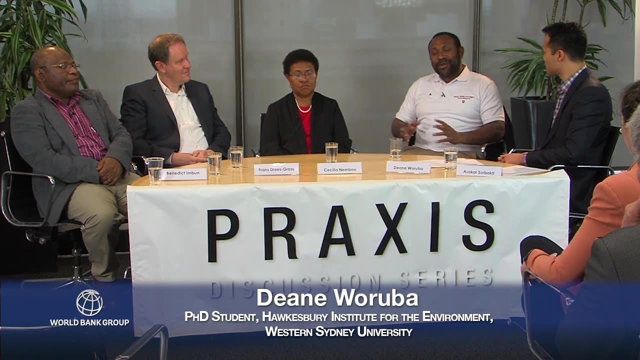 We were independent for about six years And at that time, when I started primary school, I remember on every Wednesday for Mufti Day, I wore a tree bark with leaves. Here I am sitting in this conference, in the biggest city in the southern hemisphere, studying 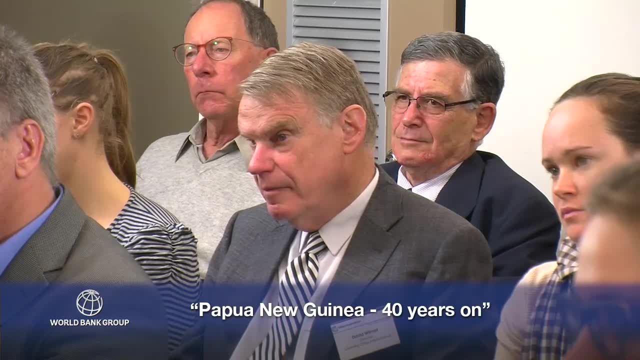 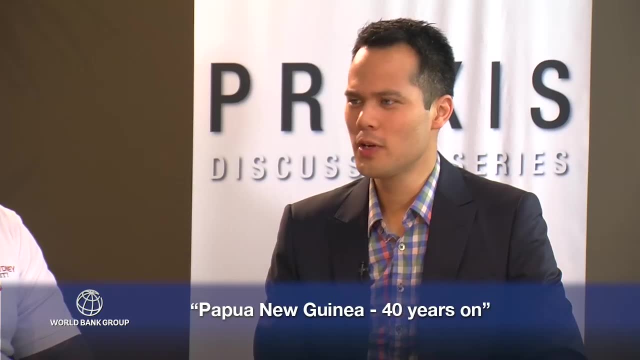 a PhD and talking to you, So you've seen a lot of development in such a short amount of time. Yes, It is hard to believe, isn't it, that it has only been 40 years And you look at a country like Australia in excess of 200 years. 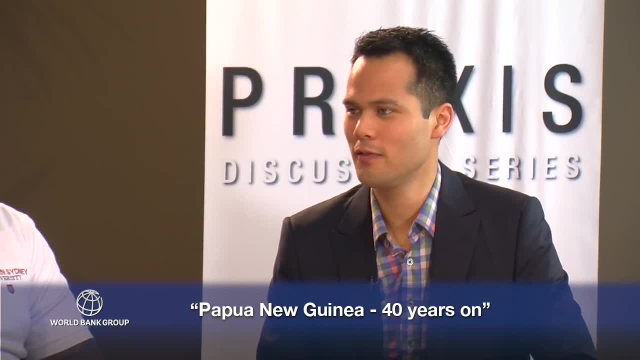 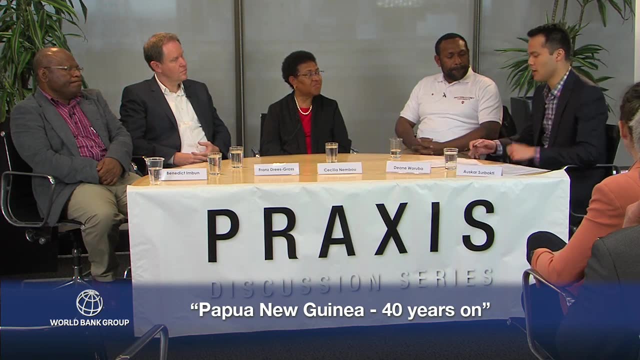 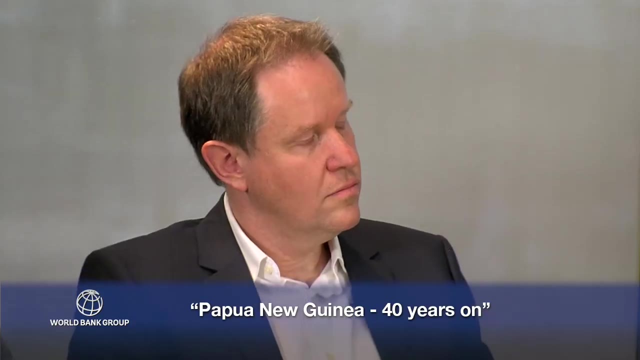 There's still a long way to go, as Ben, you said, And we will talk about that now, I guess. Can I ask you, Franz, from the World Bank perspective- obviously there is a particular focus on PNG- Can you just explain to us what you see as the achievements? I guess that 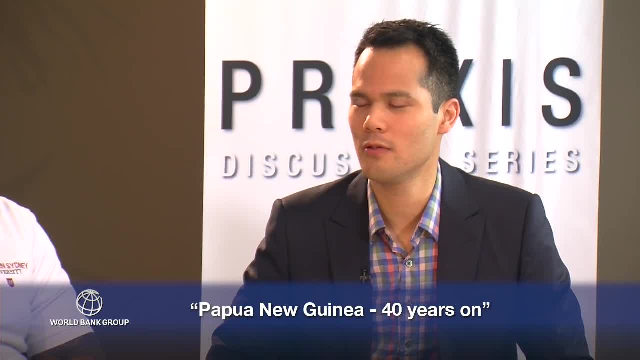 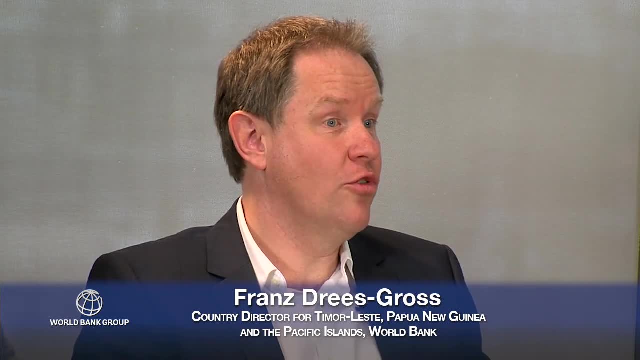 PNG has acquired over the recent years. Let me just say, at 40 years, it is a historic milestone for PNG. Yes, It behooves us to look back and to focus on some of the things that have gone well. first of all, For one thing, PNG now is richer than it was, significantly richer than it. 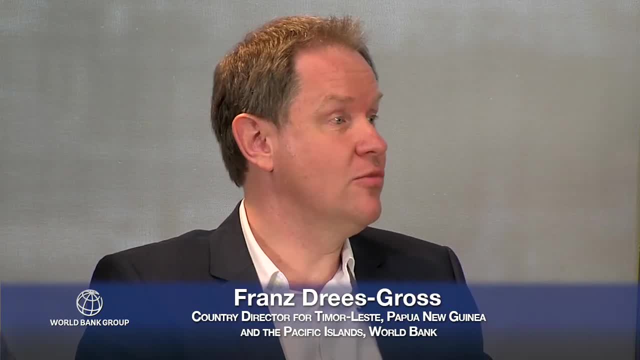 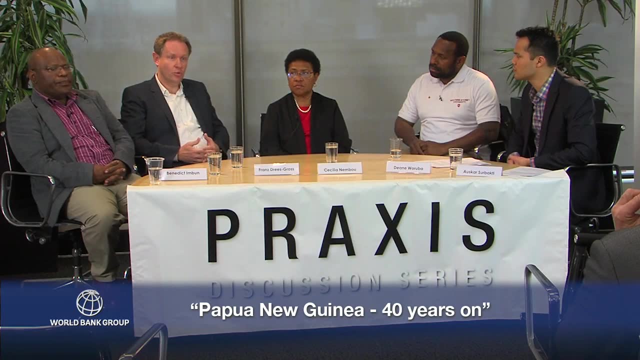 was at independence. At independence, average incomes in PNG in 1975 were about $1,500 per person. We're now at $2,400 per person And while that rate of growth from $1,500 to $2,400 isn't staggering, certainly not by East Asia standards. it is a significant increase. The economy is not only bigger, it's much more diverse than it was 40 years ago. At independence there was one big mine, that's Panguna in Bougainville. Now there's quite. 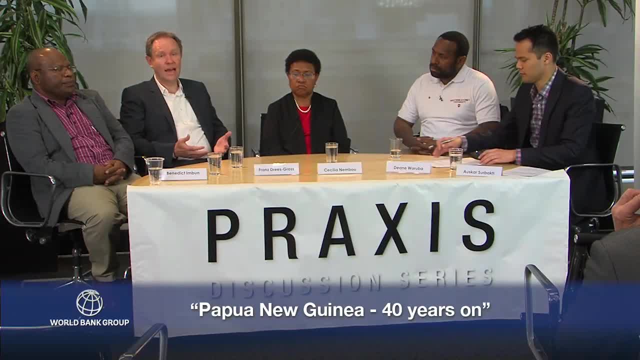 a few of them. There's a number of large mines. There were no natural gas developments at all in PNG. Now there's a huge $19 billion natural gas export project At independence. agriculture meant basically cocoa, coffee, tea and copra. Now, in addition to those, 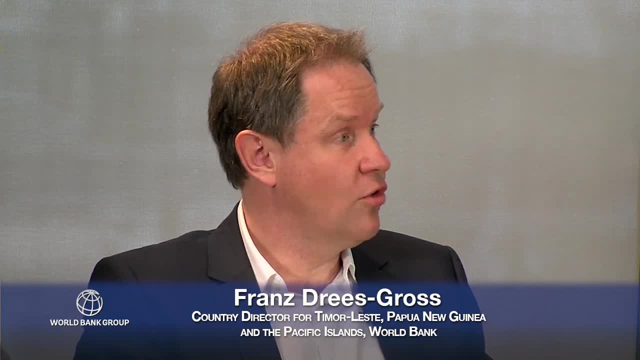 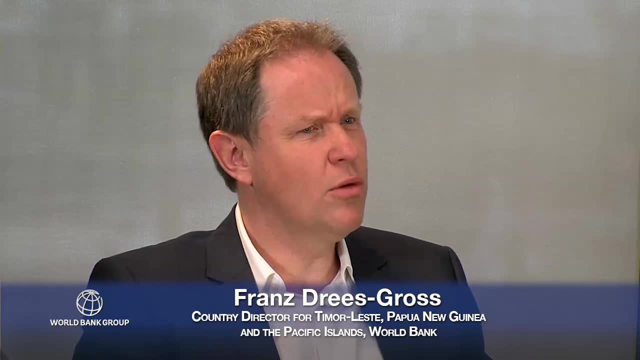 sectors. you have tuna processing, for example. Coffee is 60% bigger than it was in 1975.. Cocoa is 25% bigger. So they're not hugely bigger, but they're somewhat bigger. And there's some others, just some human development, I think. milestones that are impressive. I. 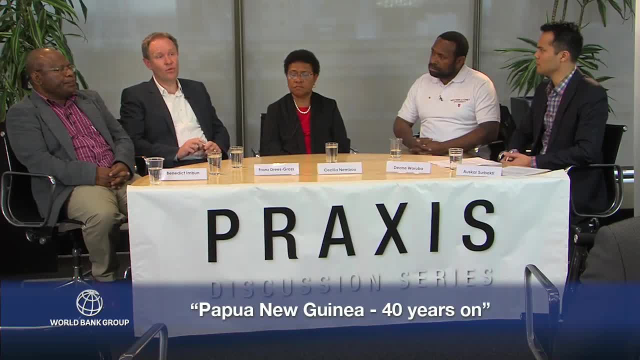 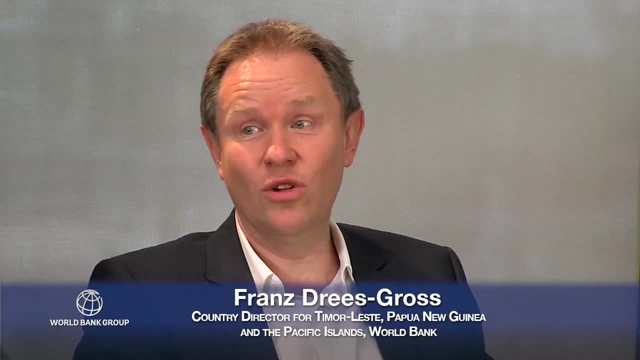 mean Ben just mentioned. it just came to mind that he was in primary school in 1975.. Well, if he was in primary school, he was one of only 50% of primary school age kids that were in primary school in 1975. 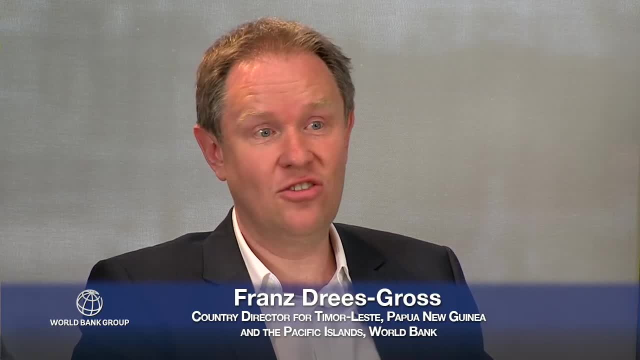 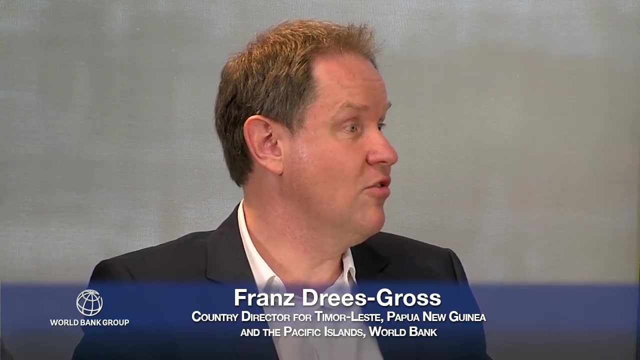 Today, 96% of primary school age kids are in school, So that's a huge achievement. The number of kids actually going to school, especially in primary school, has increased significantly and that's a relatively recent development. So, looking back, there are a number of substantial 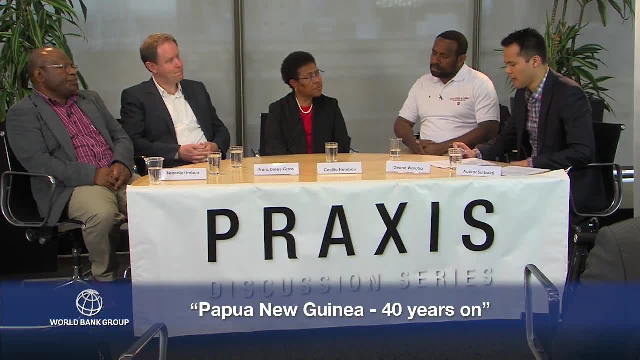 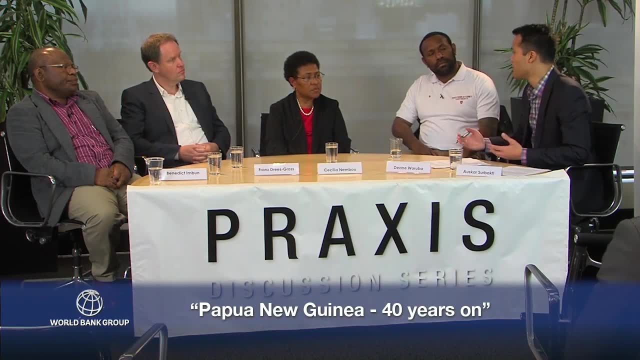 achievements over the last 40 years. Cecilia, if I could ask you, Franz just mentioned there, I guess, the development of the education sector in the country. That's a particular passion of yours. Why do you believe education is so important in your country? 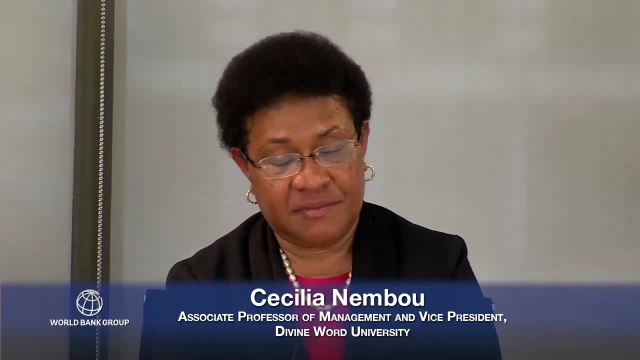 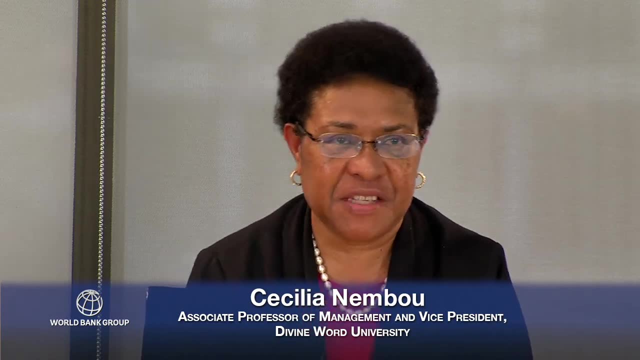 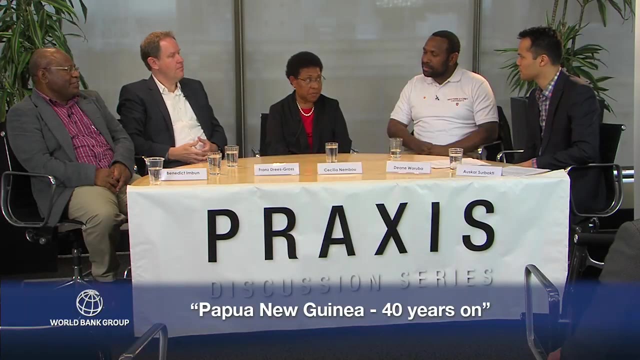 Let me begin by saying I actually graduated with my bachelor's degree six weeks before independence, So I've been working for 40 years, while PNG is 40 years. I believe very much that everything depends on education. Singapore has demonstrated this very well. 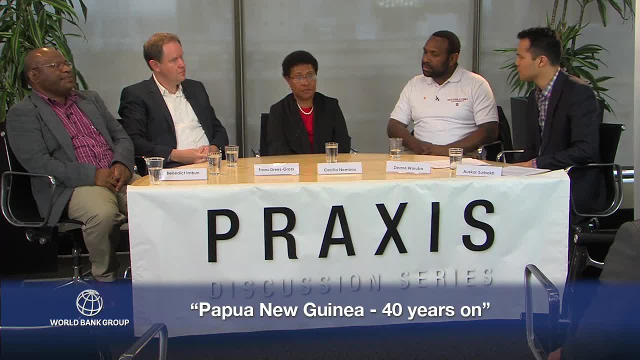 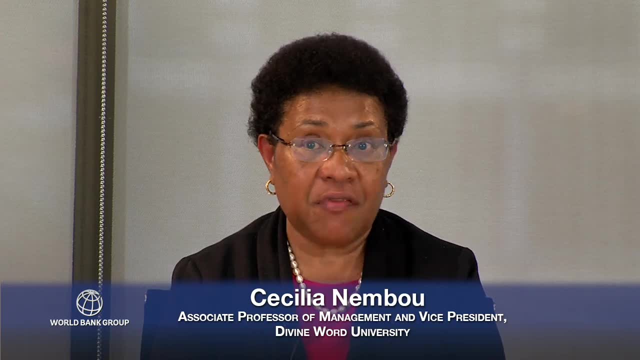 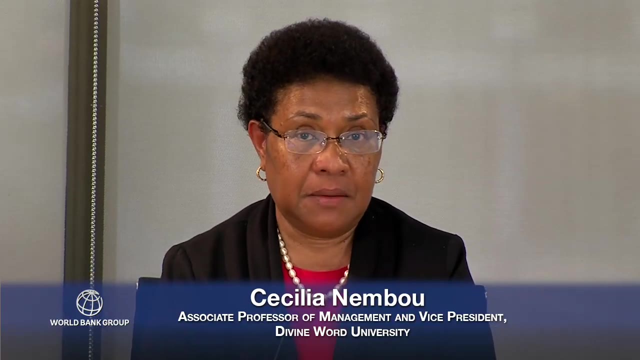 A number of other countries have got on board: Finland. I believe in Europe, Or is it Sweden, Switzerland? The development of the people is very much necessary. You cannot do anything else without educating your people And I believe the developments that, or if there. 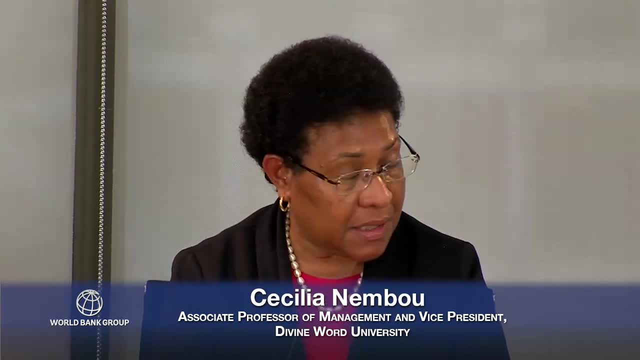 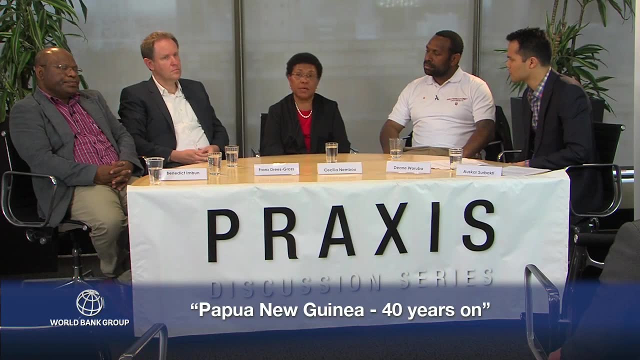 are any, and the drawbacks in our development at the moment have got to do with our level of education. We have come a long way. At independence we had two universities, Now we have six. We have an increasing number of tertiary institutions, So that sector is growing. but 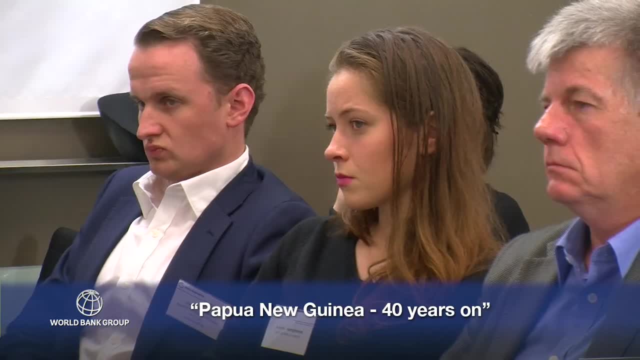 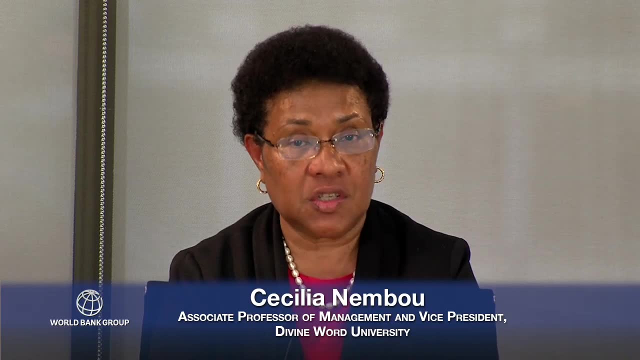 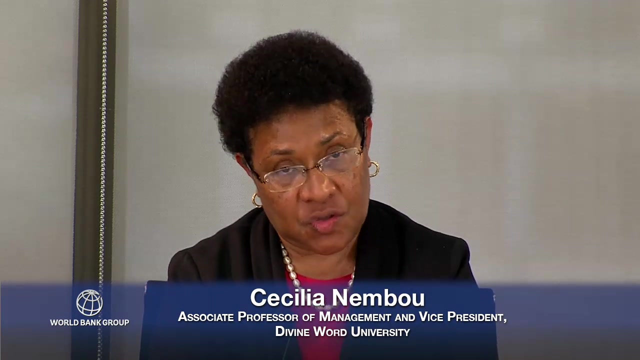 still, there is a lot of room for improvement. So, yes, the number of graduates coming out of university has grown since independence, But I would like to see more graduates coming out of university In order for us to with our 2050 vision with the seven pillars number. 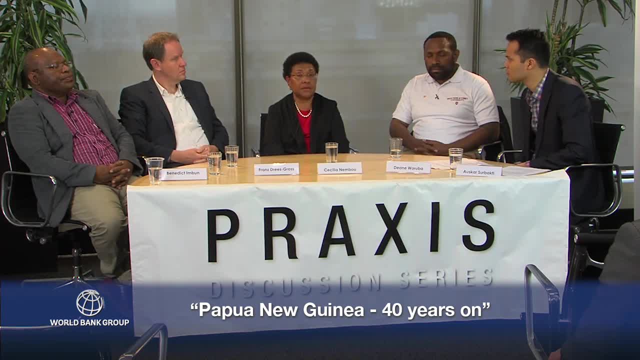 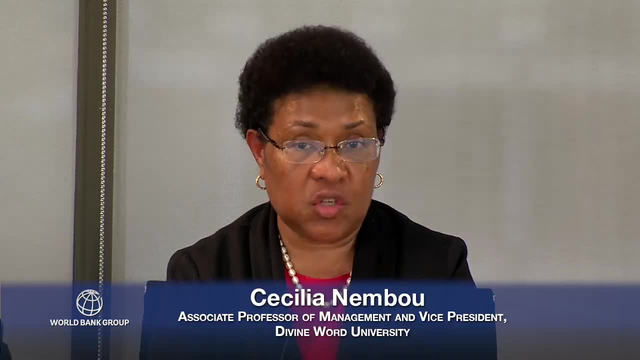 one. it's not by accident that number one is human development, youth and human capital, youth and people empowerment, because you need to educate the people in order that you can do anything else To defend our country. we need educated people. The army has got. 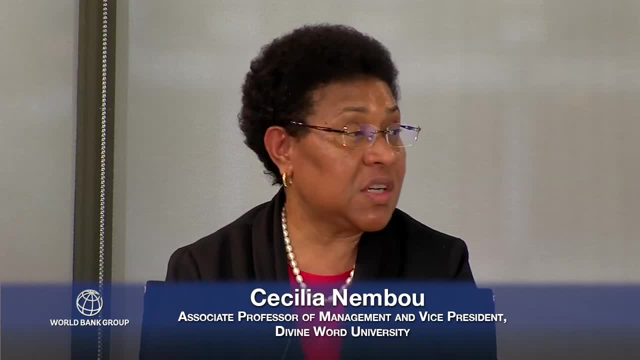 to be educated. The police have got to be educated. The reason our agriculture is behind is because the people do not know the science of cash cropping and things like that, And we'll ask Dean in a moment about the agriculture. We'll ask Dean in a moment about the agriculture sector, because that is a particular area. 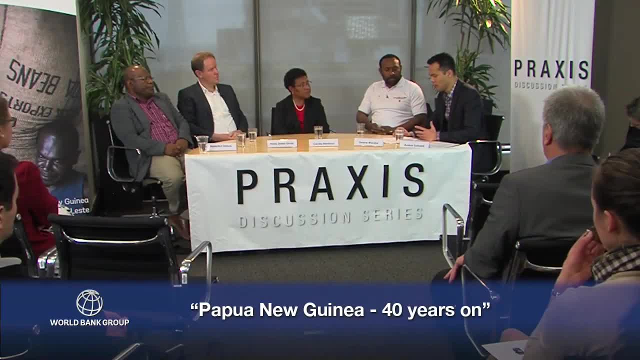 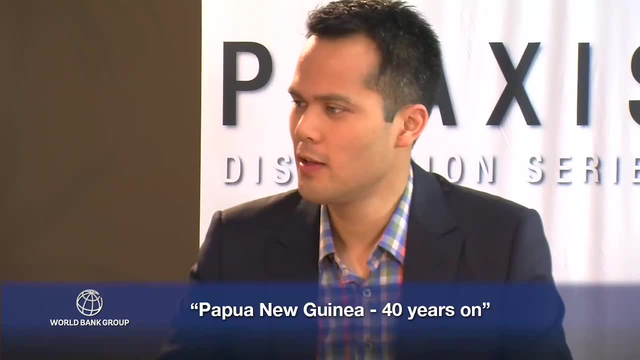 of interest to you. But in terms of the education system, am I right in saying that primary and secondary education at the moment is free for Papua New Guineans? But you're saying that there's a bottleneck After grade 12, there's a lack of options. Is that correct? 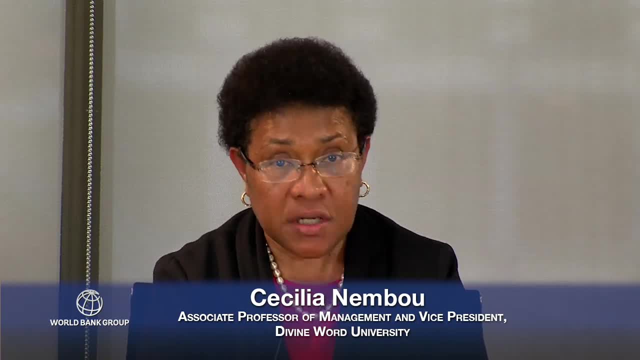 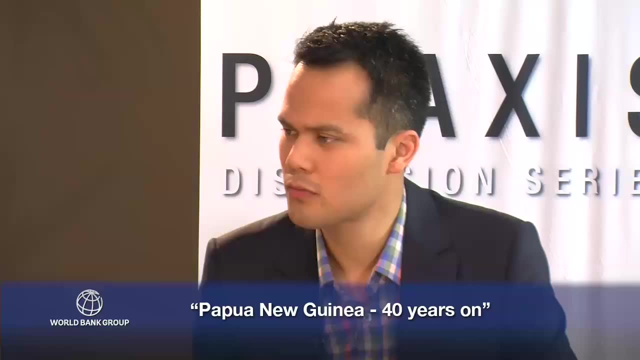 Yes, but the development has been such that in the colonial days education was free And there was at that level. there was a universal primary education, Then there was education, Then fees were introduced, And when fees were introduced, parents, the village. 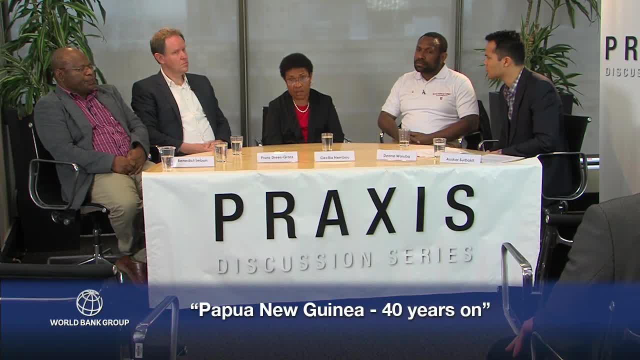 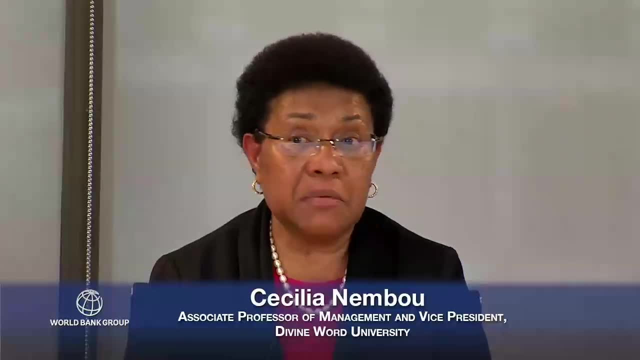 people couldn't afford. as you know, 85 percent of our people are in rural areas. They couldn't afford school fees, So the education level slowed down. Government has just recently realized that, And in the last year or so they brought in the new policy on fee-free. 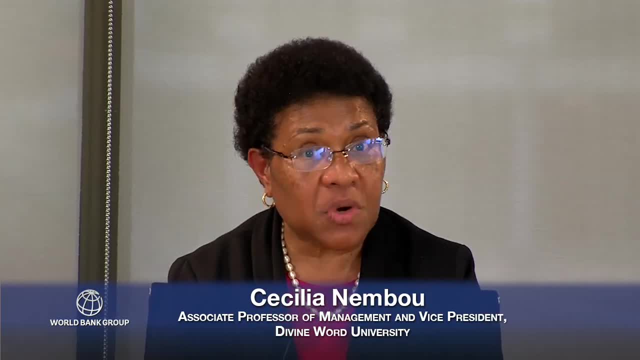 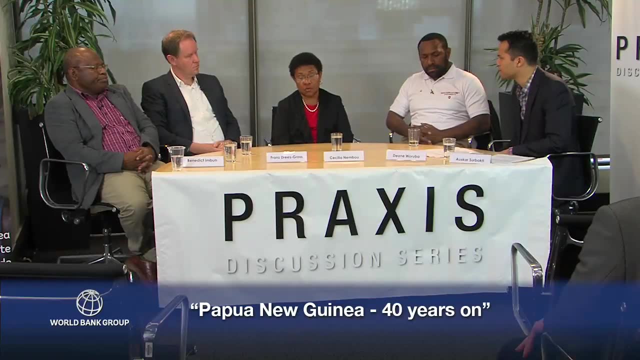 education. They have yet to come to terms with what all that means. For example: yes, there are hundreds and thousands of children now who want to go to school. Parents are saying: parents want them to go to school, But there's not enough classroom space There. 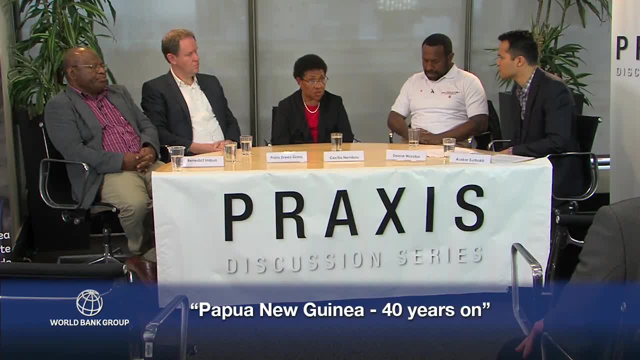 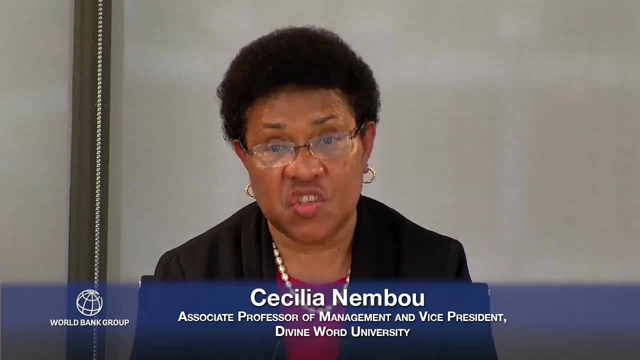 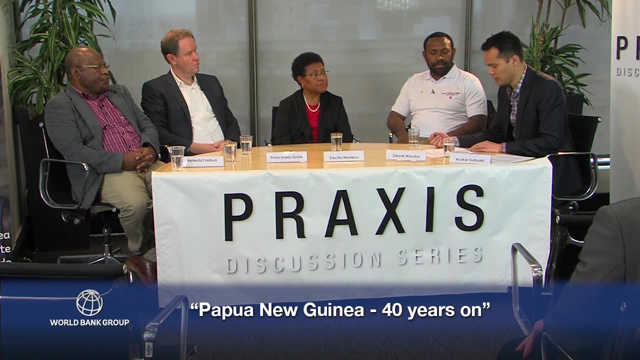 are not enough teachers to go around. Yeah, So there are some issues with seeing the implications of policymaking before those policy decisions are taken. But, yeah, we're getting there And I think, to quote what you quoted previously- so the country is at the moment seeing 20,000. 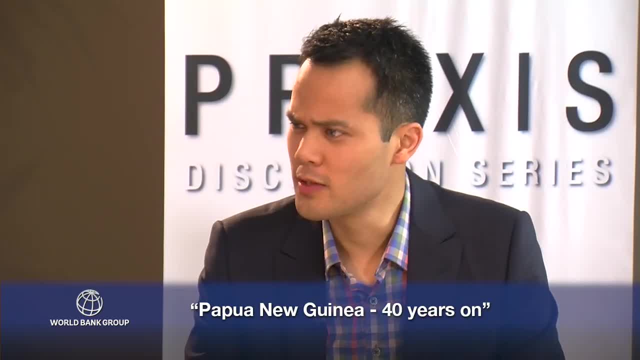 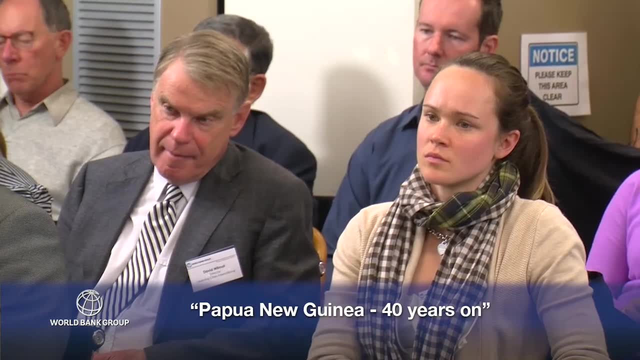 graduates from grade 12, but there are only 5,000 tertiary spots of our students And that's not available for them. So clearly, the tertiary sector is an area that needs to be developed. But, Ben, can I ask you? you're an expert in the employment sector in Papua. 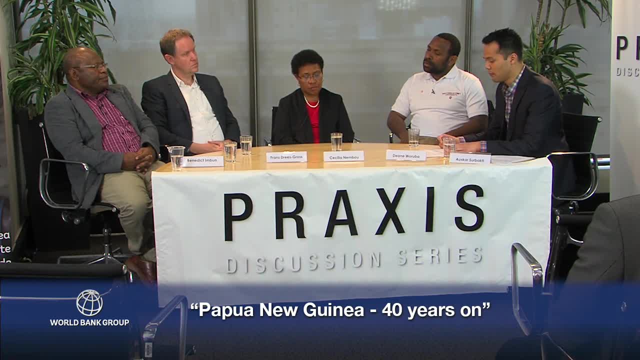 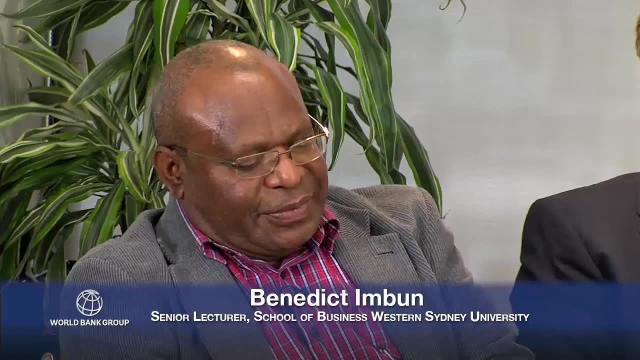 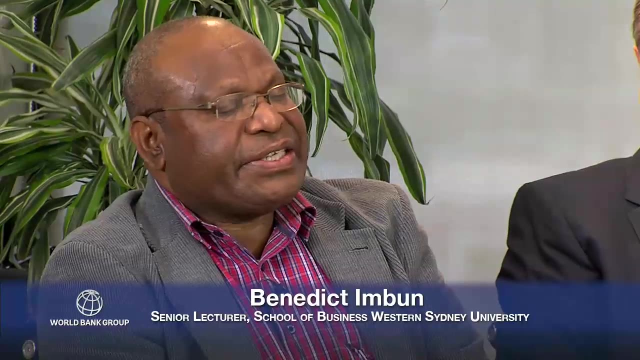 New Guinea. Even if the country manages to provide these 20,000 graduates with the equivalent number of tertiary spots, will there be jobs for them at the end of it? Yeah, there would be a challenge. I mean actually, given that the extractive sector 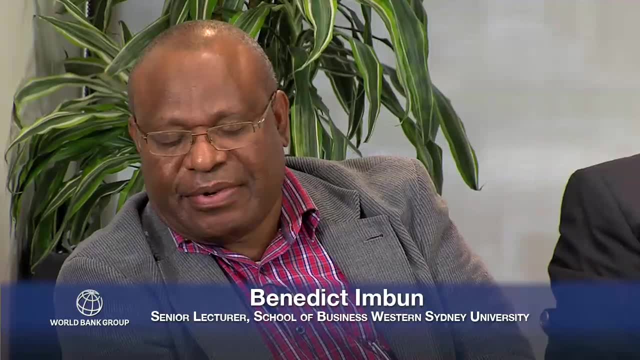 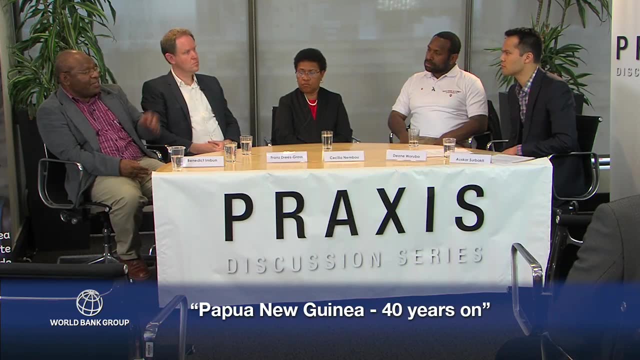 is actually the most dominating sector next to agriculture, but the extractive sector is more capital-intensive- fly-in, fly-out, consultants, miners based in Cairns, So there is little trickle-down effect that would trigger the economy to sustain or provide more employment. 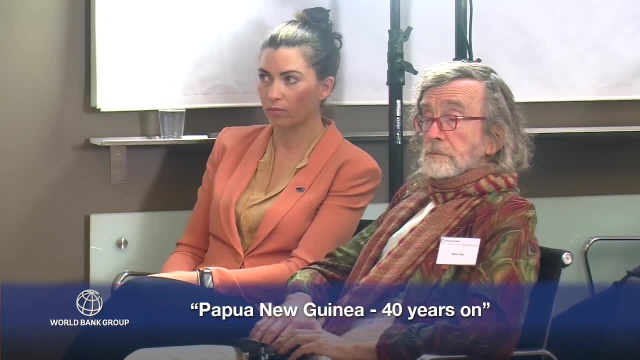 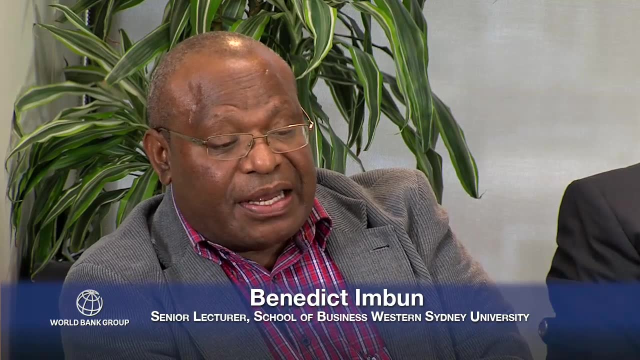 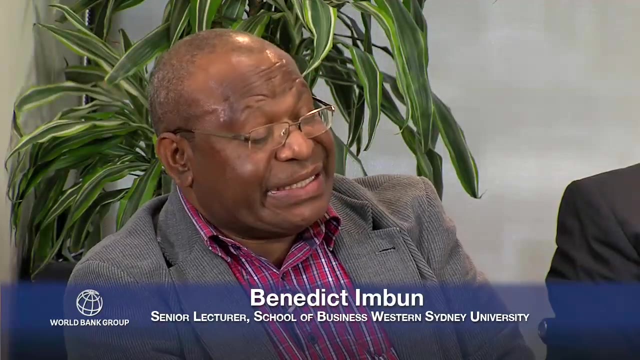 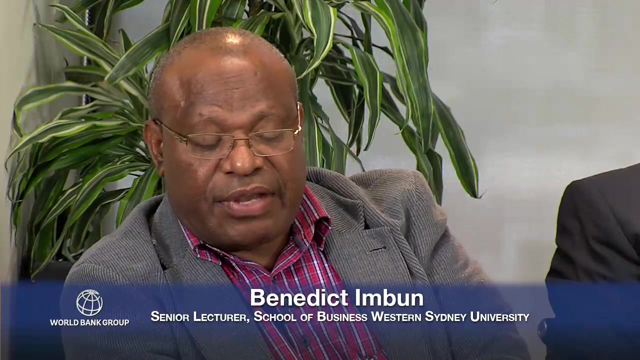 opportunities. So, although the government has gone hugely in favor of the human capital or human resource development, Alternatively, on the other side, they haven't actually done much more on the labor market side in terms of, you know, youth empowerment or labor market initiatives or to have jobs. 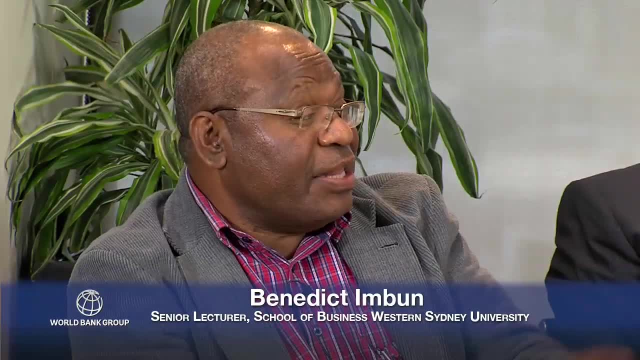 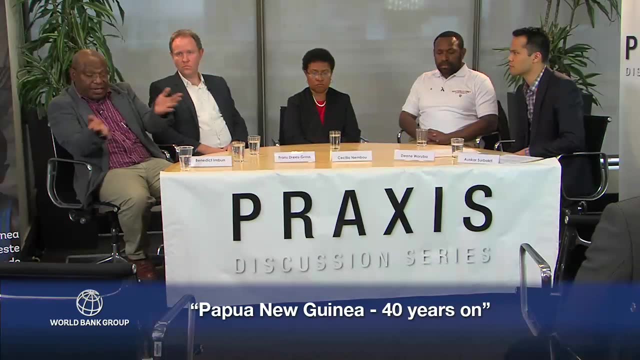 particularly in the agriculture sector. So that's where the mismatch is, That's where the challenges are. Probably down the line, after having a cohort of a core group of all these educated people around putting pressure on the government and the government, then obviously gradually they would come to realize that they need to create jobs. 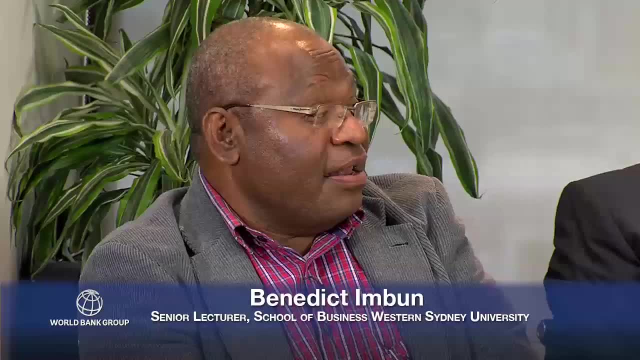 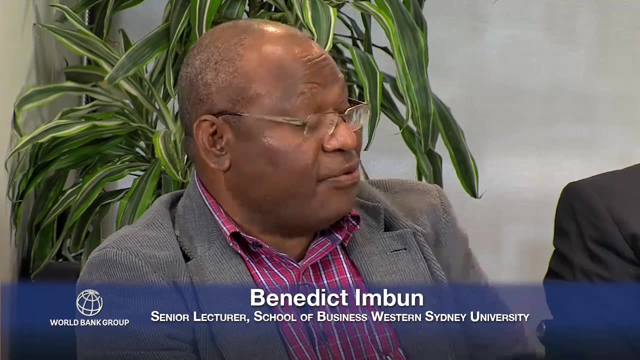 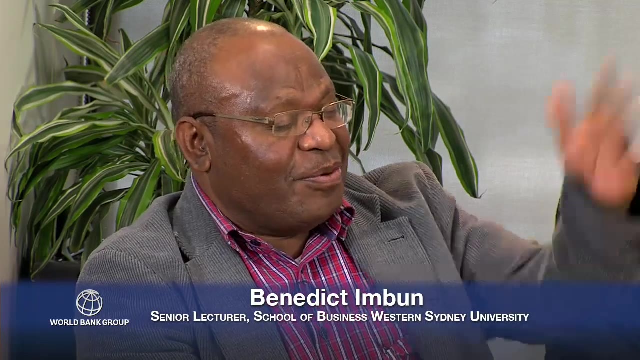 That's where the missing link is, And obviously I mean a lot of Papua New Guineans have migrated as well, particularly with the extractive sector. A lot of them work here, but that's in relation to the demand for skills and other things, But 80% of everybody, or 100% everybody. 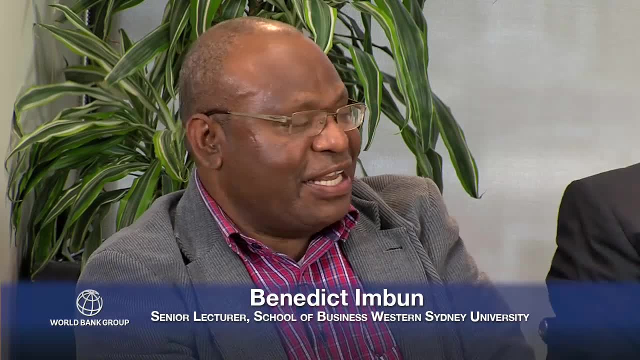 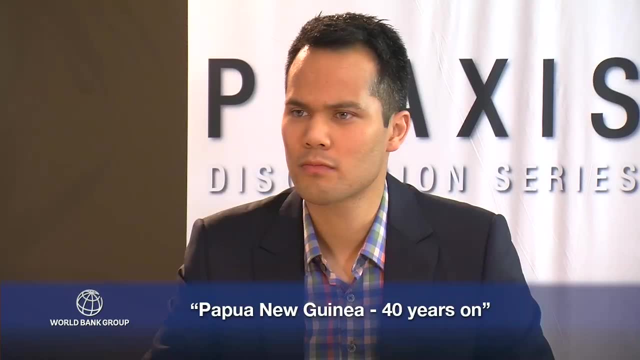 is contained in the economy, but the courtesy of the Southeastern sector, because there's probably a thousand jobs are created. A thousand jobs are created annually by the PNG labor market. So if 20,000 people are not absorbed in the formal system in terms of federing their education, obviously the 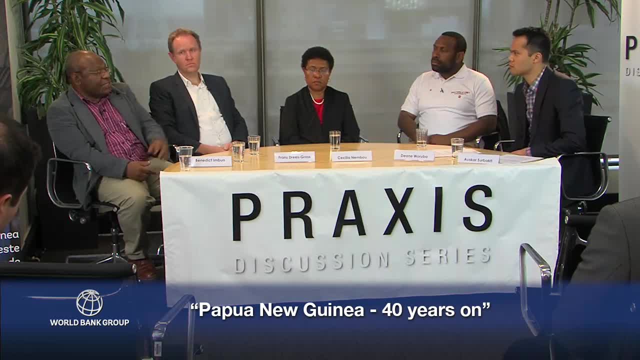 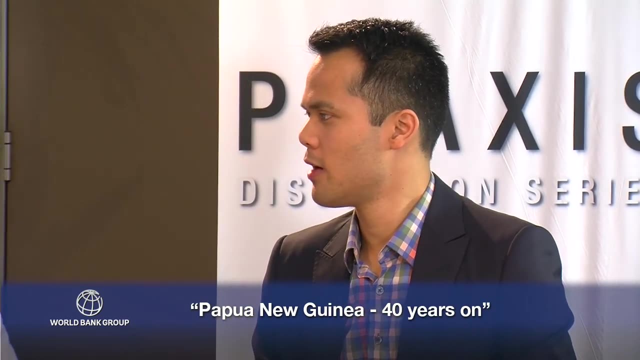 one talks or the relatives, or the subsistence sector is absorbing them. So that's a huge challenge for the government, Interesting Of the day on the subsequent government. Okay, So job creation is another challenge. That's right Dean. now, as I mentioned, agriculture is a particular area of expertise for the 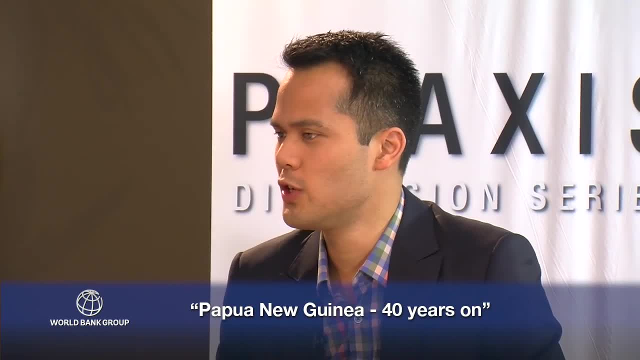 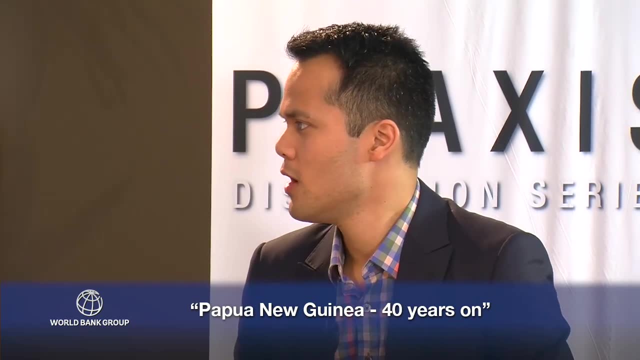 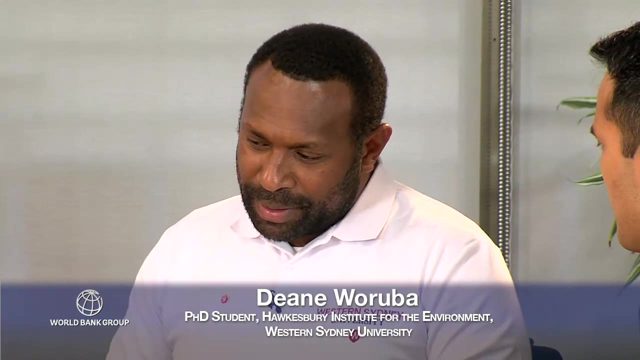 PNG. Yes, And you mentioned- Cecilia mentioned- that one of the challenges is to educate the people who are currently in agriculture about, I guess, better ways to better techniques for their industries. Is that a problem in your view? Firstly, well, agriculture in Papua New Guinea evolved independently from the rest of the 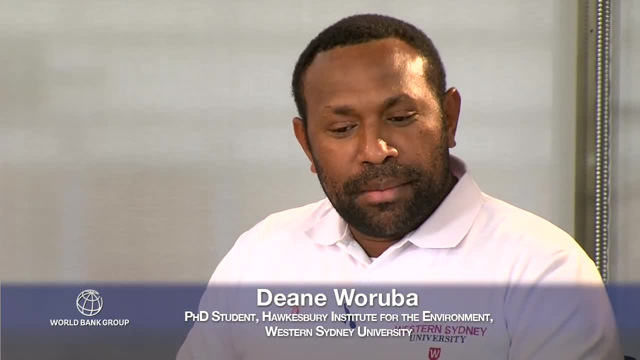 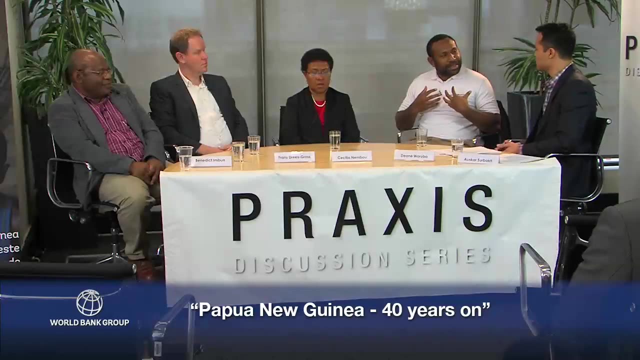 world some 10,000 years ago. With that, we've had our own practices of how we farm And in my opinion that now needs to change if we are to move forward. Agriculture that we need is, say, cash crops, monoculture, where you're cropping cocoa, or if it's. 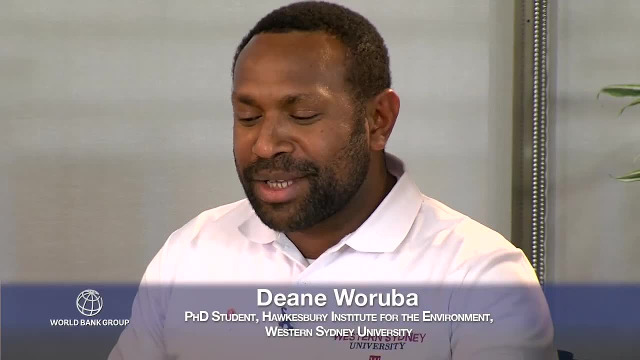 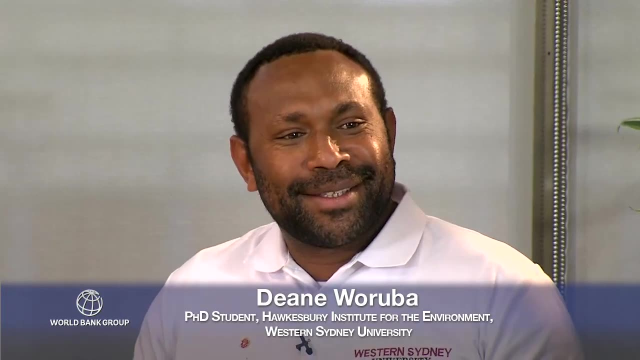 intercropping, it's just two crops, But not like before, where there's a bit of taro, banana, cassava and we're only planting perishables, things that we can't store. So that's when we have a situation like we're going through now with the El Niño. 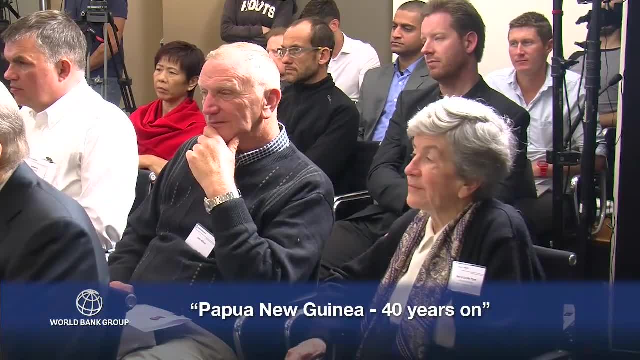 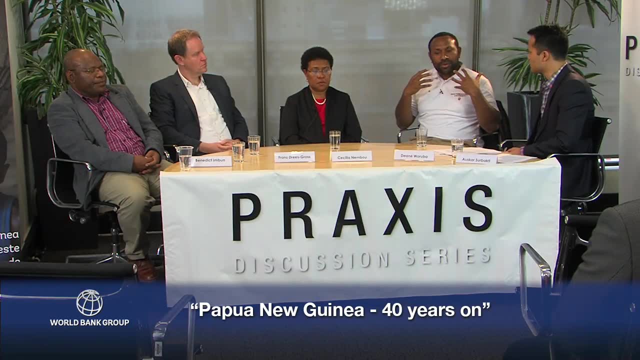 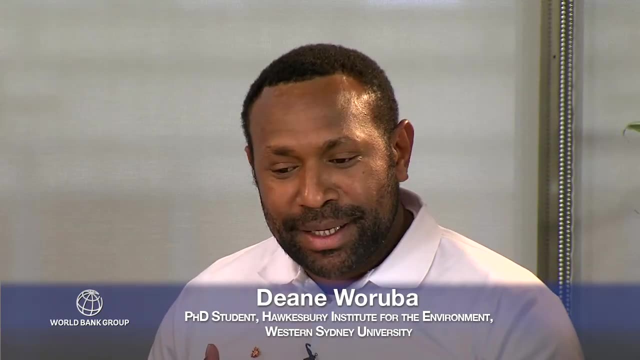 We can't store because we're not producing crops that we can store in late. we can't produce crops that we can store and sustain us now. To get our people to appreciate cash cropping, they have to understand what it is for. At the moment, in my opinion, we're. 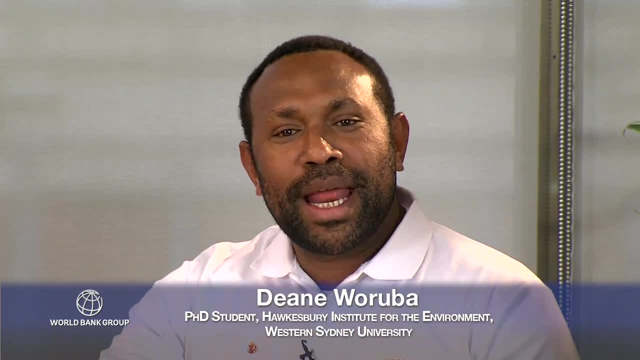 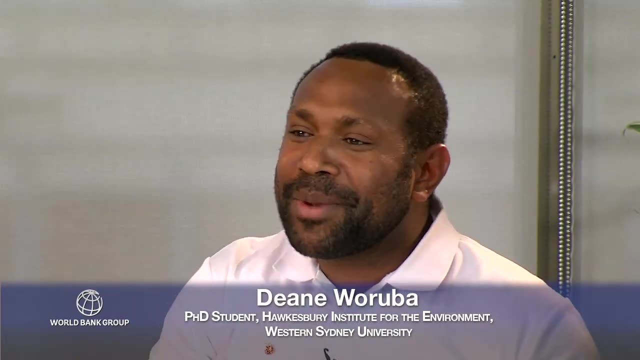 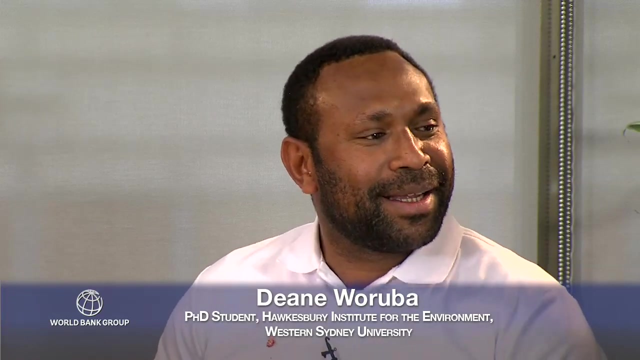 seeing these cash crops as a means to an end. I'm planting cocoa because I need to build this house. The moment I put the tin roofing up, I go back to doing my own thing. until I need to buy a generator, I go back to my cocoa garden, clear it up and then go again. 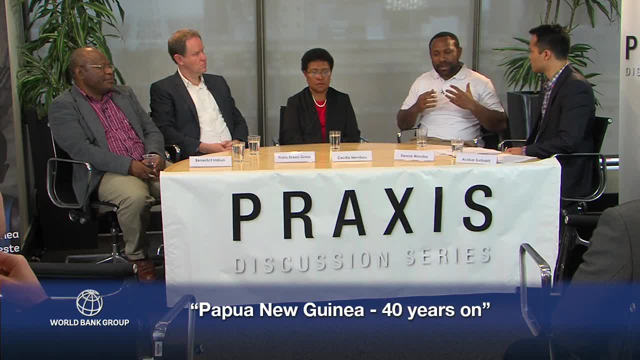 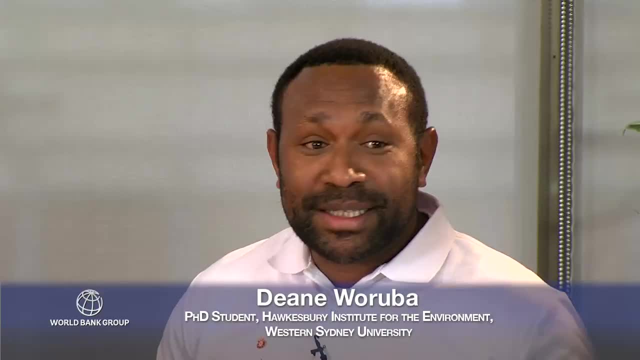 This is the mentality that we need to change if we are to move forward, if we are to keep a constant supply of our produce to maintain the economy, to drive and stimulate our economy. But agriculture still has a big, big, important role to play: More than 85% of our population. 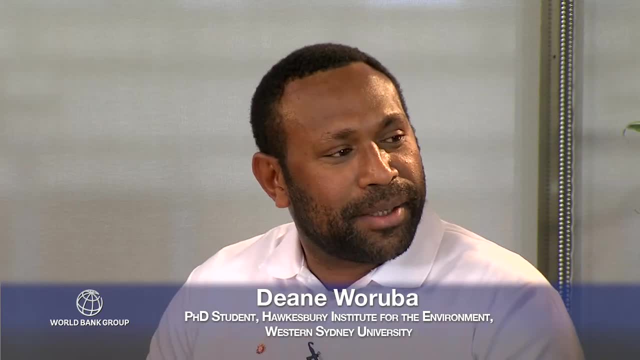 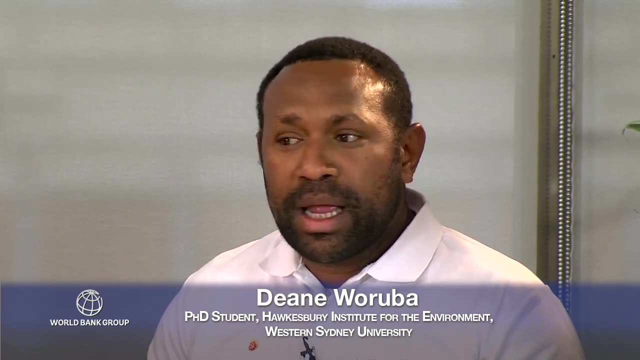 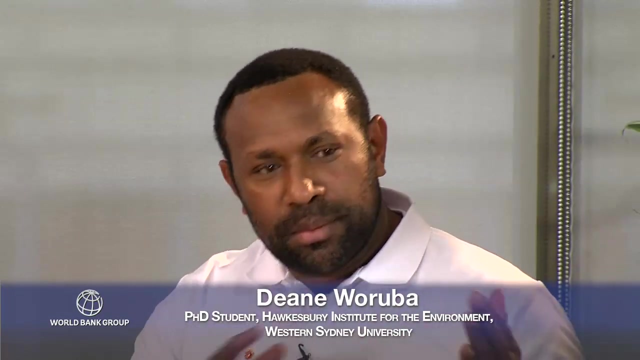 in the rural communities. they rely on nothing but agriculture. It is a very fundamental key in our development, moving forward In our vision 2050, in the pillars that we have. I think agriculture is a cross-cutting thematic theme that you could probably answer three of those pillars for development and 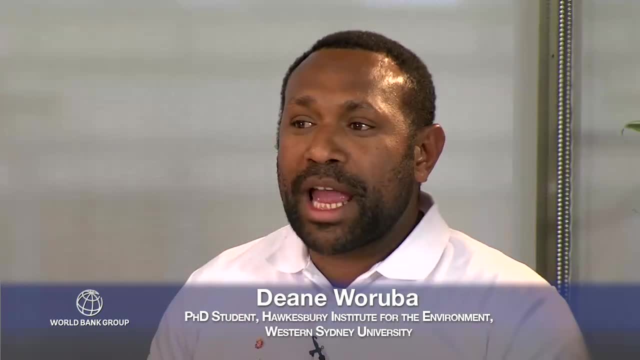 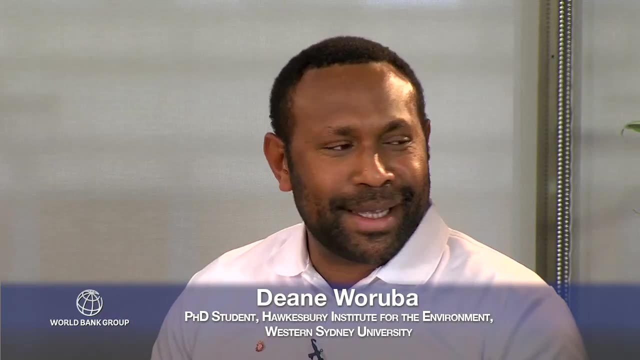 moving forward. If we achieve our vision, agriculture will play a very vital role and agriculture and natural resource development a very vital role in where we will be 50 years from now. I'm excited about it because I hope to be part of it. 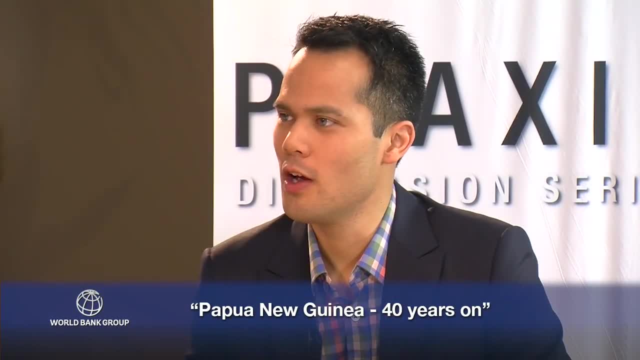 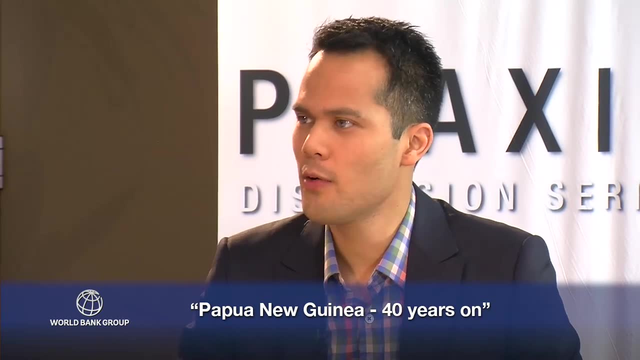 Excellent, Frans. you were recently in Papua New Guinea. What were some of the things that you saw? What were your observations? You listed some of the impressive achievements that's happened over the last 40 years, but are there areas of improvement that you saw? 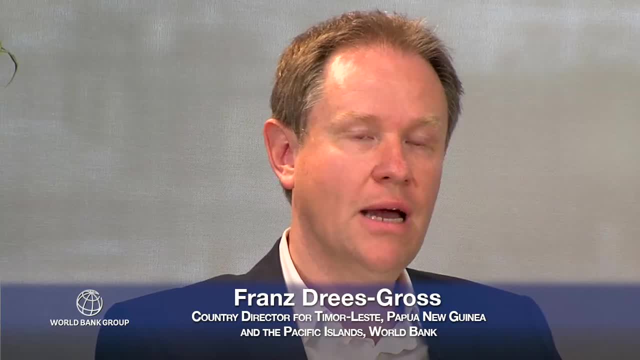 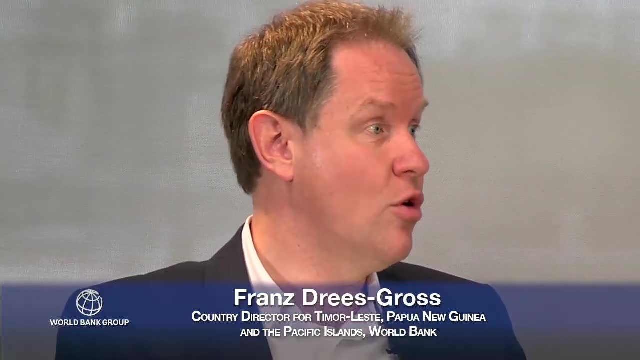 Right, Let's just pick up on what Dean said about agriculture. Essentially, you've got a country that's still 85% rural, where about three to four million people derive at least some income from cocoa and coffee. I began by saying: today there's 60% more coffee production. 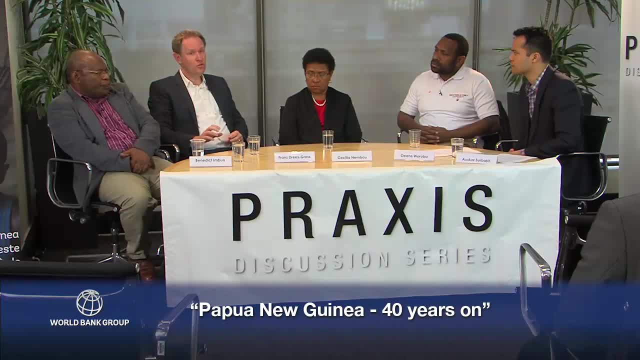 than there was at Independence: 25% more cocoa. But if you scratch that surface a little bit, it's not a pretty picture. I mean what you see, and I was just up in Mount Hagen, for example, two weeks ago- right, 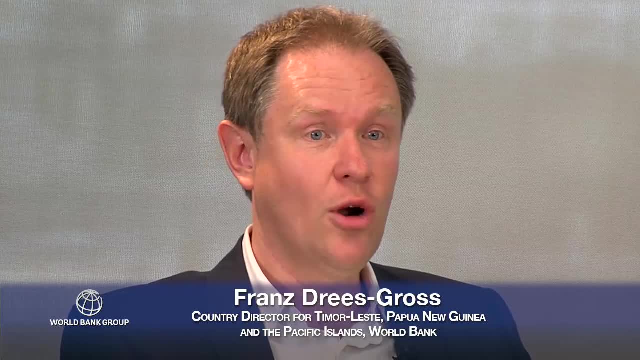 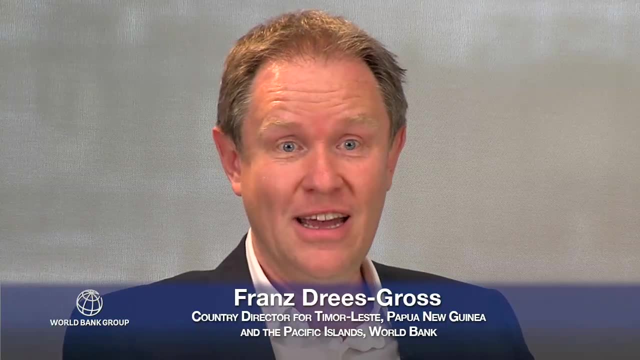 before the Independence celebrations, you visit family farms that are growing coffee, for example, and you see trees that are 20,, 30, sometimes 40 years old- as old as the whole country- and they're pretty scrawny. You've got maybe 10, 15 cherries on a tree. 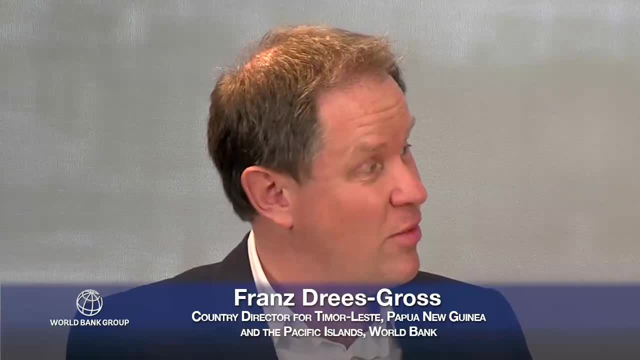 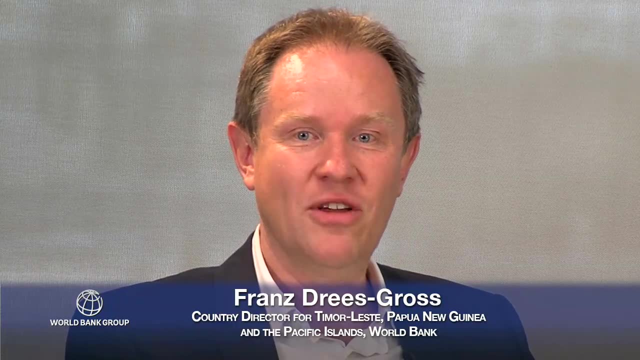 that should be carrying hundreds. So what you have is a lot of people that are maintaining sort of a toe in the coffee production sector, but they're not running their farm as if it were a real sector. They're running it as if it were a real source of continuous income and livelihood, And you 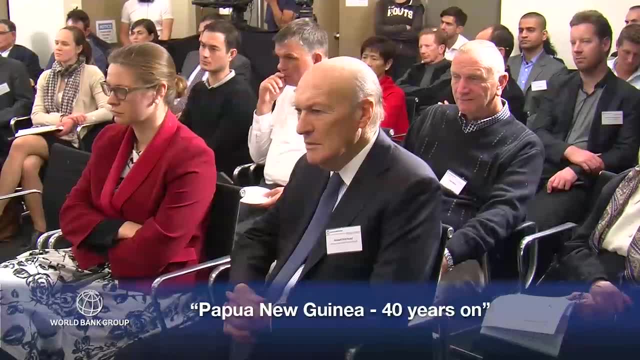 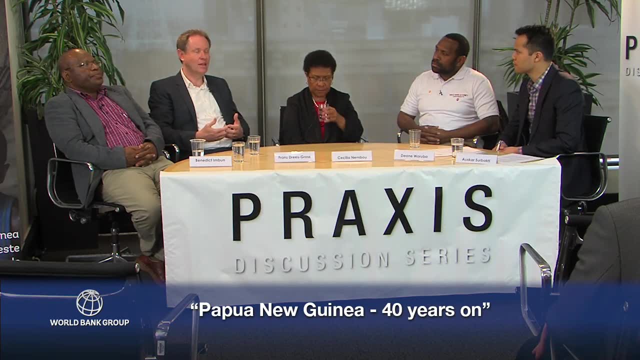 could produce a multiple- I mean many times- a family farmer on the same amount of land. by replanting, rejuvenating the coffee trees, for example, You could be producing much, much more. And it is a matter of education. It's a matter also of, of course, having the 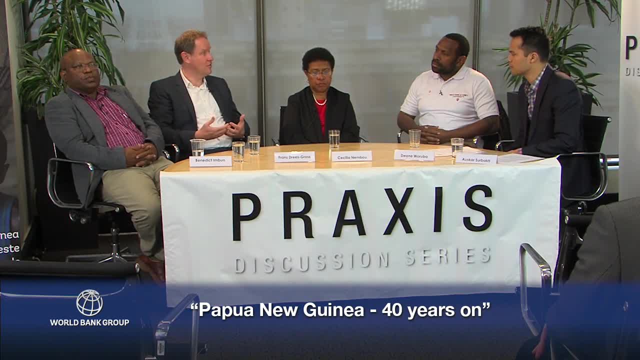 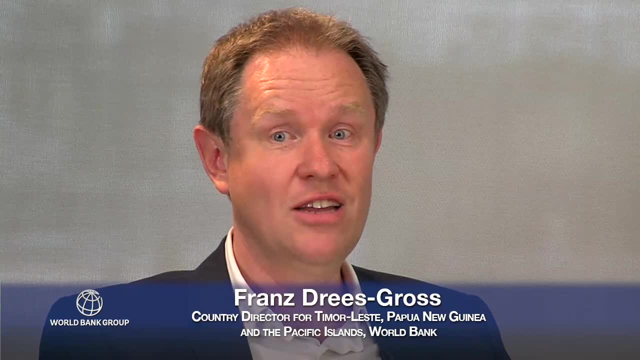 supporting infrastructure, the access, roads, the electricity, the processing facilities, et cetera. But if you're going to, we talked, Ben did- about where the jobs are going to be coming from. Part of it is being more productive in agriculture and then building on that to process the yields. 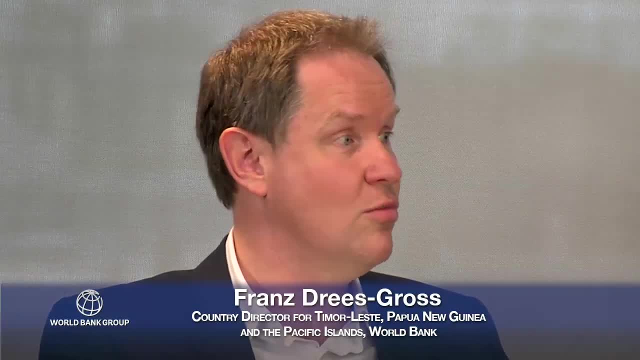 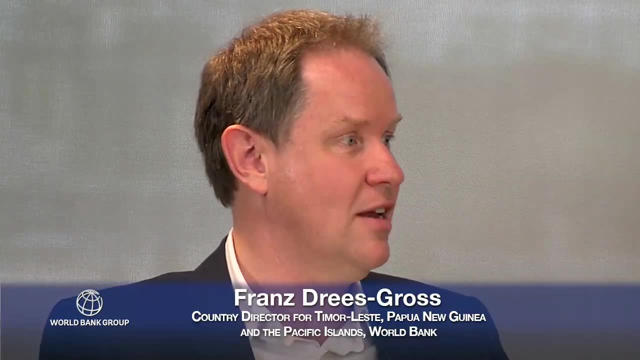 of agriculture. That's where the jobs are. They're there, they're in tourism, they're in services, but they're not so much in mining, where you're going to have a few very well-paid jobs, but mining doesn't tend to generate enough jobs for a country like like PNG. 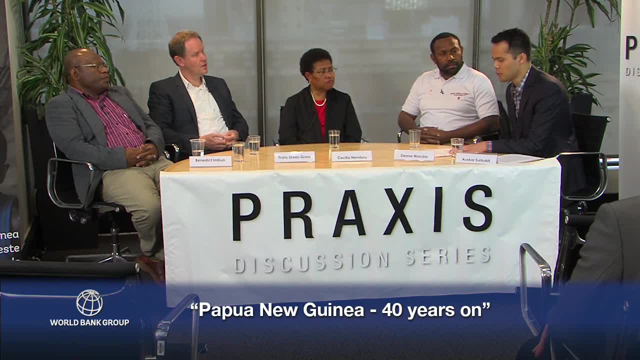 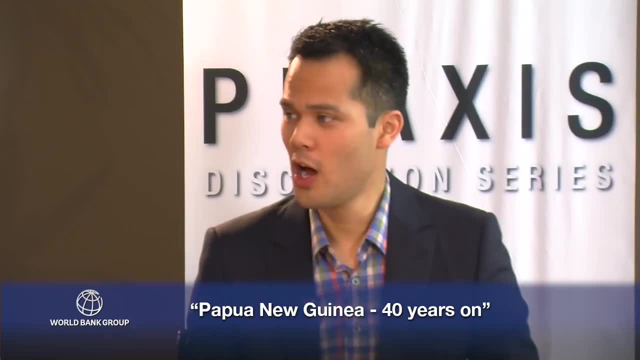 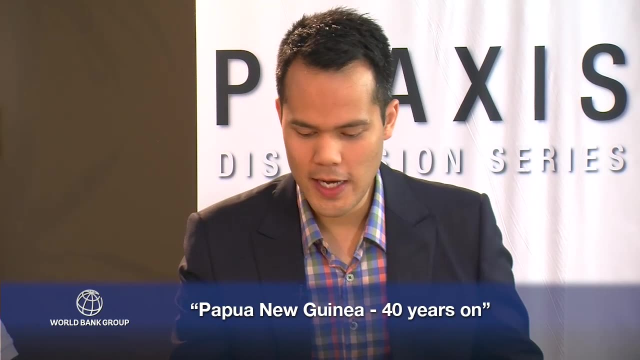 Okay, Before we go to questions, let's briefly talk about the Vision 2050 document. So this was a document that was developed by the Samara government in 2009.. Yeah, And to quote Mr Samara at the time, he said: we leaders and people must know where we want. 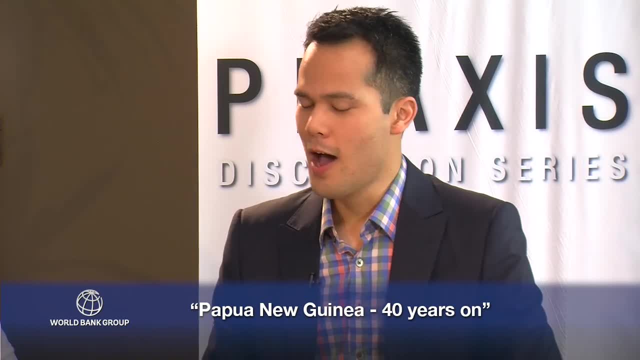 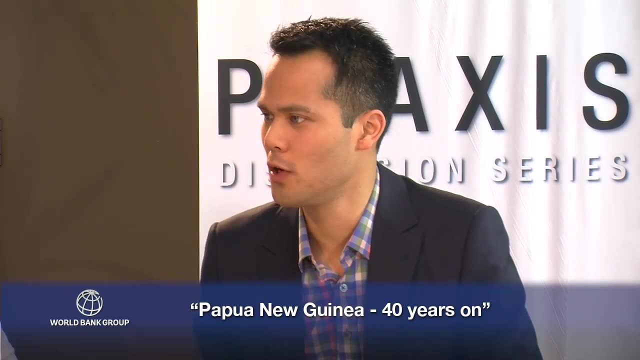 to go before we can decide how we should get there. What, Cecilia, can I start with you? What do you think about the Vision 2050 document? I mean, summarise it for us first and then give us your view. 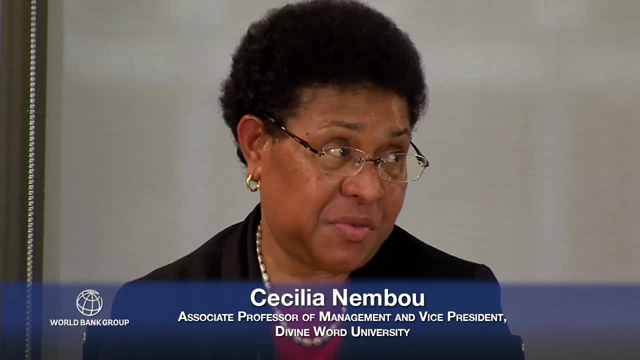 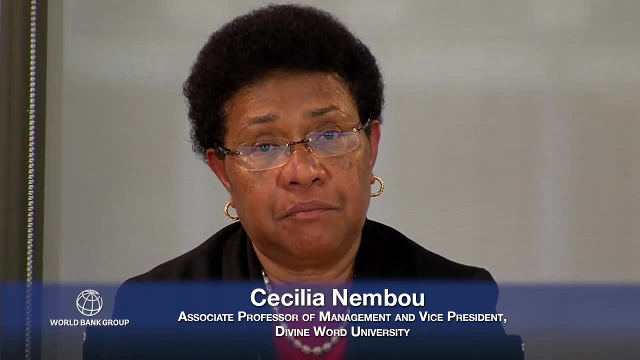 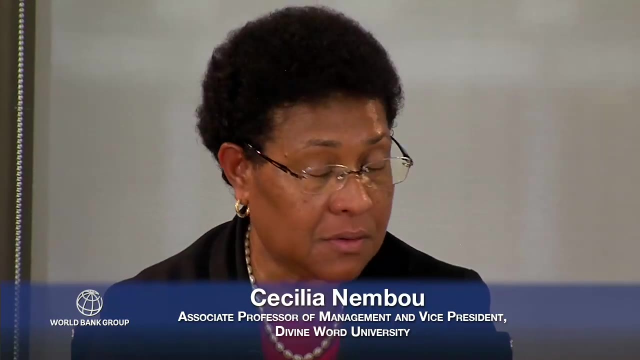 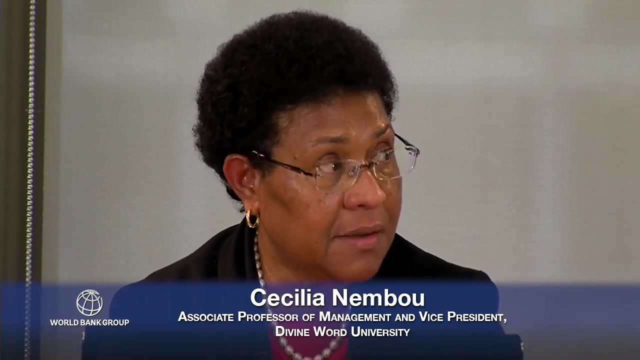 Vision 2050 is actually a strategic plan, a 40-year strategic plan for Papua New Guinea. The vision is that between 2010 and 2050, we would develop, we would address the seven pillars such that by the year 2050, we will be a smart, wise, fair and happy society. 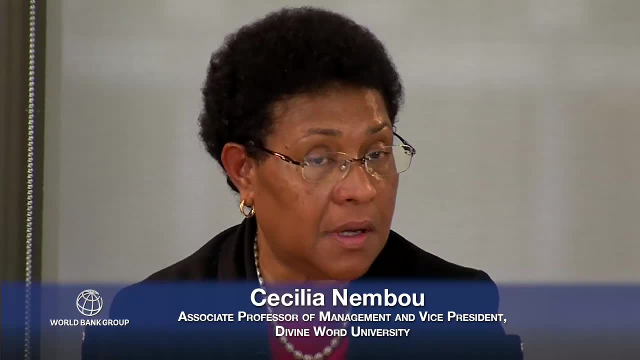 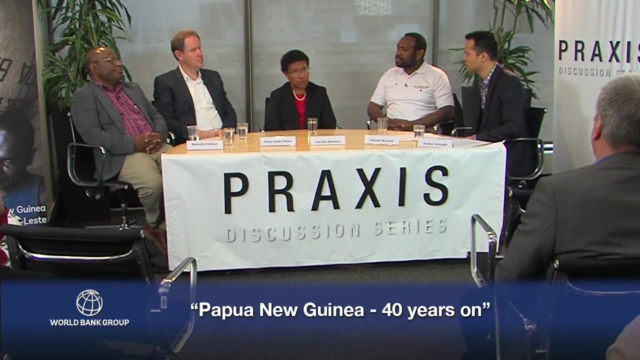 Now, that's a mouthful, but we need to make it work. The task force that put that together on behalf of the government put it in place, Okay, And put it in the form of the seven pillars Now. the seven pillars I see as seven strategic. 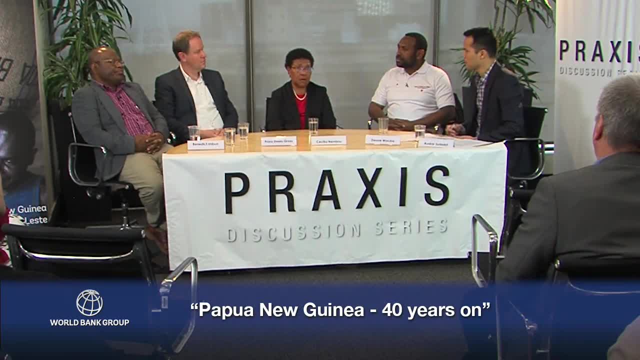 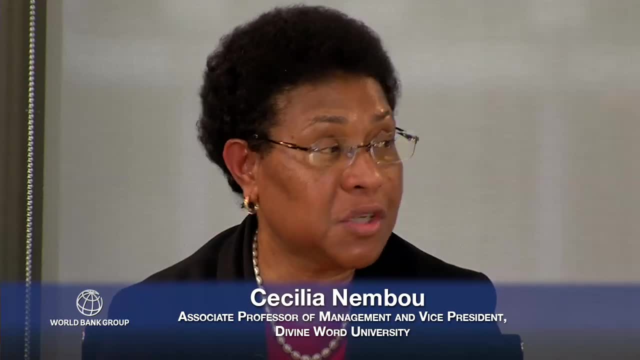 objectives. The first one is human capital: youth and people empowerment, human capital development. The last one is to do with strategic planning, to actually continue to get involved in strategic planning and implementation monitoring. And then in between, there's defence and there's 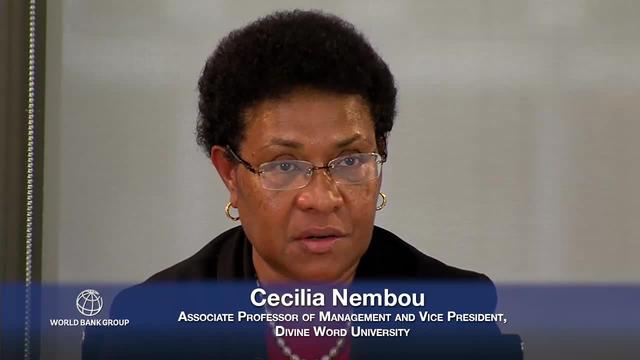 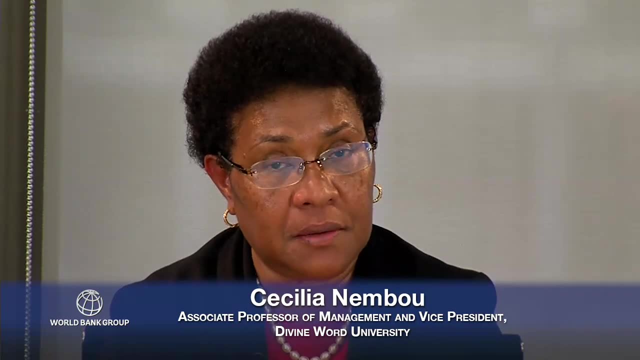 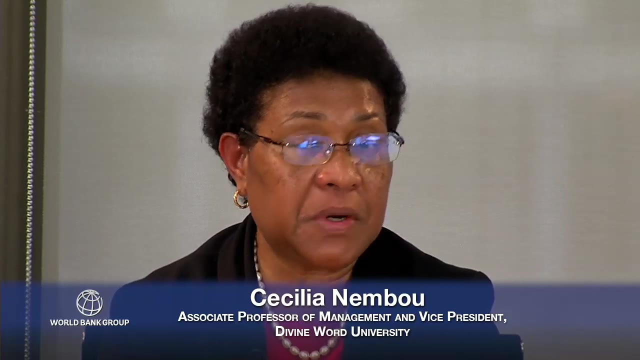 environment and the others. I cannot list them all off by heart, But I think it's a very good plan. It's a very good plan because it actually is derived from our five national goals, directive principles which were put together at the time when we were preparing for independence. 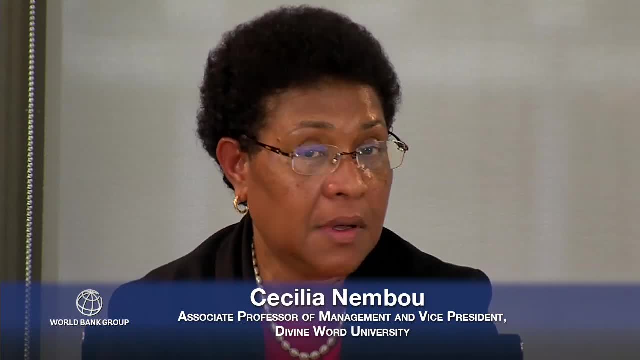 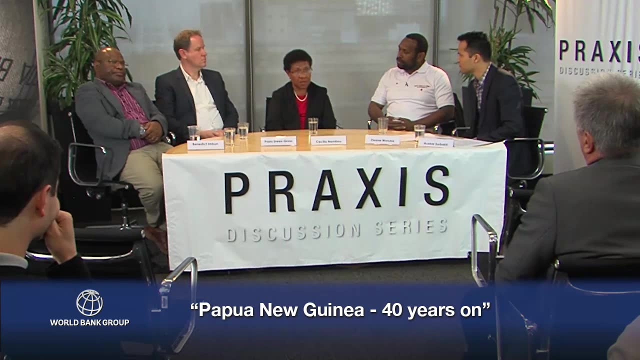 and we put together our constitution, And I think it's a very good document. What makes me happy about it is the fact that both sides of the house have accepted it. The bureaucrats and the whole society, at least, and those of us in the education system, have taken 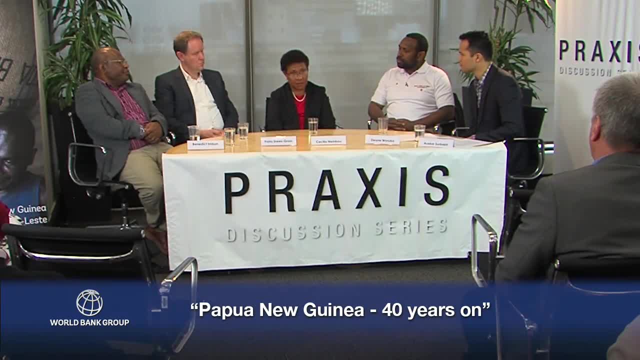 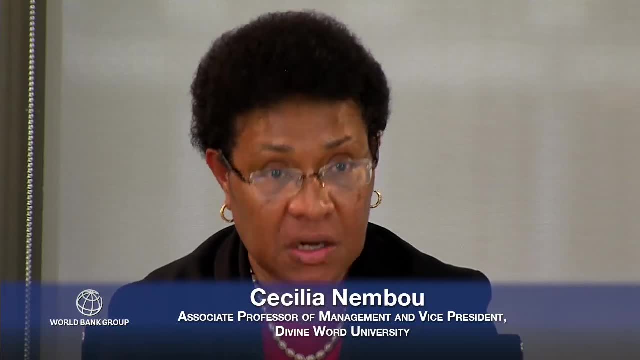 very seriously the first pillar because, as I mentioned earlier, we cannot do the other seven without addressing the first one, which is to educate our people. And I believe that if we educate our people at every level of education, from the technical to tertiary, 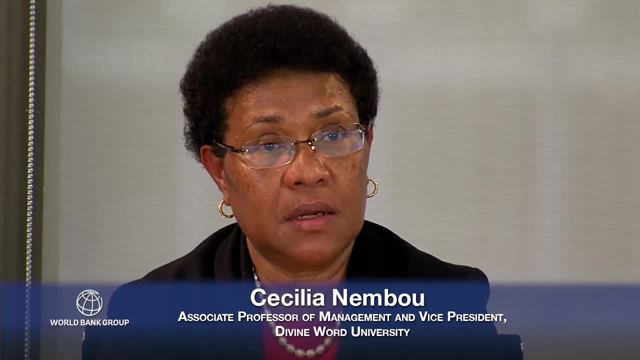 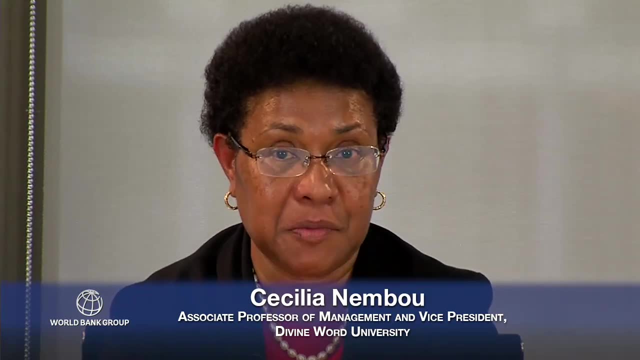 level to schools, starting in the schools, then we're not going to realise our plan by 2050.. But I always say to the young people, when I'm speaking to them, that this vision is for the young people. I say it's for you and your children and your grandchildren, because I've 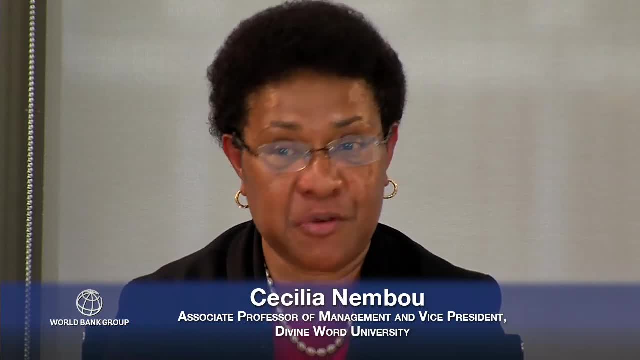 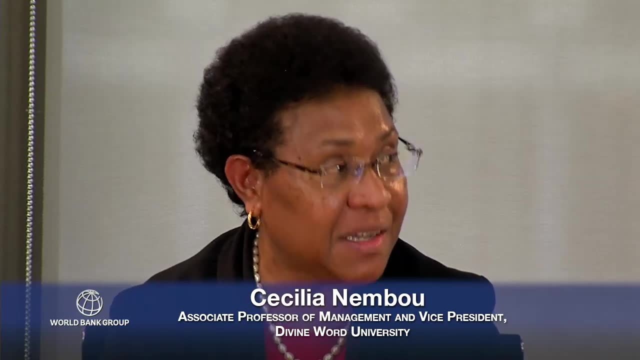 lived mine In Papua New Guinea context. I have worked for 40 years. I'm ready to retire, But I encourage them to take ownership of this plan, this strategic plan, and make it work. But at the moment, before I retire, I'm helping to educate the younger ones who 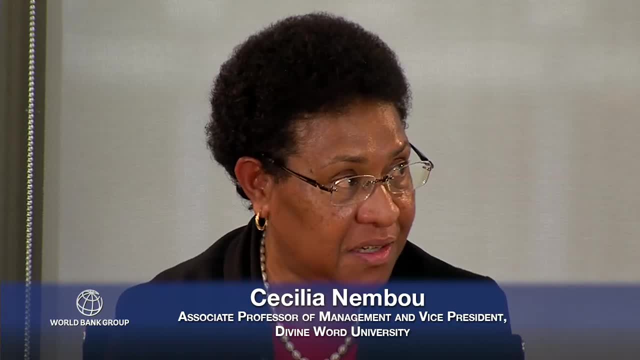 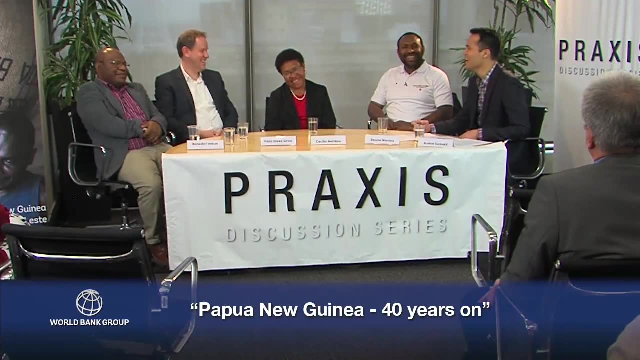 will actually benefit from a clear direction of where we are, What we are going and what we need to do to get there, And let's hope you'll be around for many more years. Cecilia, Ben, do you agree with Cecilia? 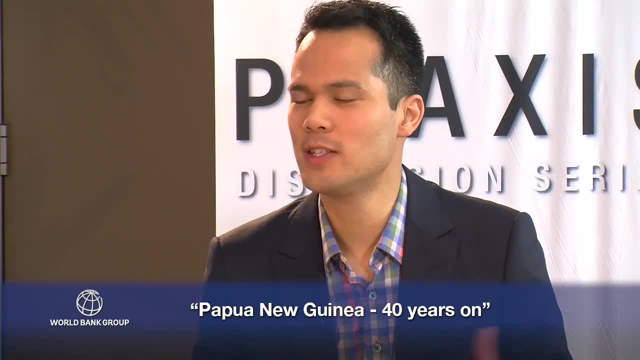 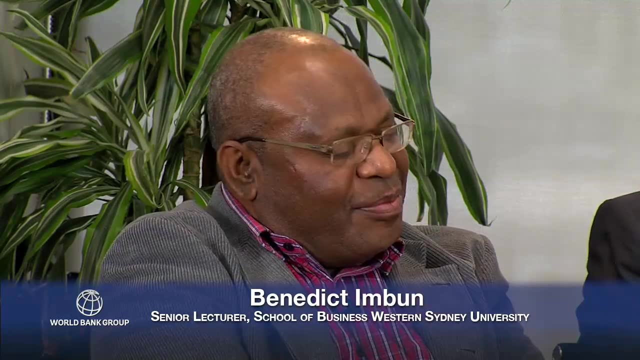 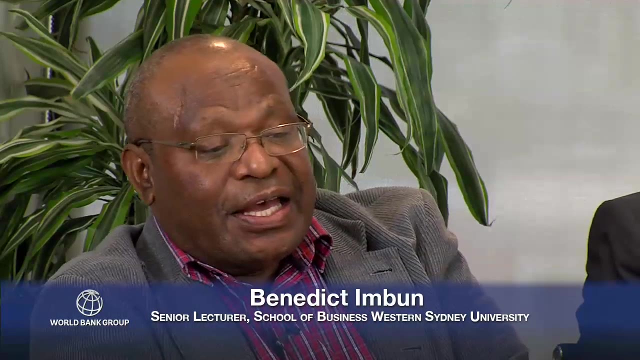 It sounds like it's a very positive document that has widespread support politically. Do you think it is achievable? Well, it'sachievable would beI tend to say more idealistic, more on an abstract level, But how we are going with the development of human resources. obviously we are making 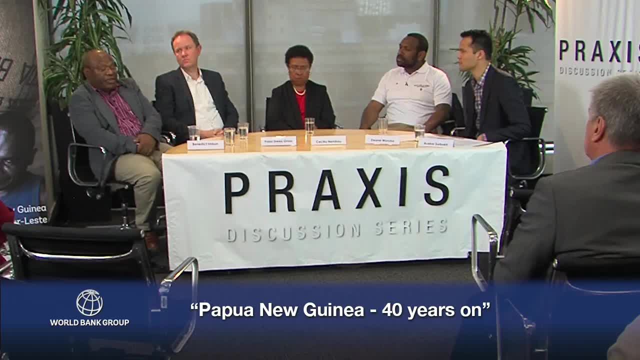 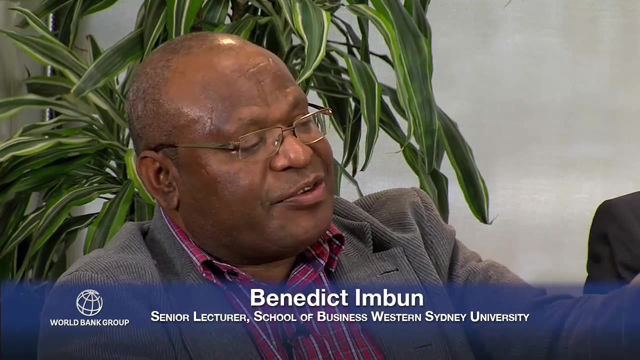 huge steps towards, you know, Empowering people with education skills, But it has to be pragmatic. applied. I mean, 85% of the people obviously live in villages isolated from whatever happens in Waigani. So in terms of transmitting, in terms of, you know, making it more practical, like the 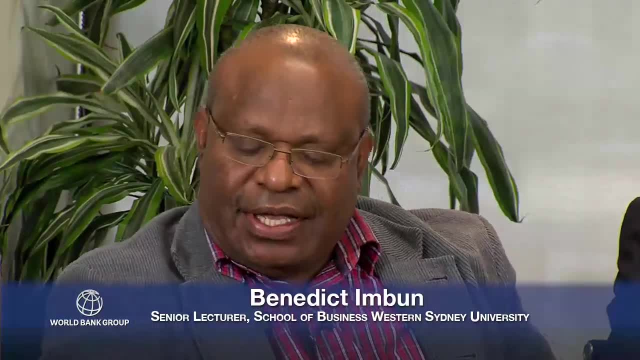 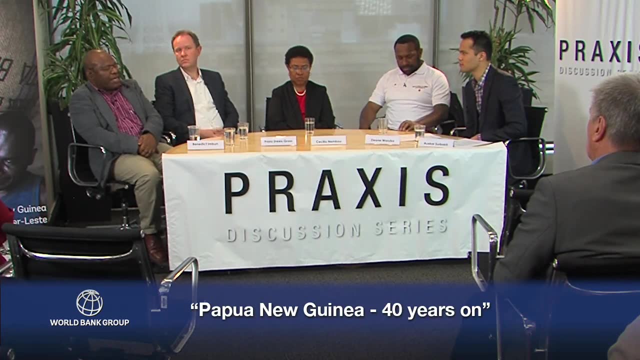 agriculture you have, Frank mentioned, people could even develop more on the agriculture, I mean the piece of land that they have, so that they can have constant supply of money. But you know, agriculture is obviously one of the pillars there. But in terms of transmitting, 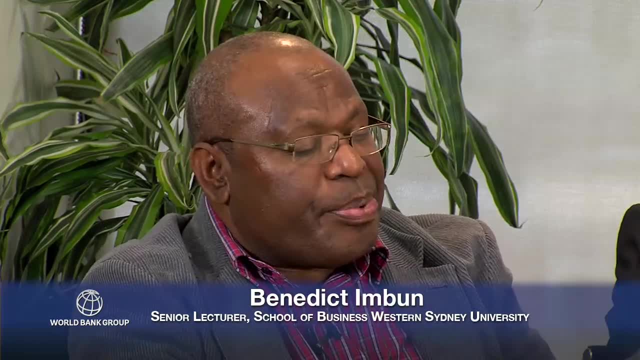 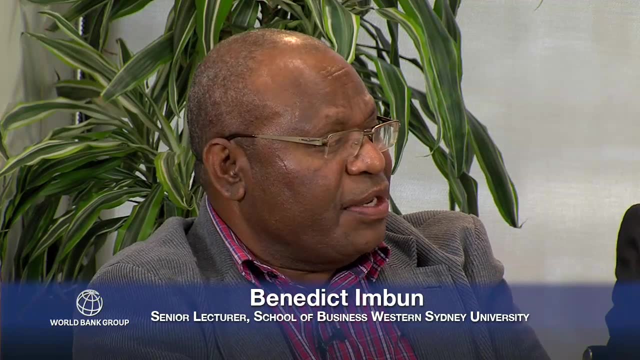 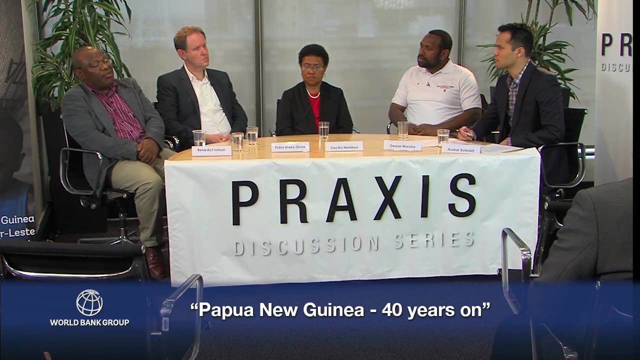 or transpiring or, you know, making it more practical to the taste or to make it more applicable to the people. it's a huge step. I mean, the donors are there, obviously trying to assist wherever they can, But, being a subsistence economy, a dominated economy, peoplealthough. 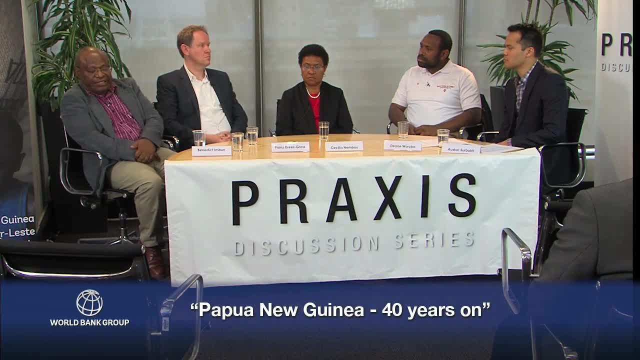 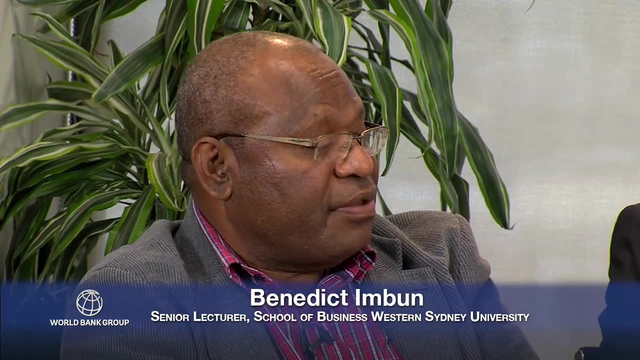 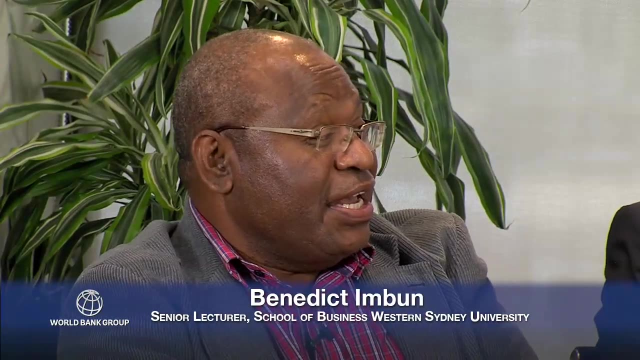 a lot has improved in terms of literacy skills, numerical skills and understanding of the economy works, But in order to achieve things, a government plan such as the Vision 2050 needs to be more easily understood. Otherwise it's an abstract stanza alone. 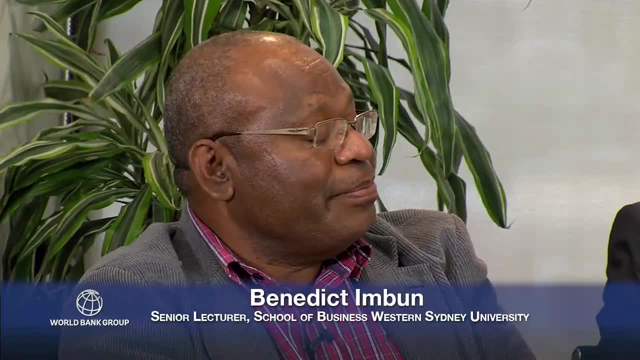 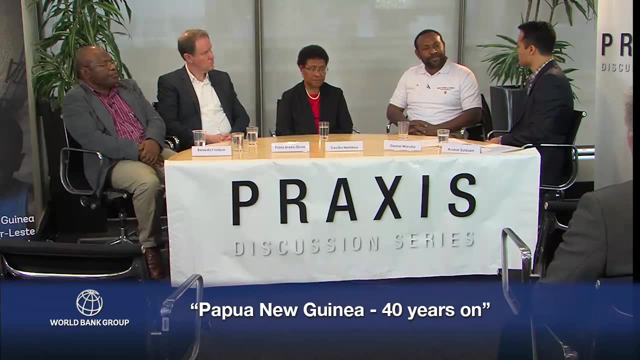 It's just a political document. Yeah, Okay, I think Vision 2050 is a great document. It's, first and foremost, it's homegrown. WeI was not there. I was not there at Independence, But when it wasthe Constitution was drafted it. 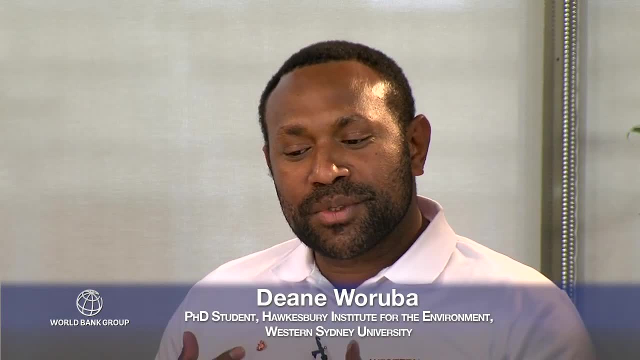 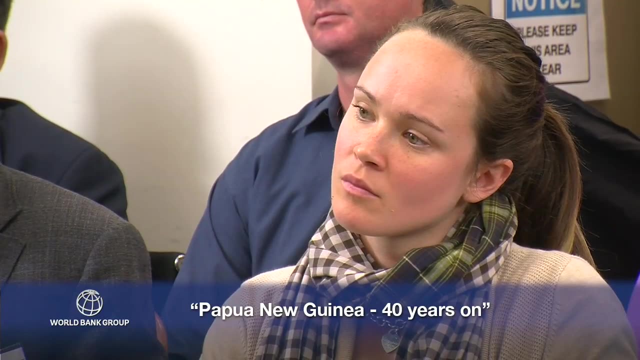 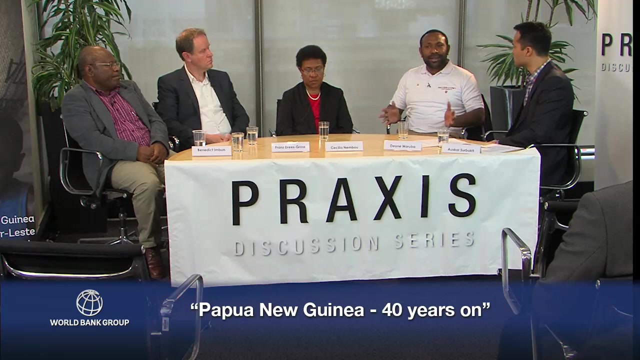 was homegrown And they reflected on societies and other countries that were more similar to ours, in Africa, for example, And likewise this Vision 2050 document brings that element as well. I don't know of any other country who's got such a strategic vision and where. 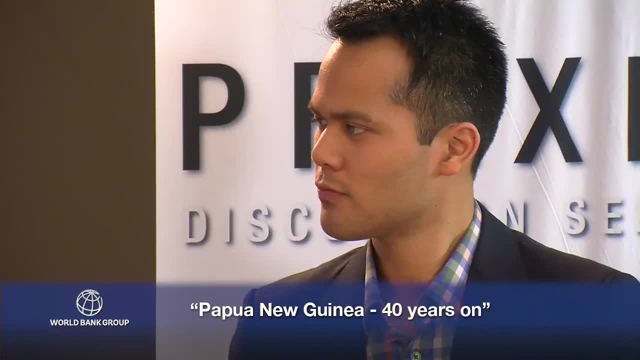 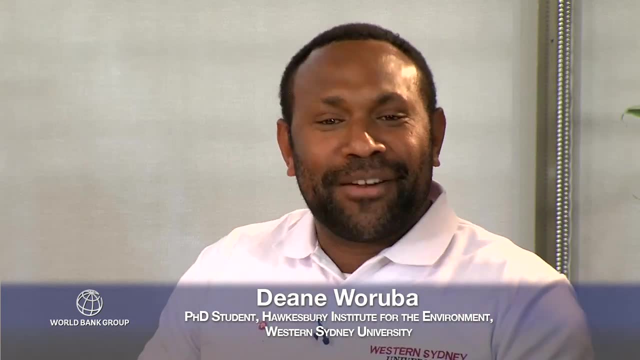 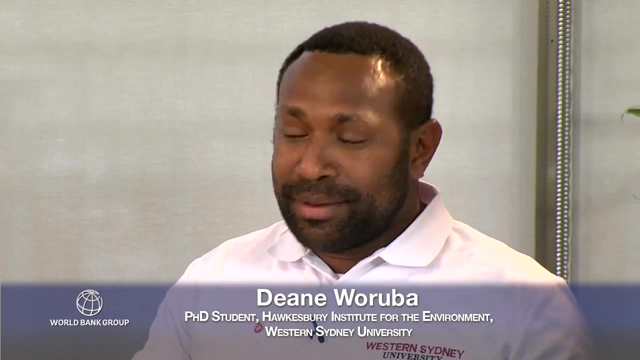 he wants to go, And we would like to get in a vehicle that is more inclusive- more inclusive of people knowing where we're going to drive to instead of just getting in a car for a ride. And this is what Vision 2050 is, And having that goal, it might be a little bit. 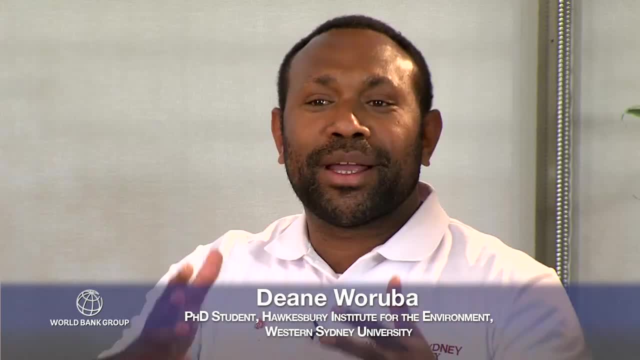 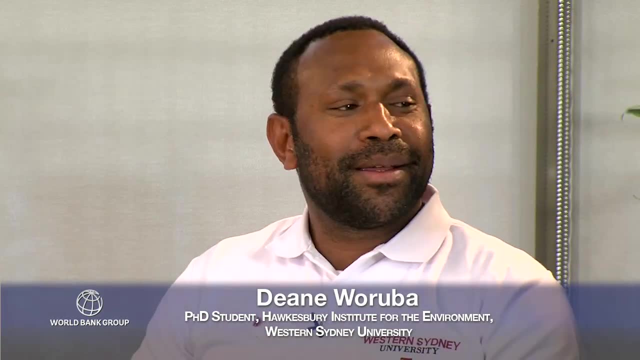 abstract for the moment, but it's the general direction in which we're going And, of course, the destination might change a little bit because you've got to stop, take a pit stop here and do that on the way, But you'll get to exactly where you want, which is those. 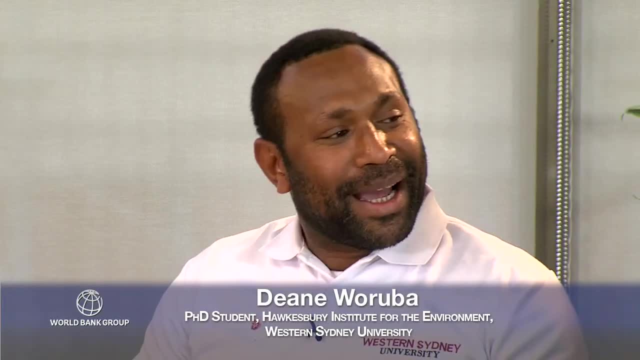 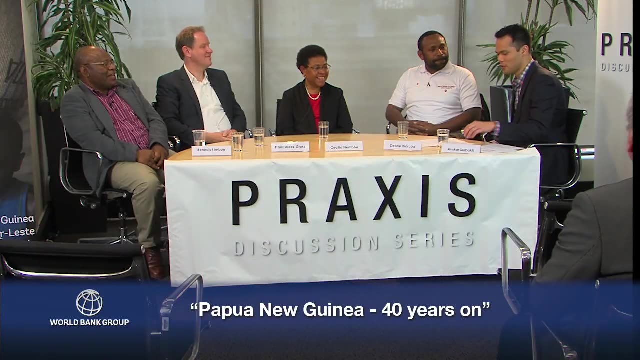 big words that Cecilia Tell us She said about being wise and happy and healthy and fair and happy. Yeah Well, it sounds like the document has won you over and, as Cecilia says, it is for the future generations. So that's a good start. Let's open to questions now. So those in Sydney. 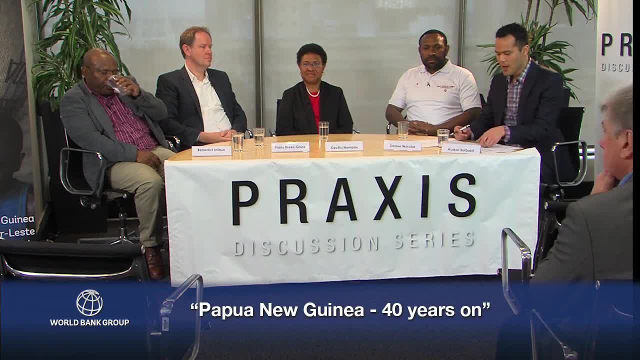 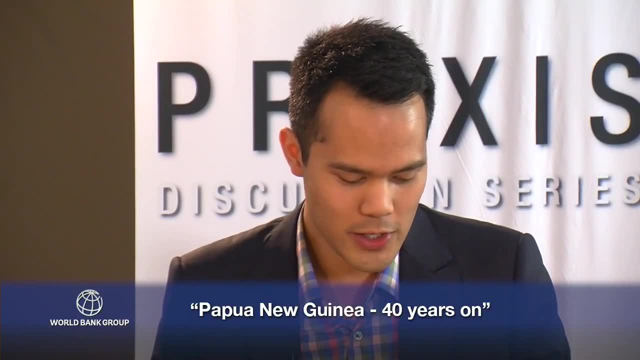 and abroad. please feel free to send them in. Franz. we have a question directed for you from the PNG office. PNG may be richer in monetary terms, but it's not necessarily the same in terms of income. How has that translated into human development? 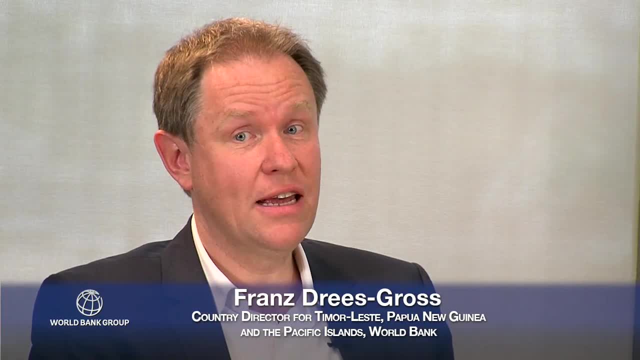 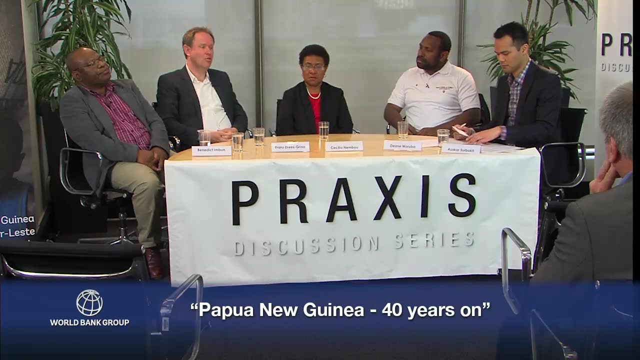 It hasn't. It hasn't fully. I mean, if you take, yes, PNG is richer in income than it was in independence, about 60% richer- But that growth in incomes hasn't been enough to really dent poverty. The most fundamental human development measure, of course, is just 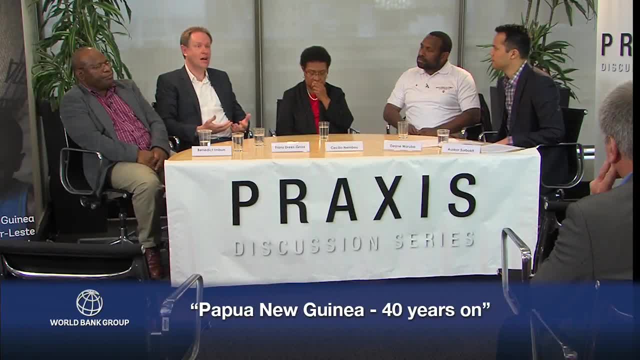 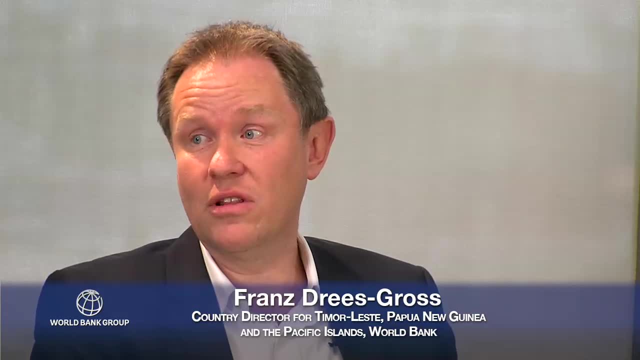 whether people are escaping poverty, whether they have enough for nutritious meals and basic needs, And basically on the basis of the best data that's currently available. there's a lot of information. poverty in P&G really hasn't changed since the mid-1990s. It's stuck at about. 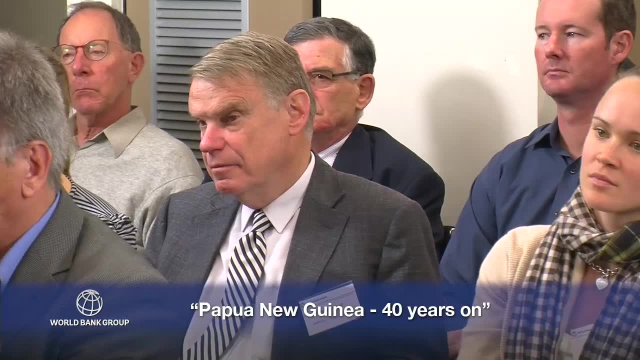 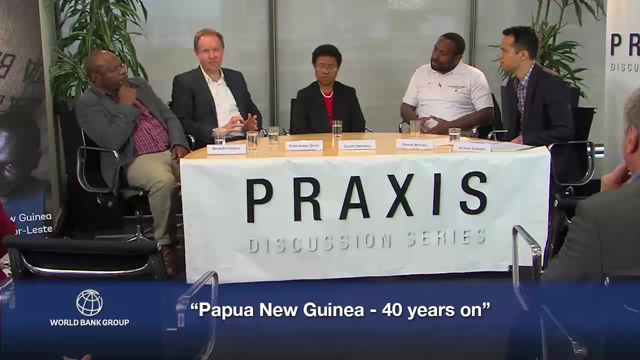 40% of basic needs- poverty. So on that level there hasn't been much development. I think on education there's been a big push in the last couple of years and I think very laudable and very, very much appreciated to get kids in. 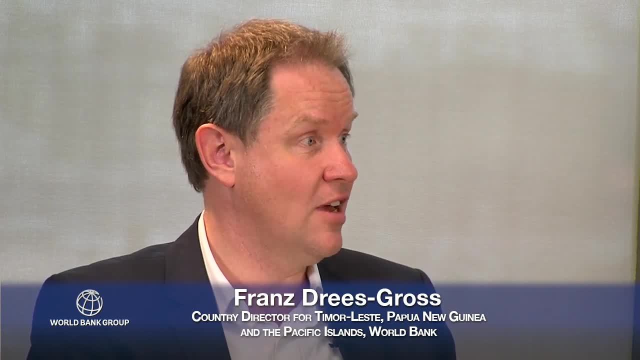 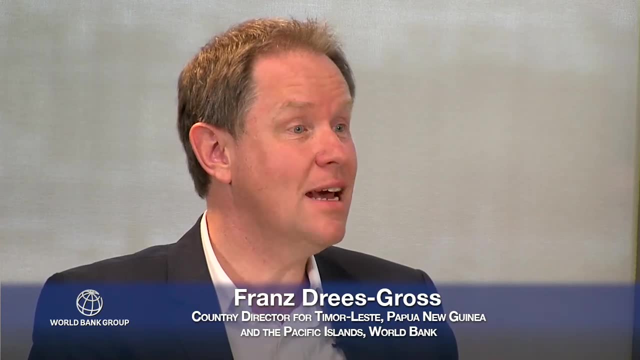 school. So the numbers in school are great. now They're 96% of primary age schools. kids schools are in school. But if you dig a little bit, only 10% of kids that actually graduate from primary school go on to secondary school. much, 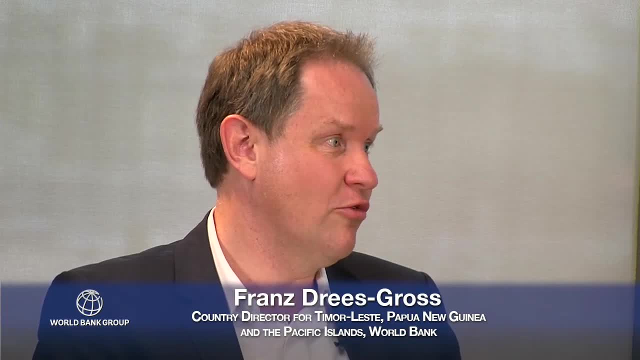 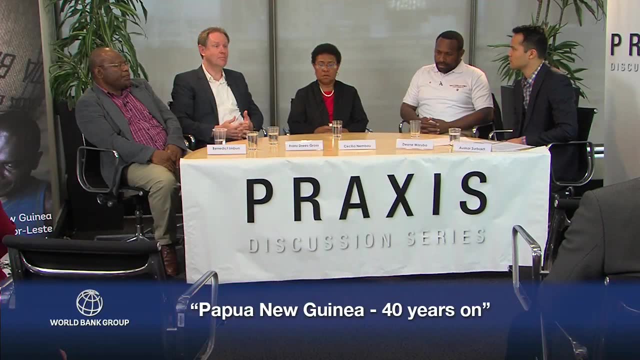 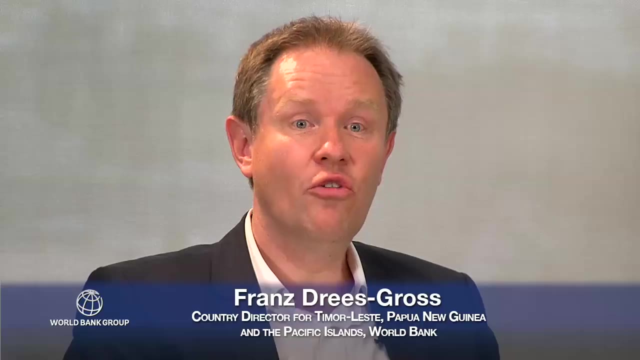 less to the universities where Cecilia will be working for them. And there's this whole bulge of adults who have never had this chance. I mean, we one of the things that came out of the household income and expenditure survey in 2010, when you surveyed P&G's population overall- 45% of all men in 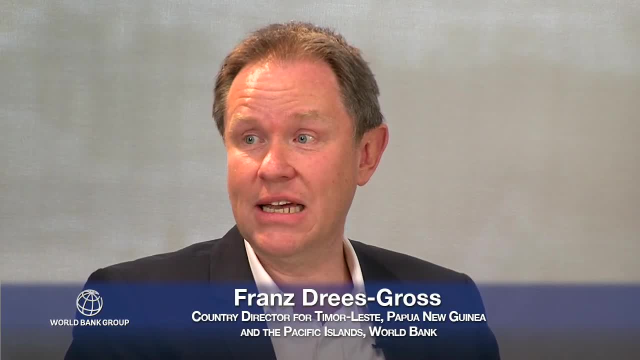 P&G were in primary school, So that's a big difference. So I think that's a big difference to see that there's a lot of the most successful students that were in P&G and 57% of all women in P&G hadn't finished a single year of school. 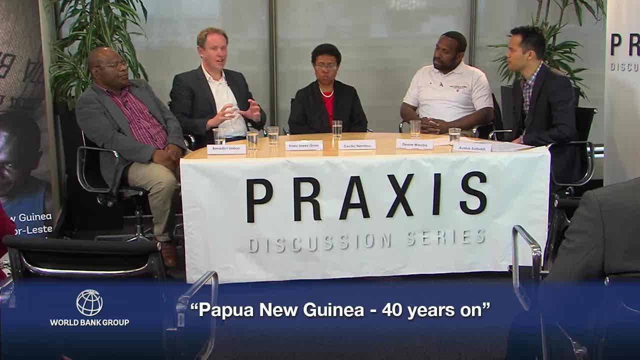 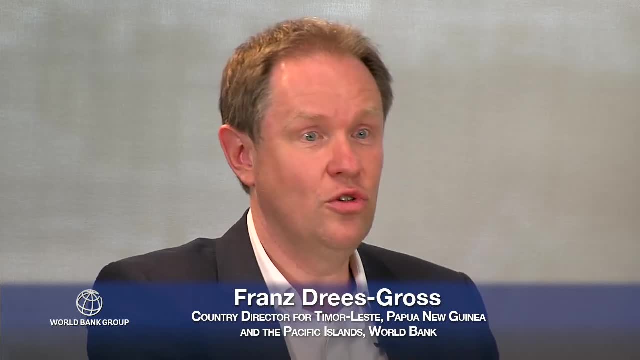 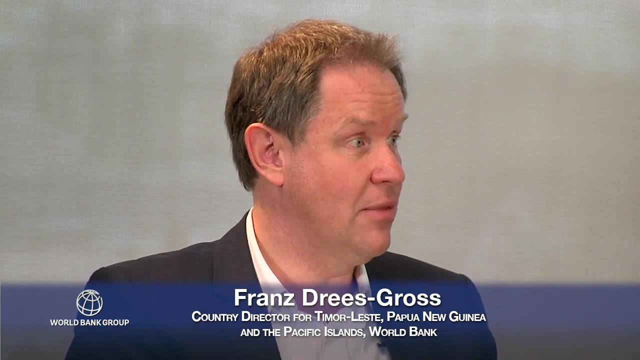 They may have set foot in a school, but they hadn't finished even one grade. So you've got this whole stock of people out there that has very, very little education and you know, as you bring them into primary school you start to change that. But this is a generational undertaking. So I think P&G has made a 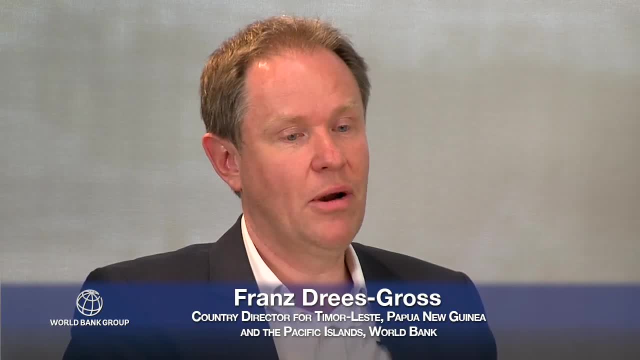 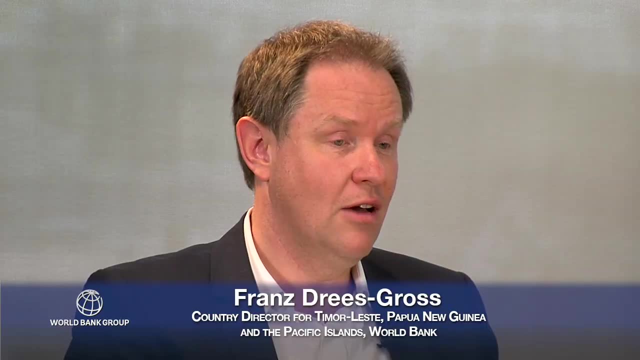 of physical assets. in P&G You have about twice as many kilometers of roads as you did at Independence, but a lot of towns are still really remote and cut off. You have 13% electricity coverage right now. That's the lowest in the Pacific. 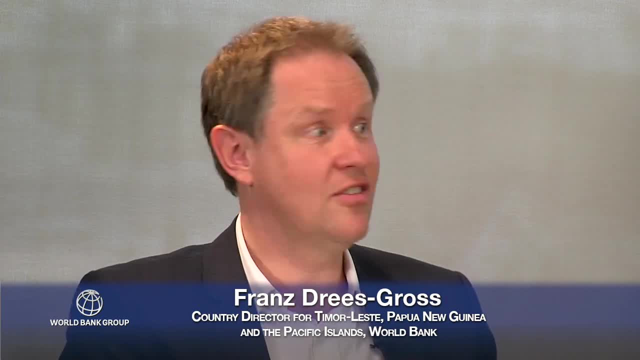 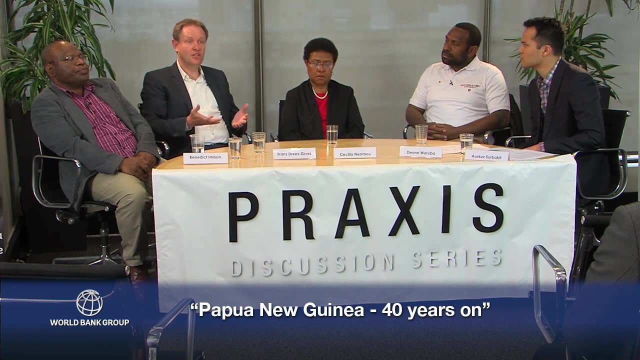 And it's not just households, it's also mines and other commercial users that have to self-supply. right now, Water and sanitation coverage is lower than it was 25 years ago, And it's partly because systems just haven't kept pace with population growth. 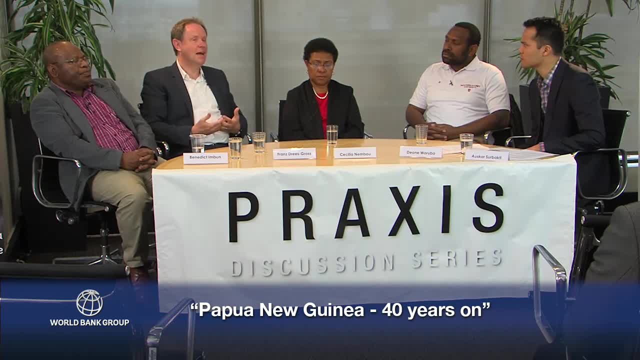 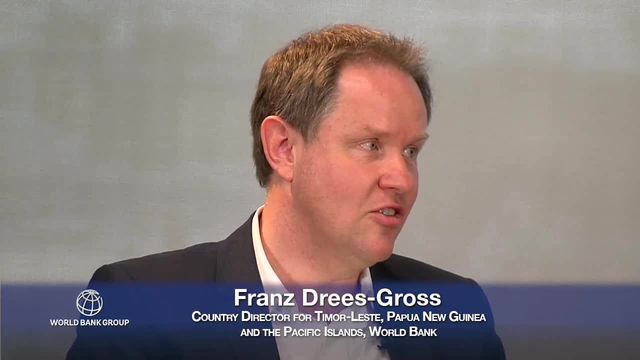 It's just about 2 and 1 half percent. So it's a big challenge. Despite all this, I mean I could just repeat these statistics one after the other. But here's why I'm optimistic about P&G despite these challenges. 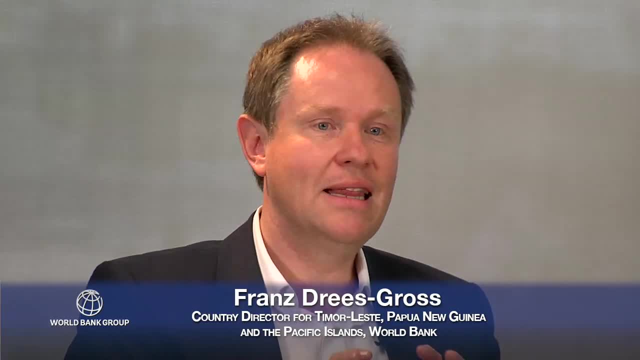 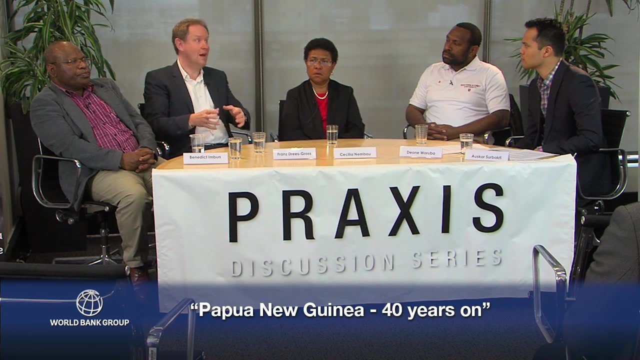 And I think it's because P&G is in a group of countries that has the natural resource base to finance its development. The big challenge is how do you take what's in the ground- the mining assets, the natural gas and other things- and turn it into human assets? 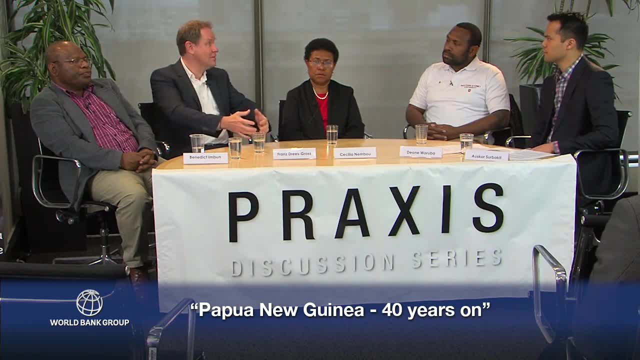 and physical assets, How do you turn it into healthy, educated people, And how do you turn it into roads, water supply, et cetera, And so there's good stories on how to do that. They've taken one good step just last couple of months. 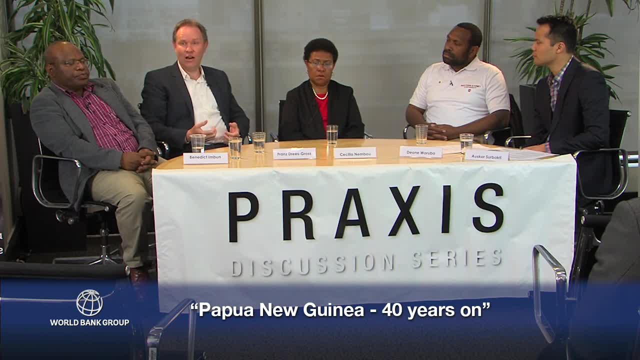 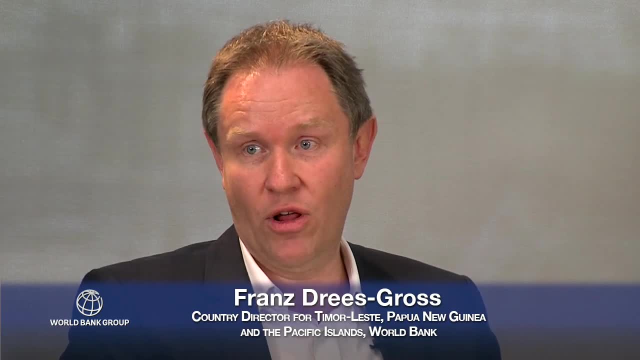 is to set up a sovereign wealth fund, for example. So at least what's taken out of the ground, what's paid in royalties and taxes at least, is accounted for. 50% of it flows into the sovereign wealth fund. We'd like to see that go up to 100.. 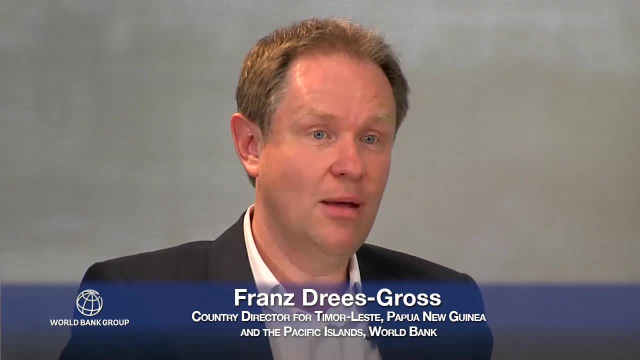 I know the government's thinking of that, But at least you've taken that first step to say: let's be transparent and accountable with what's coming into the cash register. And then the next step is: how do you do that? And the next step is when you take it out. 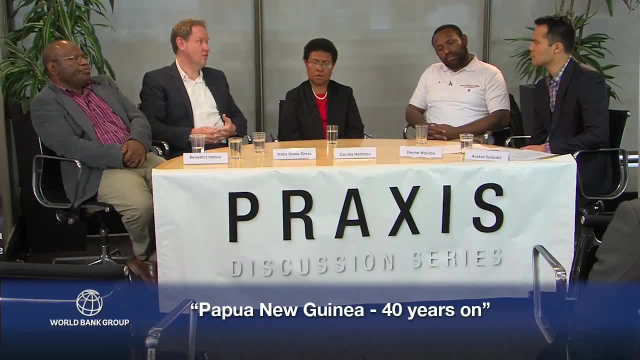 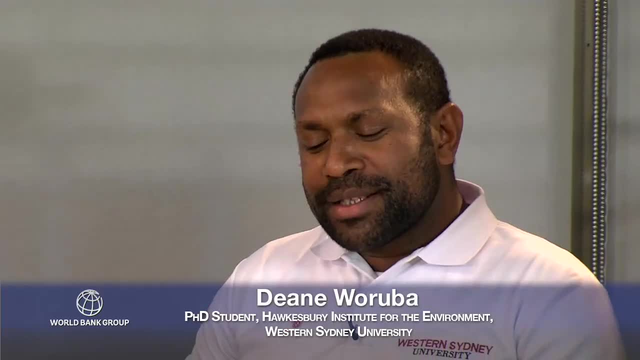 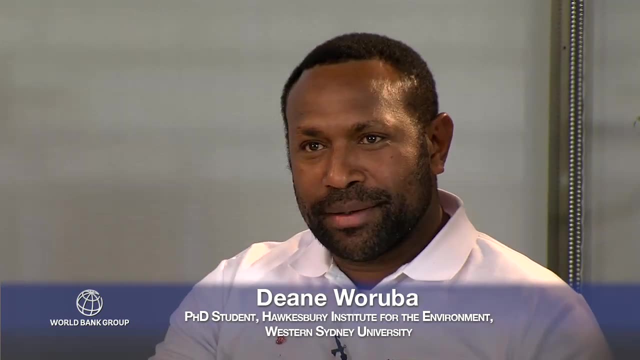 of the cash register. make sure that you get good education, good roads, et cetera, out of that. Excellent. Can I interrupt? I don't think it's fair to classify Papua New Guinea by the term poverty, looking at it as what we normally. 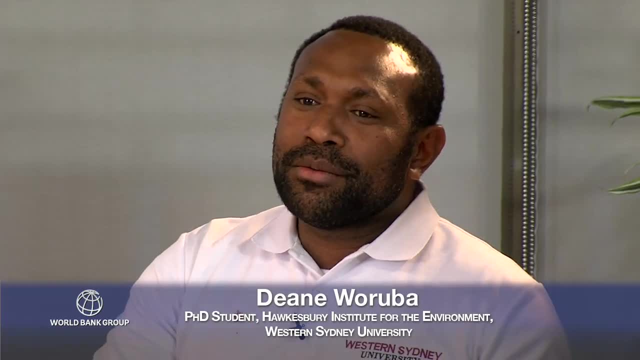 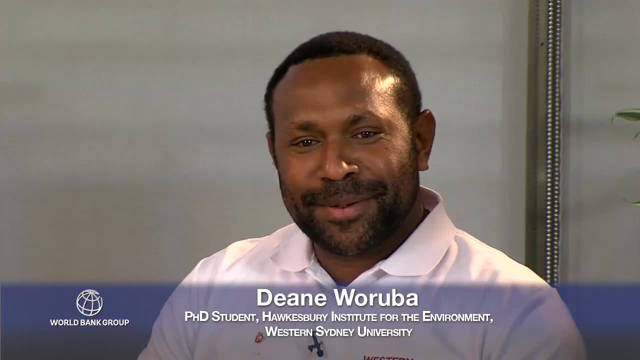 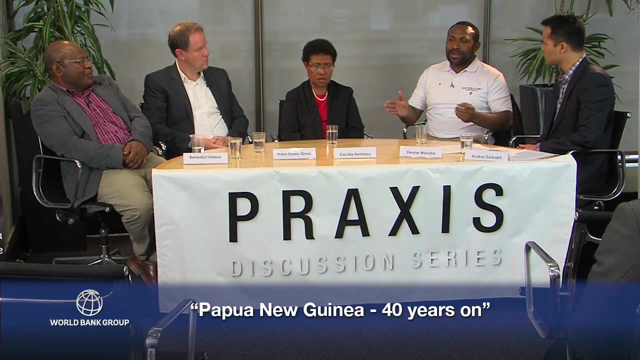 would perceive it in other countries because it's quite unique in the resources that we have for subsistence living. So the term poverty must not be seen as people are going through trash, or translated to: if you're using money as an indicator, They've still got plenty of food nutrition. 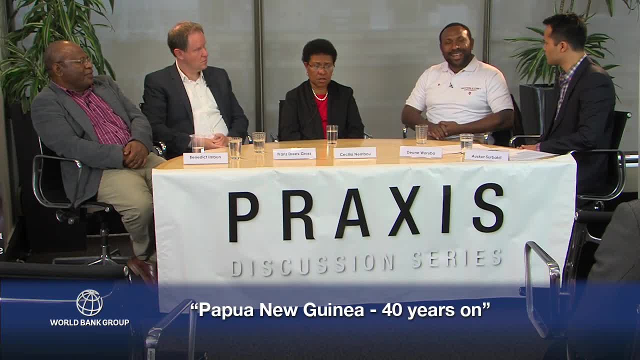 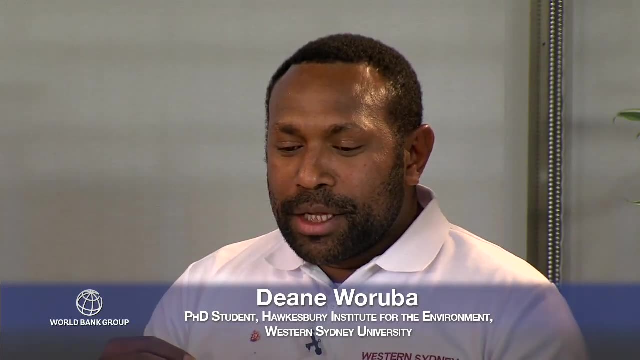 from other sources, But other statistics are still good. I think it's correct. It just could be interpreted a little bit differently for the case of Papua New Guinea. On the flip side, in terms of the sovereign wealth fund and moving forward in terms of development, if we can introduce. 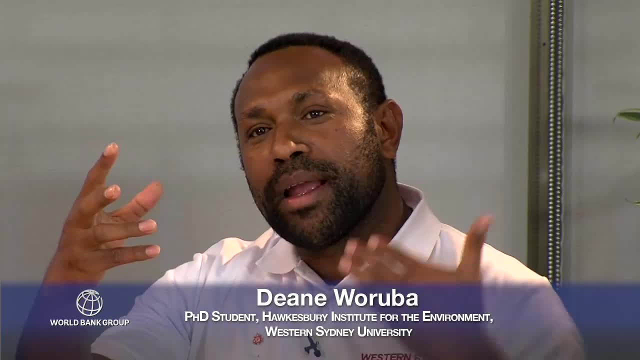 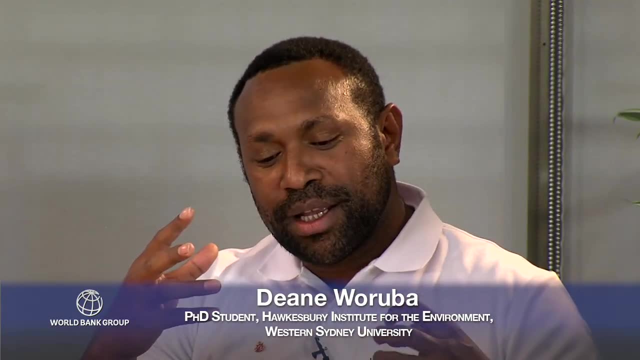 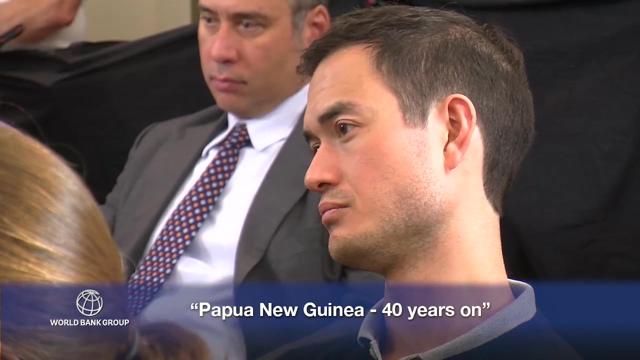 a higher paradigm, And I think that's what we're trying to achieve. By going up there, we force changes that will probably change the things that are holding us back: Issues of a global scale like marginalized population equality and things like that. 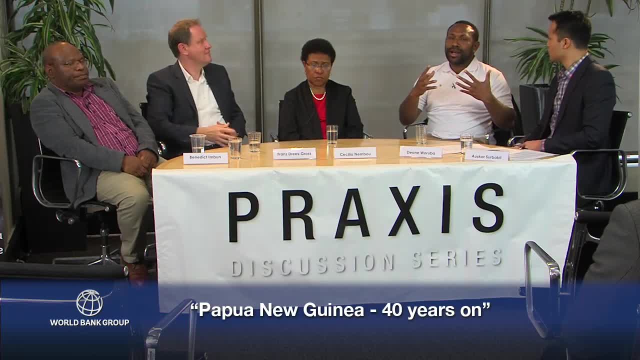 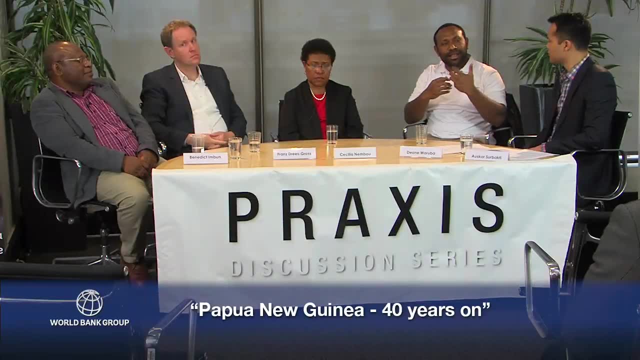 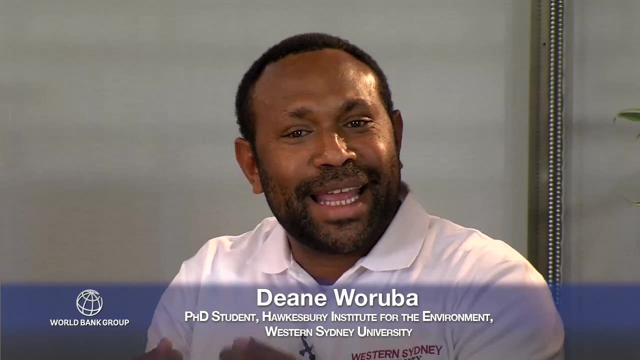 We come out at the other end with empowered people, having lost all these bad things that are holding us back in terms of development. So say, stimulating agriculture- Agriculture, which is my passion, That farmers pushing in money or giving them access to loans so that they want to do it, but you're telling them. 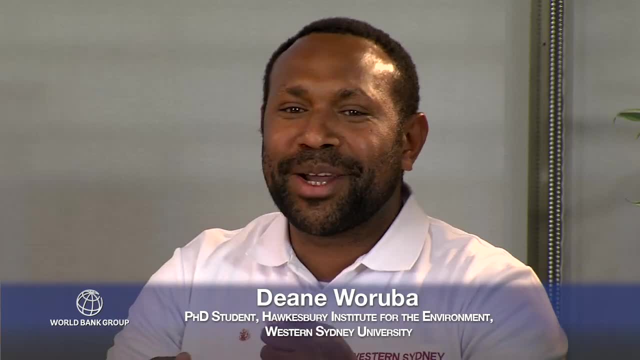 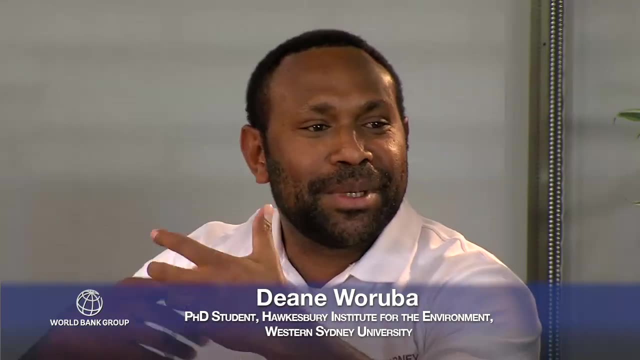 look, if you want to get this loan, you've got to do this and that and provide proof that you're not abusing the marginalized population or giving them an equal benefit in this, And then these things will drive this change for development in a positive way and it'll be very sustainable. 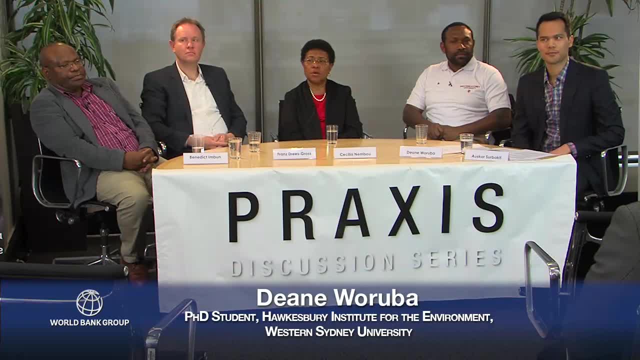 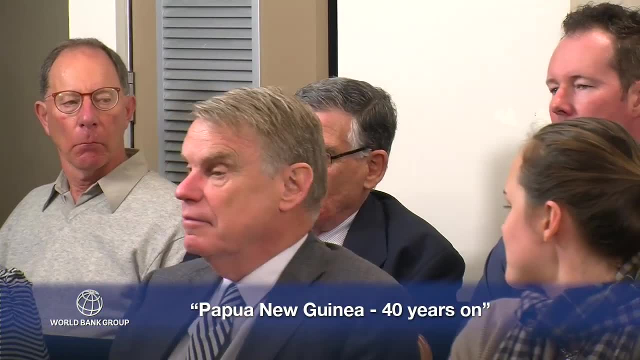 Excellent, Let's see if there's a question in Sydney. Yes, sir, Yes, My name is Ted Wolfers. I had a couple of questions which I think follow from the points just made. The first one: it seems to me that there's a problem about the kinds of statistics. 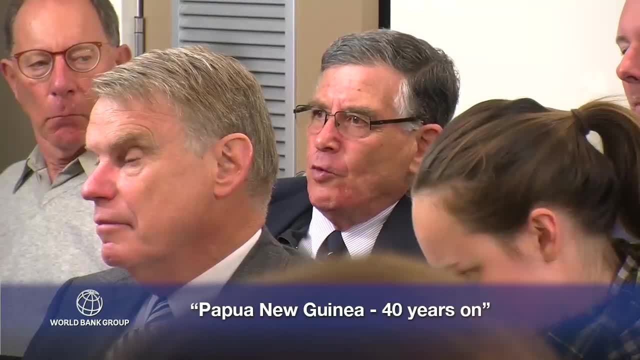 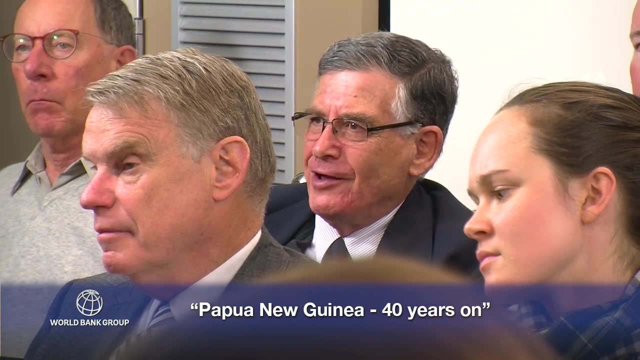 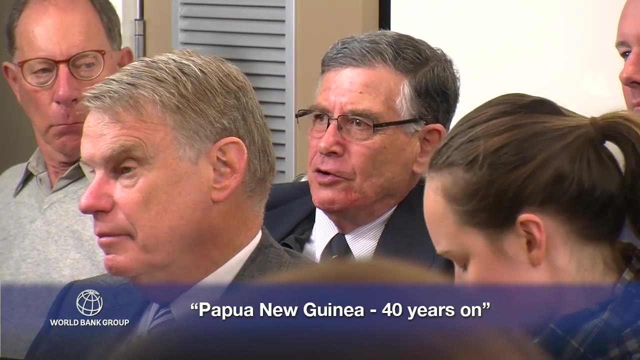 we're using that. for example, one of the positives of the Papua New Guinea education system is the disproportionate number of Papua New Guineans now going overseas and the skill loss that's involved, And so I want to look very much beyond the statistics of whose? 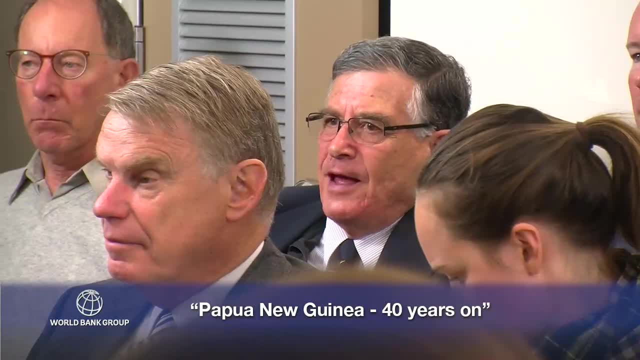 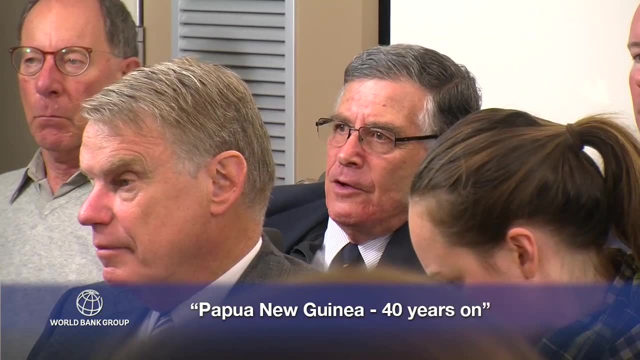 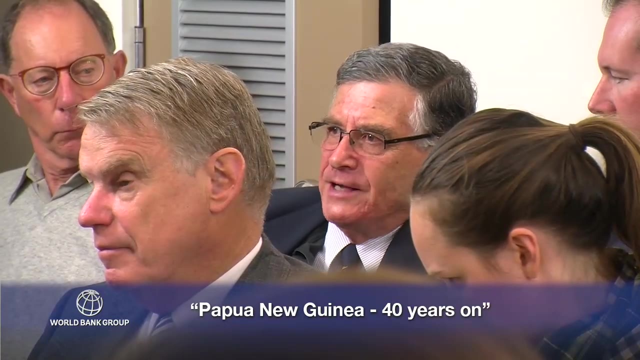 students are graduating to where they end up, And that might have very serious implications for government policies and for foreign aid programs, for example, And I think that's when I look at the World Bank statistics and others, it's really quite worrying because the figures are so high. 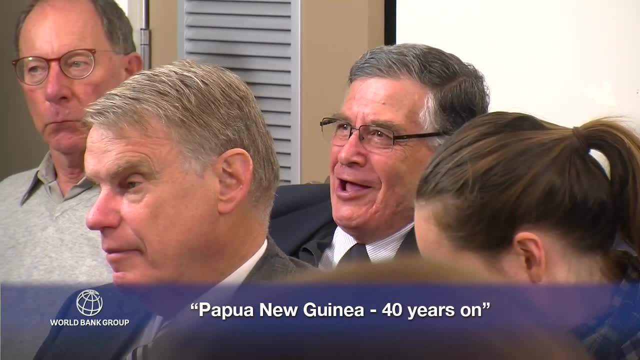 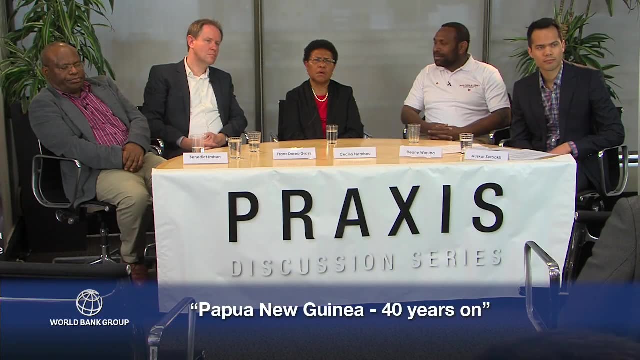 but clearly the people are able enough to get jobs all over the world. So you know, and no one wants to stop them- Similarly, the disincentive to joining the public service- that increasingly the really good people are finding other ways of working. 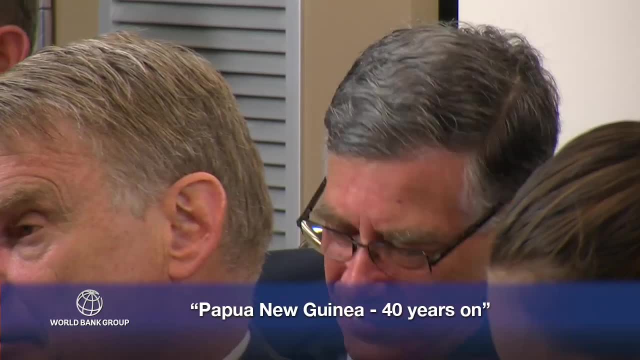 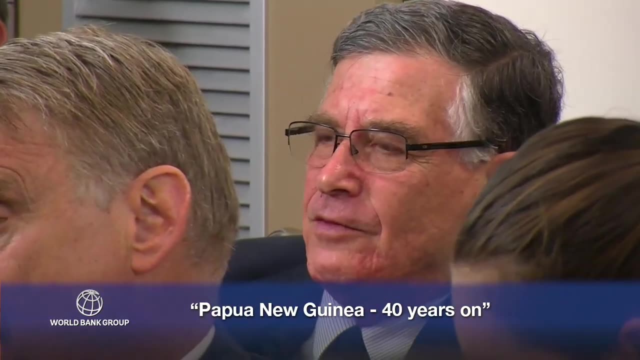 in the public sector but not joining the public service. I think that's my first question. The other one is, which follows directly from what Dean was saying, was that I don't think that the poverty measures tell me anything. I want to know. 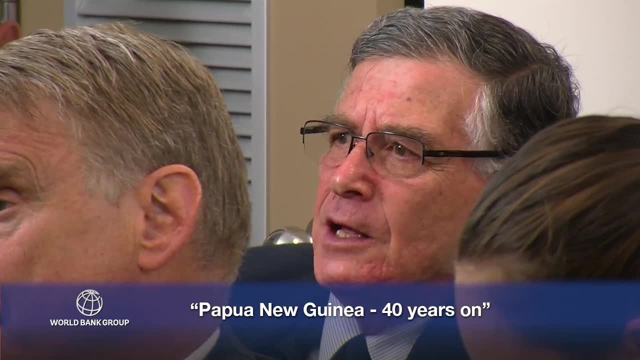 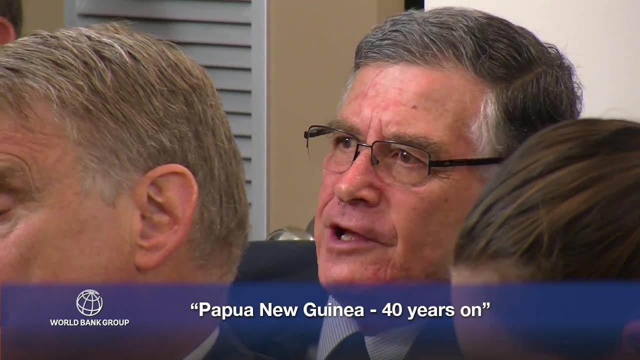 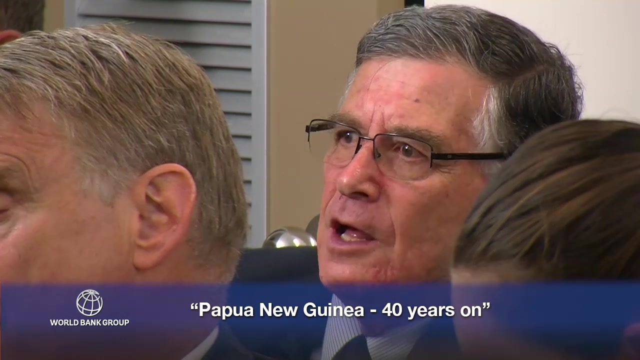 or very little. that I want to know. that's perhaps put too strongly, But it seems to me that the issue in many parts of Papua New Guinea is not poverty but impoverishment, That people are actually falling further and further behind not just healthy lifestyles, which is a real issue, but also behind aspirations. 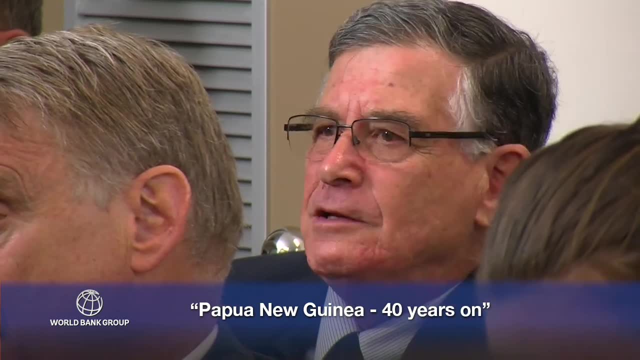 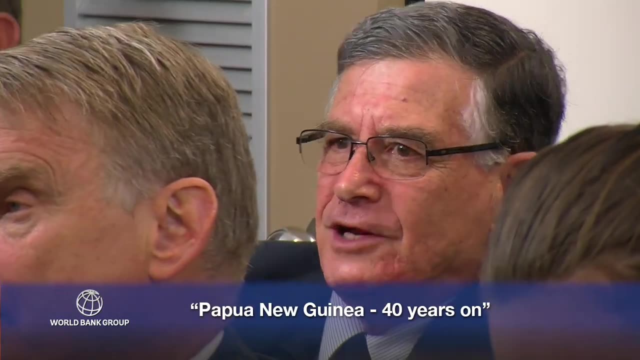 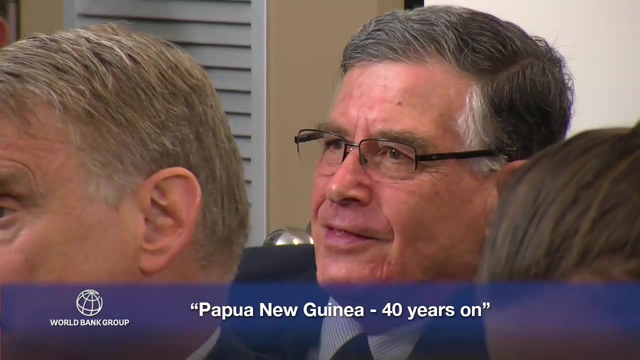 That, in fact, aspirations have changed massively and people are engaging in antisocial conduct, in some cases, not because they're poor in the traditional measures that are being used, but because they're relatively impoverished compared to what they want, And I think I'm just suggesting that it would be very useful. 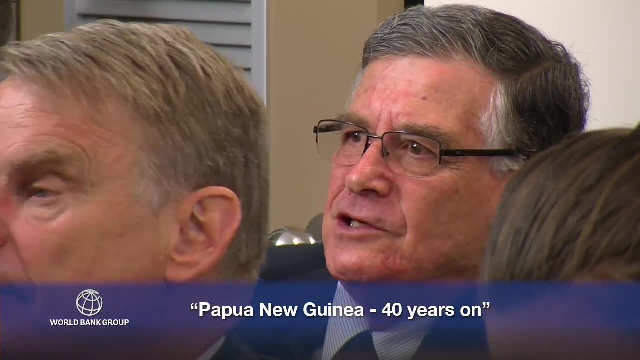 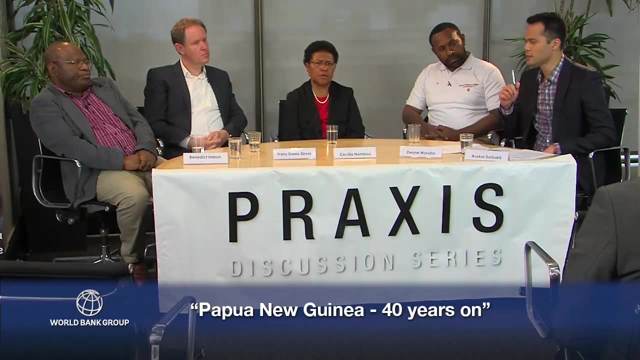 to hear the panel members talk about these kinds of issues and the kinds of measures that we might use to address these, what I would regard as very important issues. Okay, thank you. Thank you for that, And let's start with the first point, the so-called brain drain, I guess. 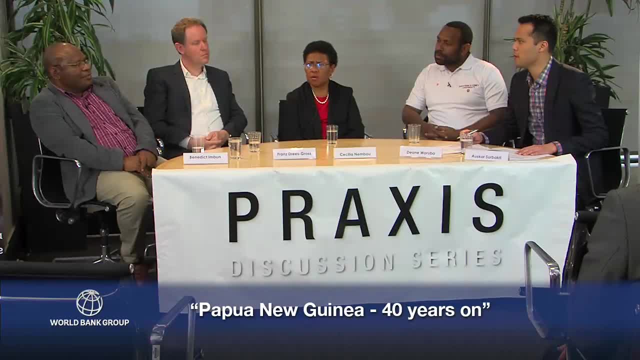 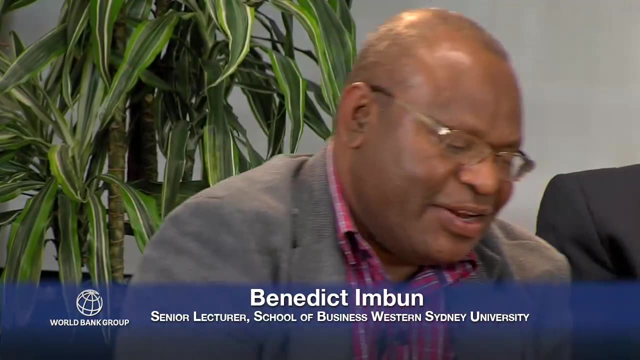 That many countries experience, developed and developing, but it can particularly have an effect on those emerging countries. Ben, you feel quite strongly about this brain drain. What are your thoughts? What are your thoughts to this, about it? Well, brain drain obviously has to happen. 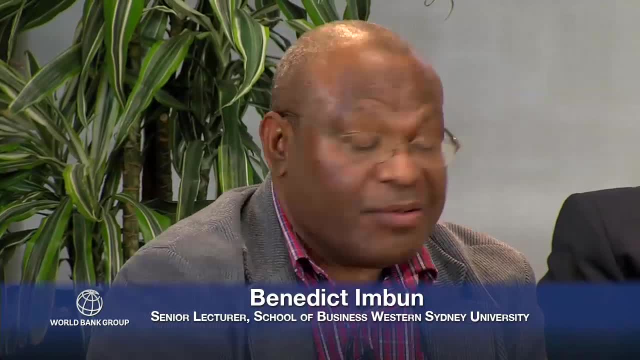 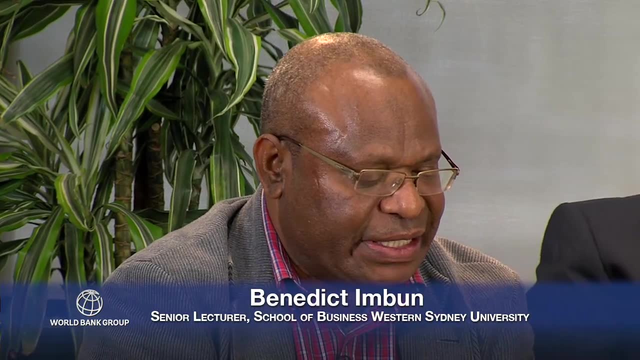 I mean, obviously, when there's a demand for labor or you know now that we are in a globalized world, people move and that's what people are freely doing. But, as I mentioned at the outset, there are some 1,000 plus number. 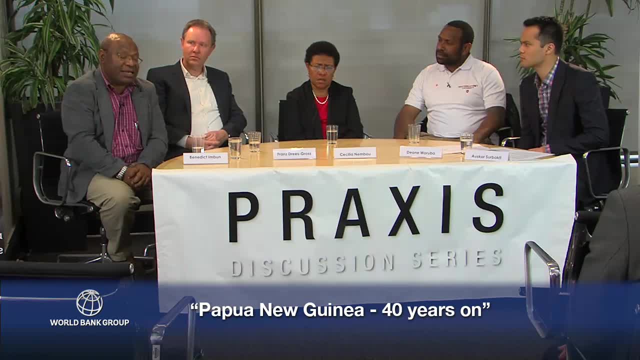 of Papua New Guinean miners in Australia and they've been exposed to, you know Australian style, you know working arrangements, running mines and with Australian employers working in all over the place in PNG mines. So they came here when the mining boom started, you know, a few years ago. 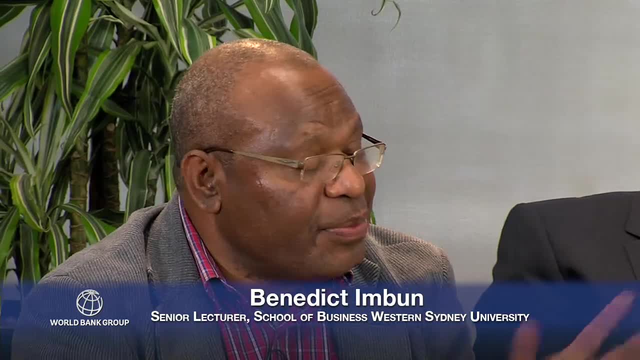 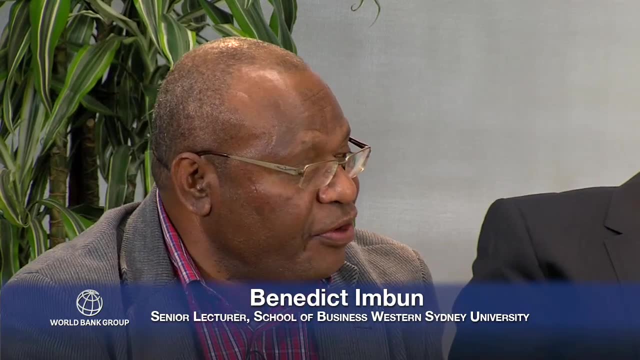 And so that needs to happen. I mean, it might not be a significant number for a lot of countries, since migration has been a way of life for them, But for PNG obviously there's a vacuum, you know, in terms of for the years, you know. 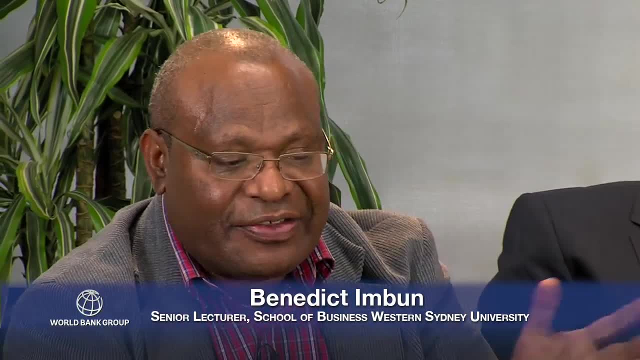 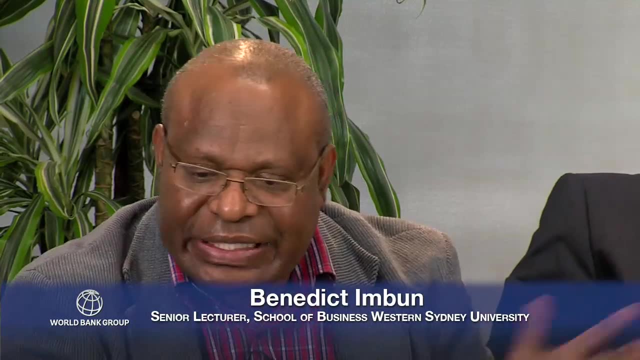 a country has built up all this skill, It's built human labor and then they start to migrate. But the PNG- I mean the mining sector- is capital intensive and there's a dual salary and expatriates and a bit more than the PNG counterparts. 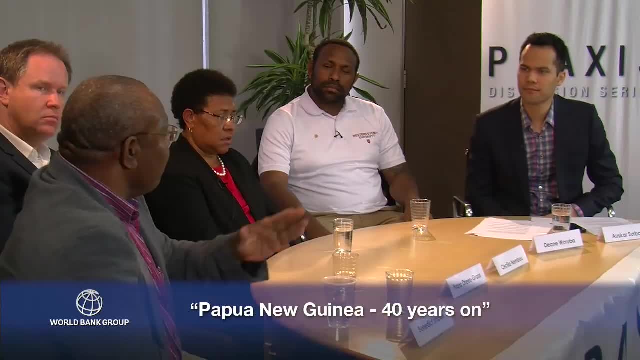 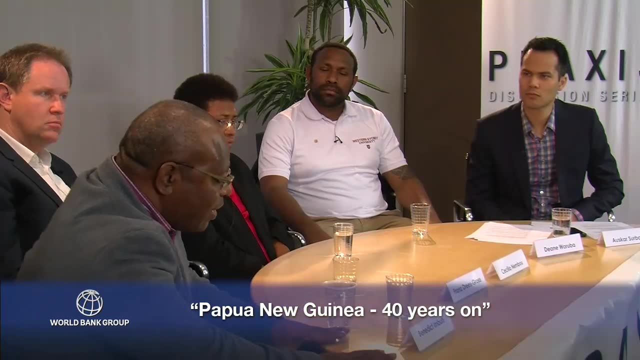 and it goes for the public service and other things as well. So obviously those things are happening And, as Ted was saying, I mean statistics are relating to that. Those things are happening. but what's happening is statistics is a development issue in PNG. 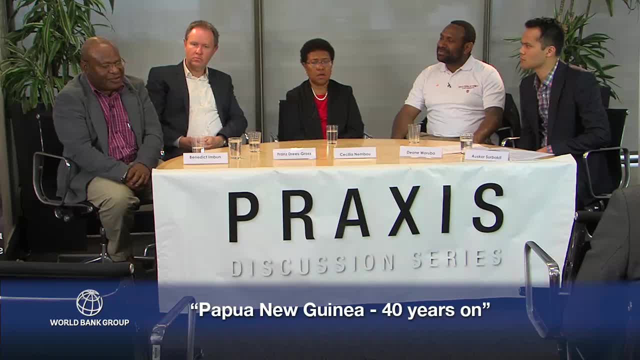 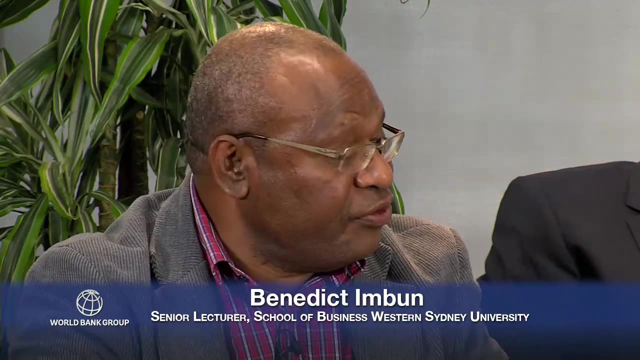 Policies are major And if you automate in a vacuum supply of labor or graduates to the labor market or demand for it, the reliable statistics is not there. Reliable statistics is a development issue. It's not aiding the development issues in terms of good quality policy making. 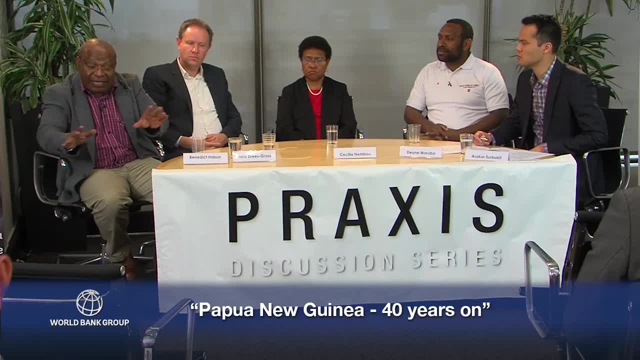 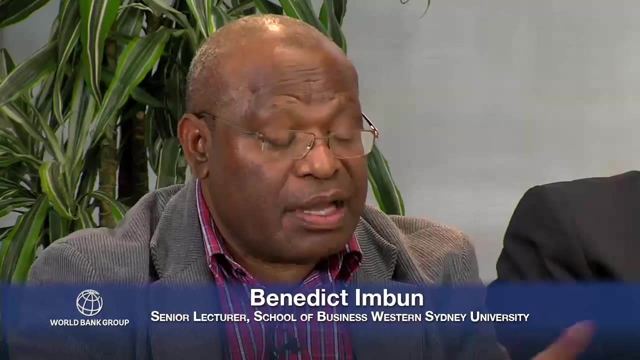 And unless and until we reconcile that major issue in terms of what we want to achieve with quality figures, we won't be able to achieve that. So I think it's a big challenge for a lot of these in 2050.. We talked about- and to run a country on a complex scale with matching good statistics. 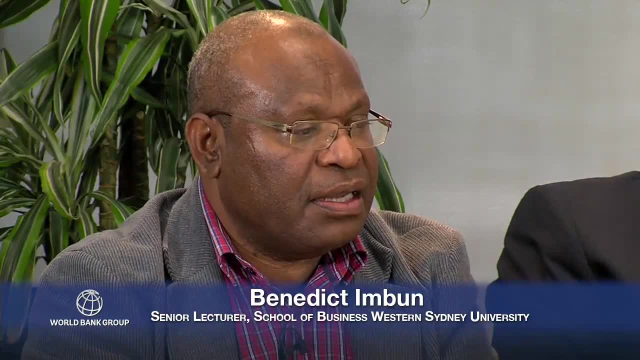 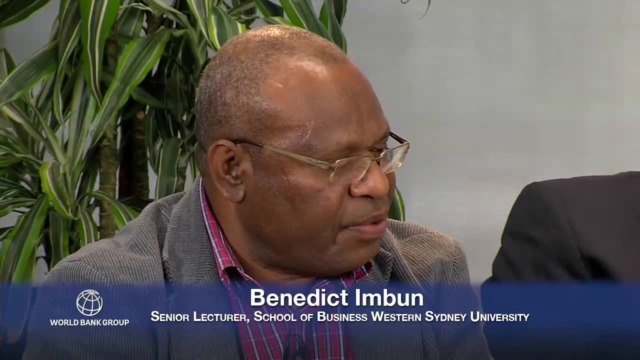 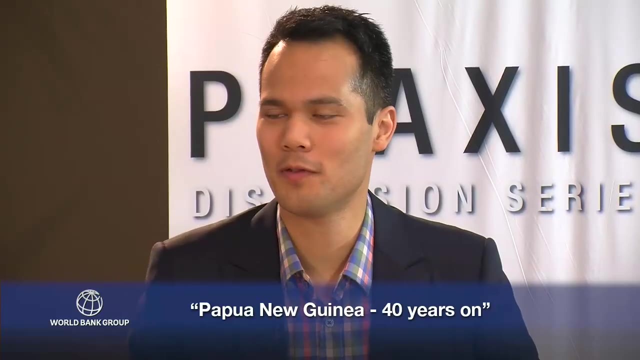 with good policy. it's a huge challenge And a lot of documentations have been done for the need to come up with reliable statistics. Obviously, we have the statistics obvious, but it's not happening. Okay, So it sounds like it's a. it's quite a divisive, potentially divisive- issue in terms of how. 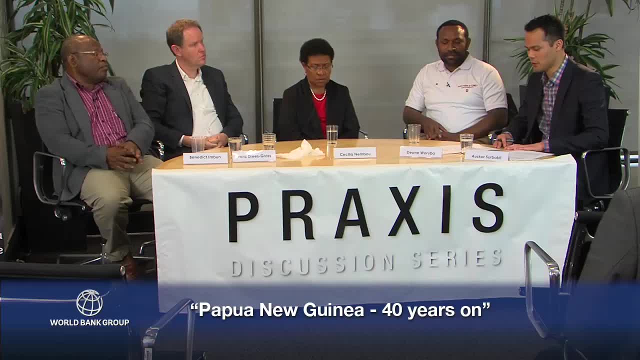 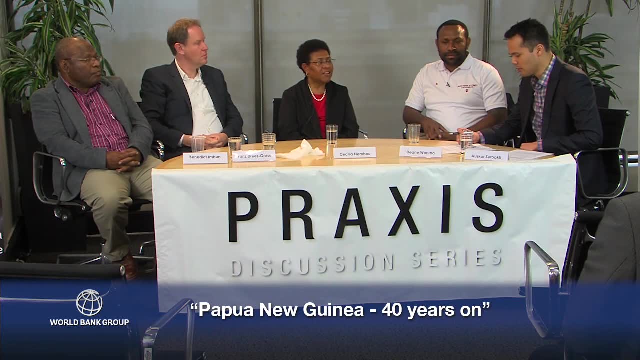 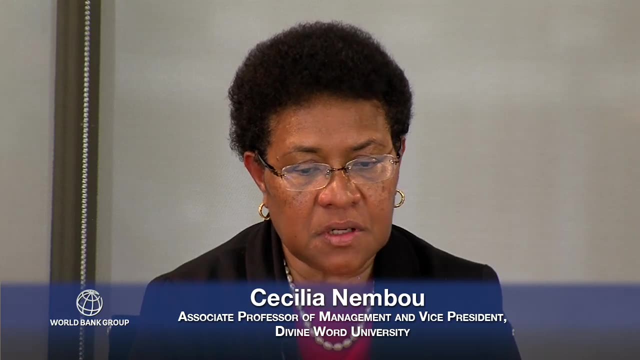 you relay that the development of a country. But let's move on to another question from Solomon Islands, directed at Cecilia. How can the government use the income it enjoys from the resources sector to better invest in PNG's education? The government needs to direct. 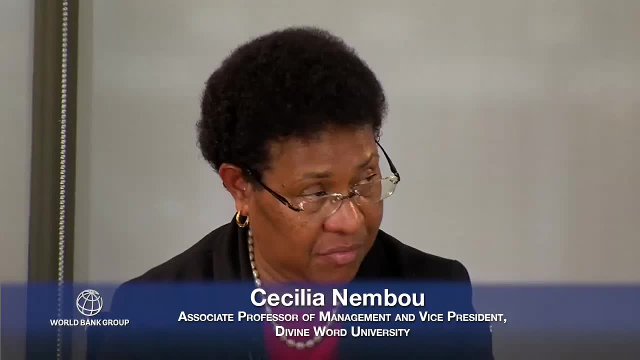 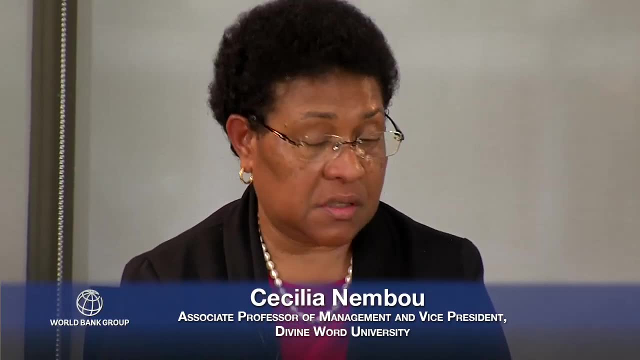 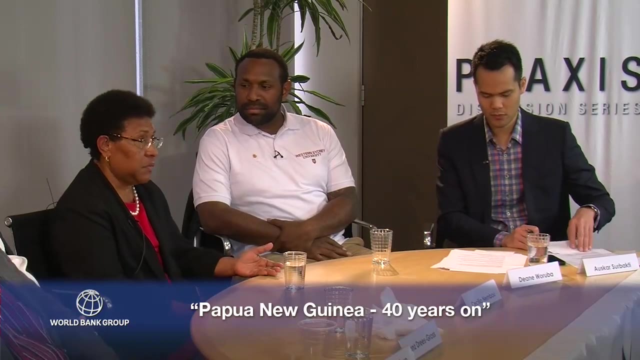 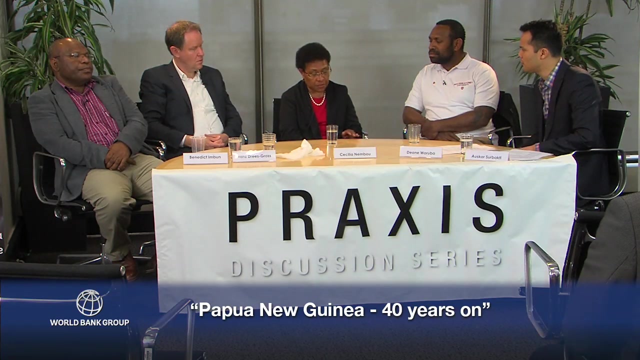 or manage the funds carefully in such a way that the different levels of education can be addressed. So, for example, higher education has been underfunded for the last maybe 20 years or so, as far as I can remember. The government needs to be able to fund more education, more of higher. 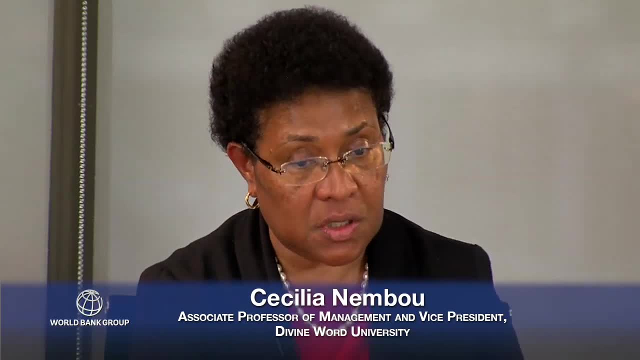 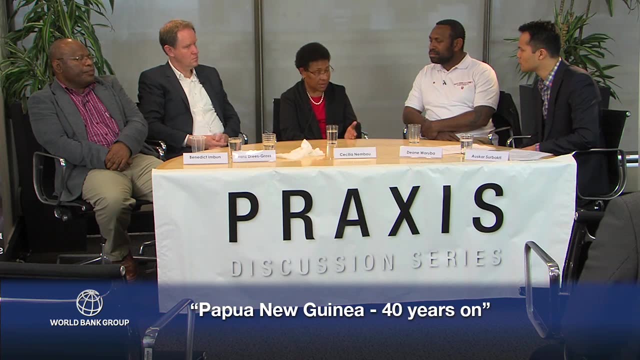 education. Recently, the government, as well as our development partners, decided that they should fund general education, And now, I think after 10 years, they realize that they need to actually pay a bit more attention to it. So, for example, higher education has been underfunded for the last. 20 years or so, as far as I can remember, The government needs to be able to fund more education And now- I think after 10 years, they realize that they need to actually pay a bit more attention to it. So, for example, higher education has been underfunded for the last 20 years or so, as far as I can remember. 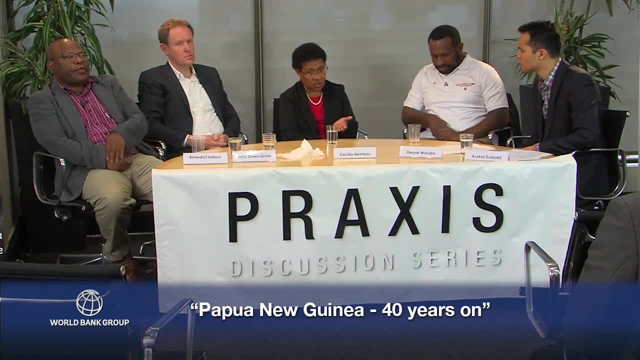 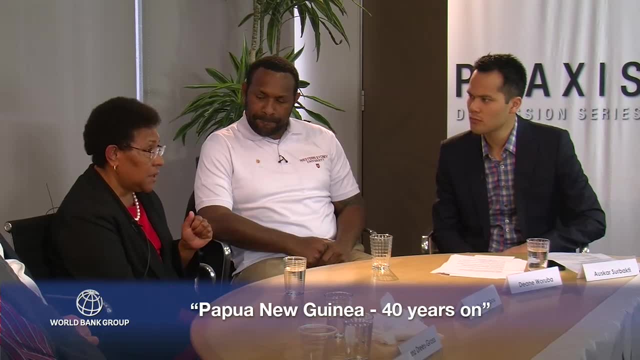 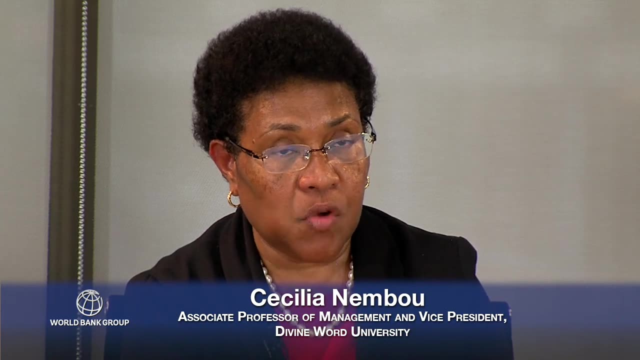 Because they build up the general education, and then there became that blockage And so something else has to happen. So investment in higher education is critical. in my view, More funds need to go to the rehabilitation of infrastructure. salaries for academic staff, I think the point. 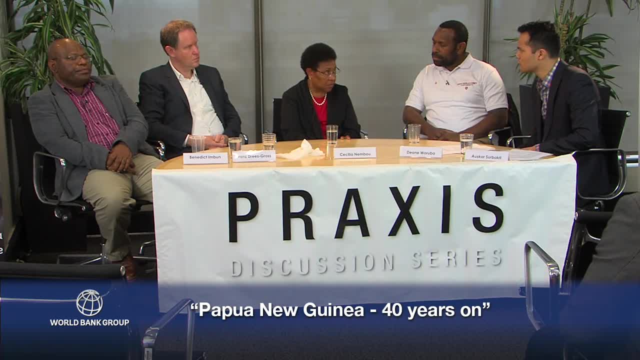 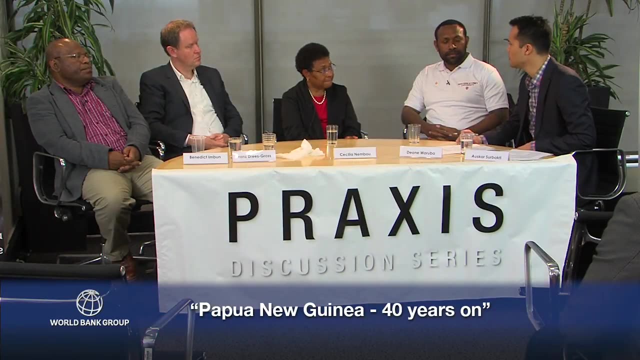 that Professor Wolf was alluding to was: why are the people going overseas? The salaries for the salaries are not equitable and not fair. The dual-based salary system in the public sector is not working. Can you just sorry to interrupt. can you explain the dual-based wage system? 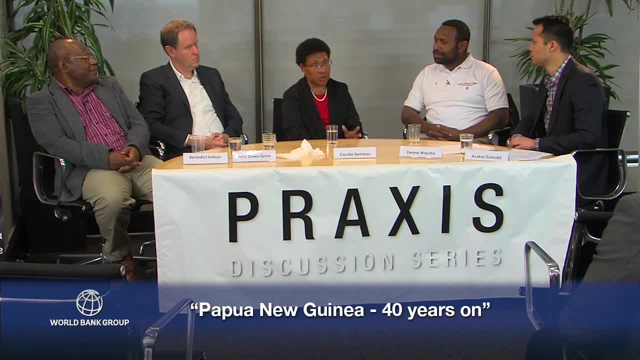 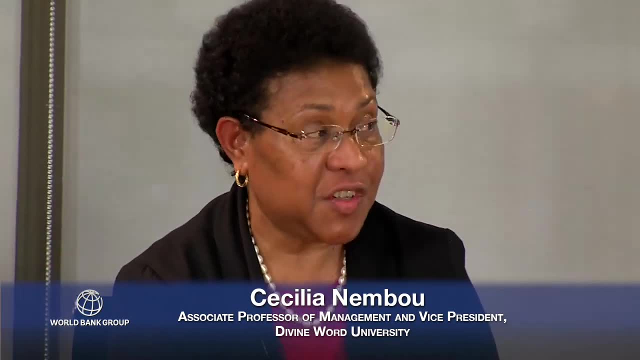 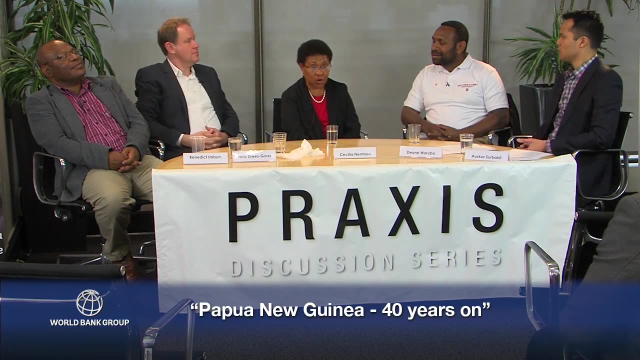 The dual-based system. some people will tell you that the dual-based system is no longer there. That is a matter of debate, because I've been there since independence and I know that it is still there. The dual-based system is where, in the colonial days, the colonial 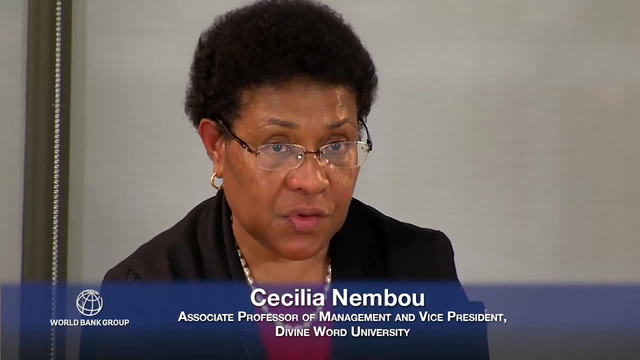 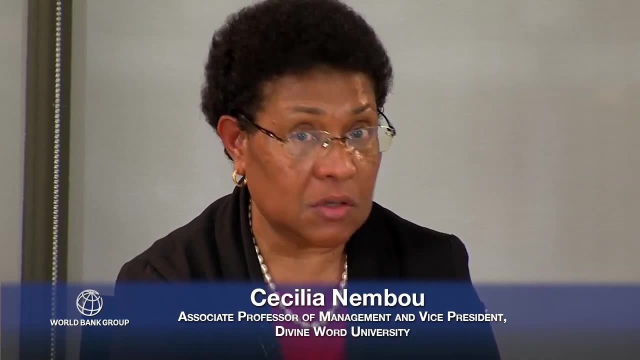 administration actually set a different set of salaries. Actually, the Australians had one system, the British people had one system, the New Zealanders had one system, Papua New Guineans had one system. Now, it was that way in the colonial days because there were 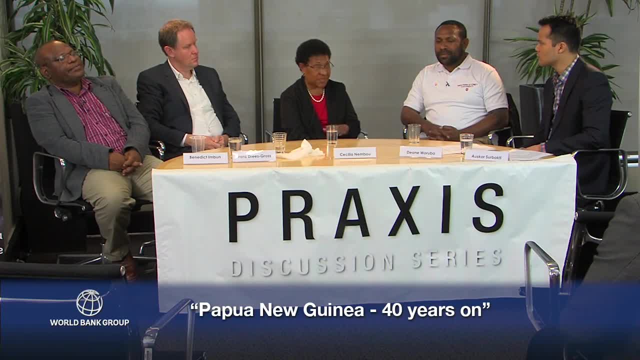 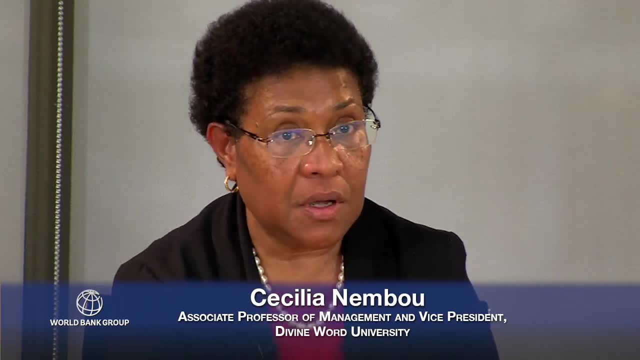 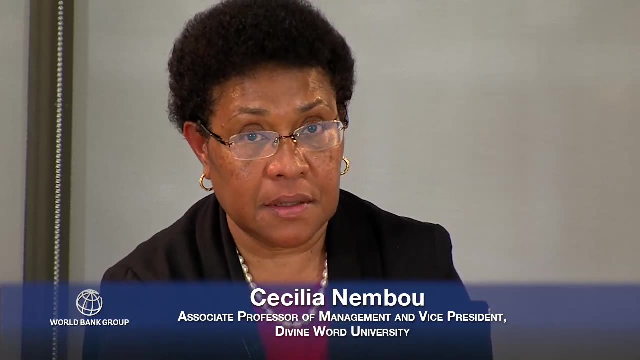 very few educated Papua New Guineans. That legacy unfortunately, in my view, has continued. It's disguised in different forms, Like right now: for academics they have domestic market allowance and international market allowance. They say, for example: unless Papua New Guineans 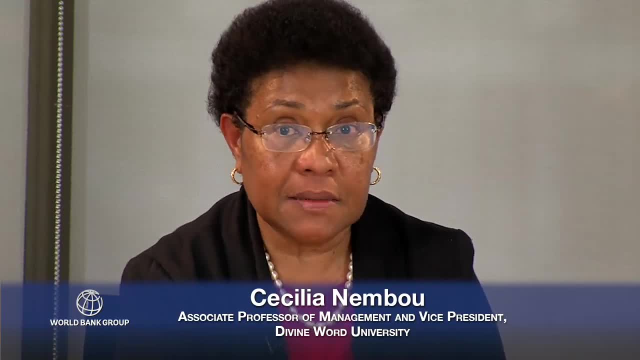 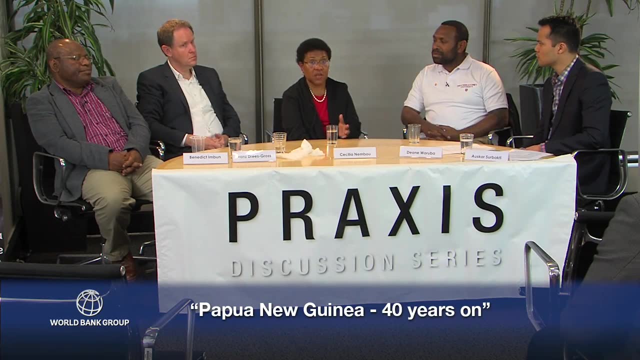 can demonstrate that they are marketable overseas, that they must continue to get a domestic market allowance. We know now clearly from what Professor Wolffers is saying that Papua New Guineans are quite marketable overseas. We have on our table, here on my screen, a 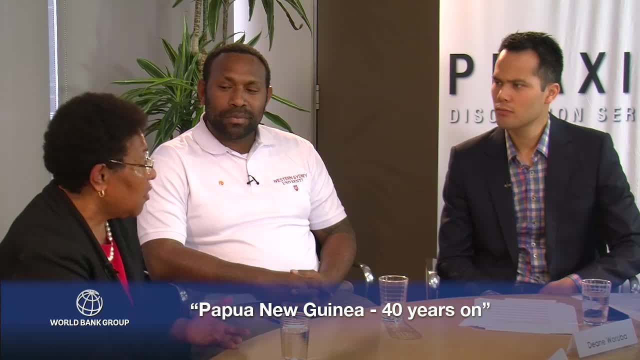 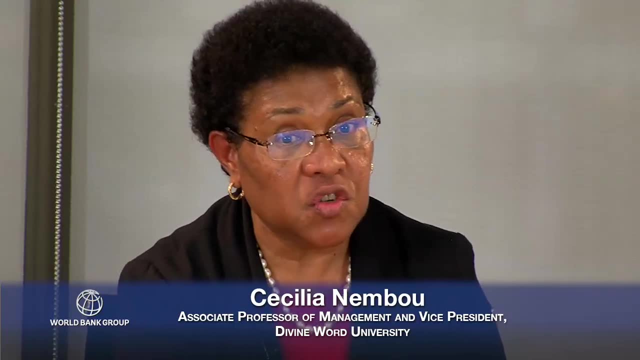 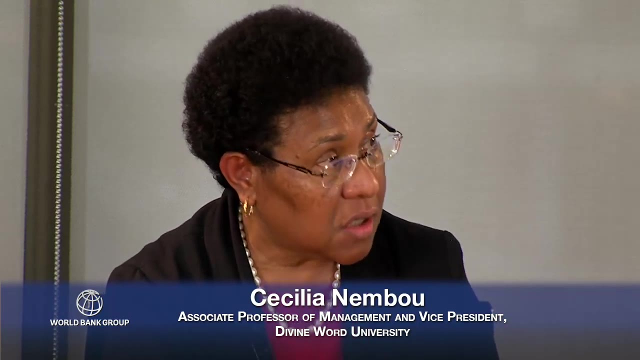 colleague, Dr Imboon, who actually is working overseas. He's a senior lecturer at the University in Australia. I myself worked for an Australian university in the United Arab Emirates a few years ago, 10 years ago. now Papua New Guineans are working overseas, So to say that Papua 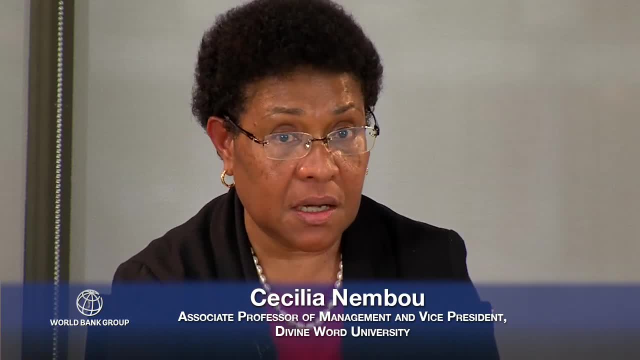 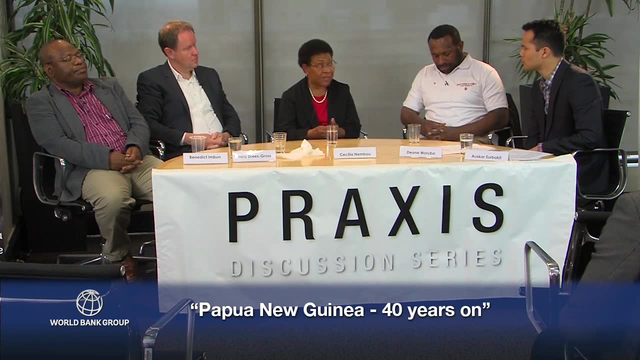 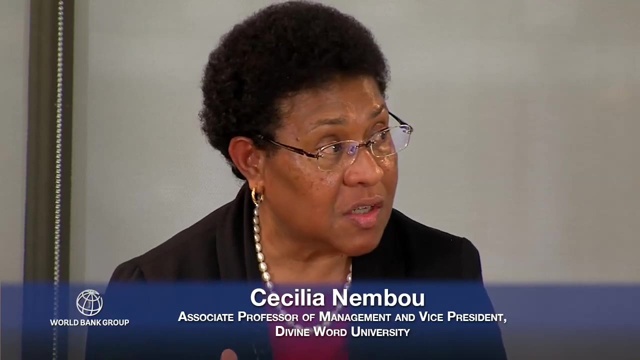 New Guineans are not marketable internationally is really a big issue for debate. The advocates who say things are fair now is because we have now a single line base, but then it is differentiated by this domestic market allowance and international market allowance, which 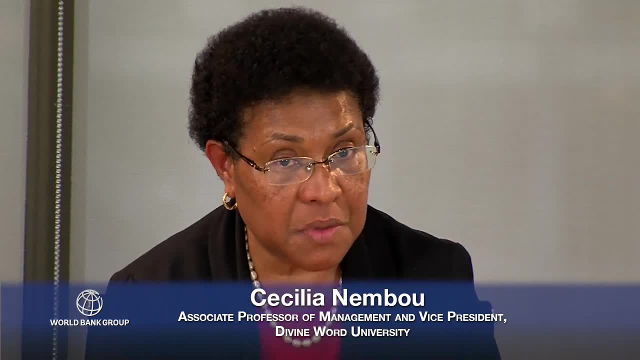 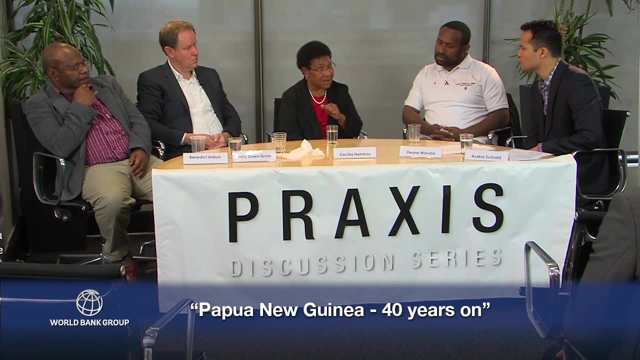 then brings back the whole thing. It tries to disguise it, but if you understand our salary structure, it's not fair at all. So that's why a lot of Papua New Guineans are dissatisfied about that. That's why they go overseas. Our academics are leaving the universities. 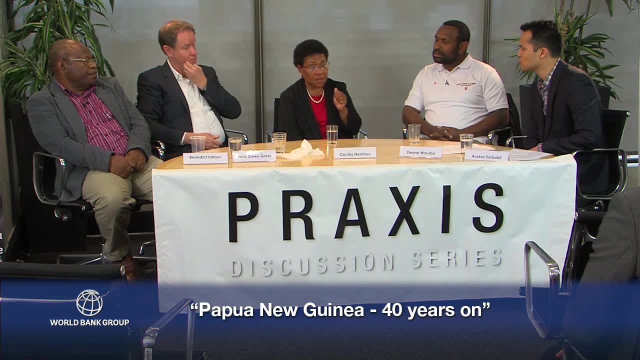 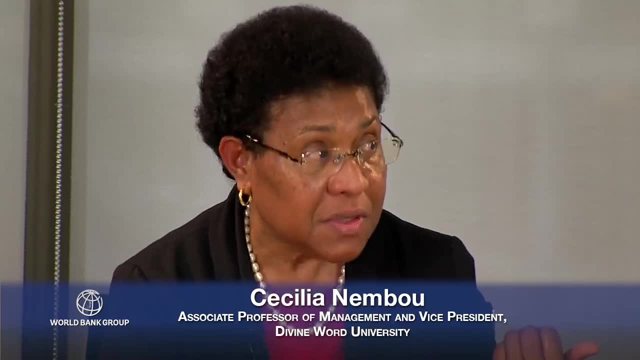 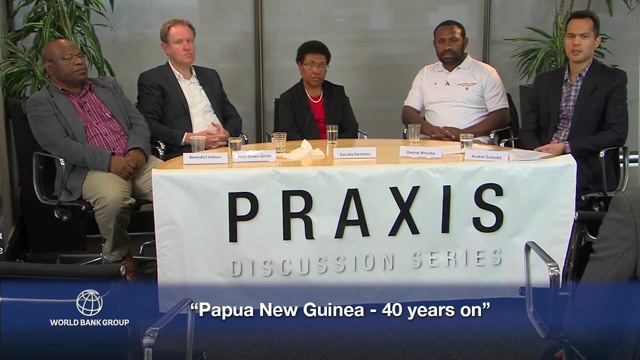 and now it is a big struggle to actually to have people teach at the universities because the salaries are not good at the universities So they're going into private enterprise where they can actually get a higher salary. So there's all that worries. That sounds like a big challenge. Do we have another question in Sydney, Sir? 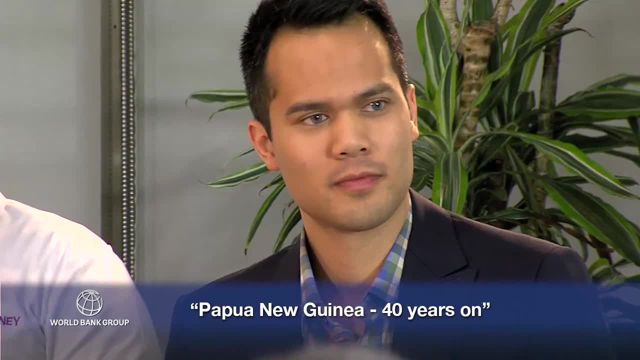 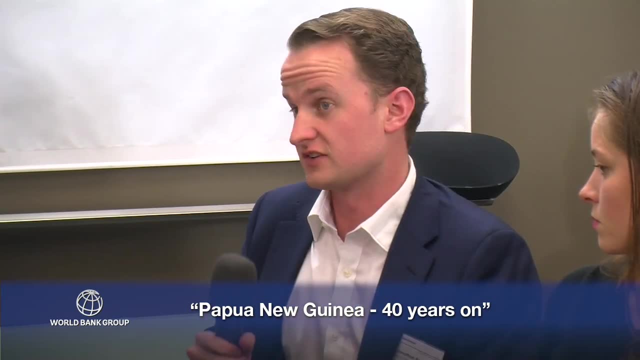 Jonathan Pryke from the Lowy Institute. In the last 40 years since independence, PNG's population has slightly more than doubled, from just under 3 million to 3.5 million To just over 7 million. Best estimates have in the next 40 years PNG's population anywhere. 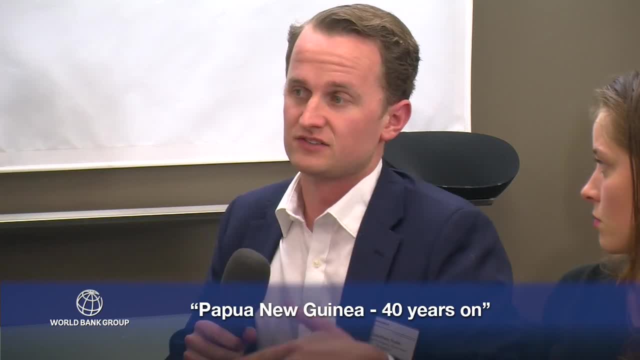 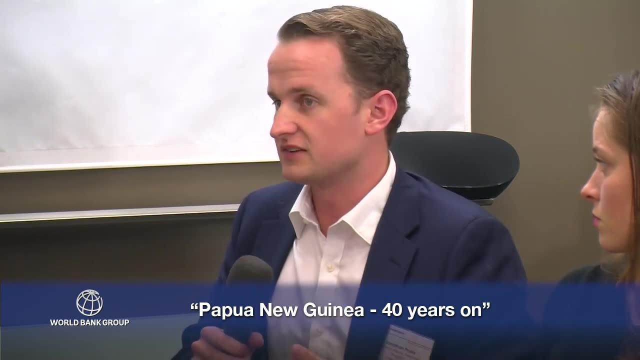 between tripling and quadrupling in size. Now, considering that the vast majority of this population increase will be happening in rural areas, can the one-talk system survive? And if not, or even if it can survive, what reforms need to take place to increase the 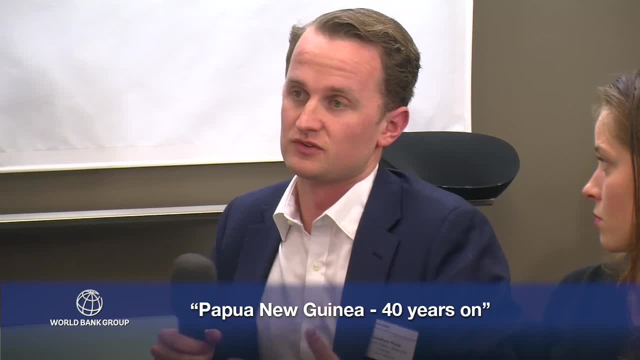 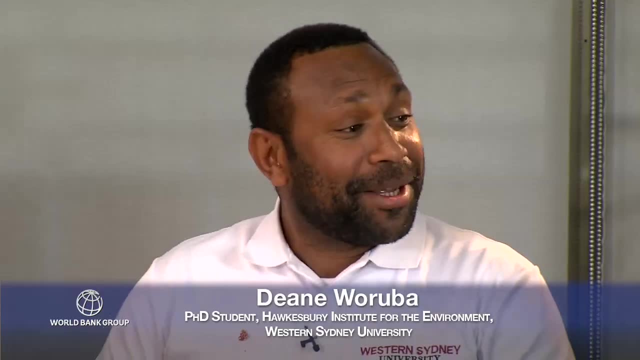 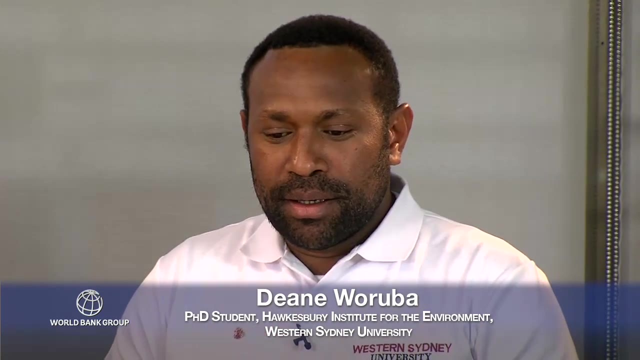 agricultural productivity to allow the system to remain intact with this population growth. Thank you, Dean. would you like to answer that? Yes, I could. I'll try. Very nice question. Yes, so that is a big challenge for us moving forward, And I sort 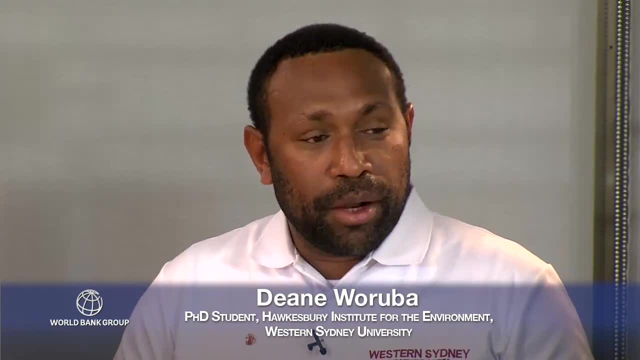 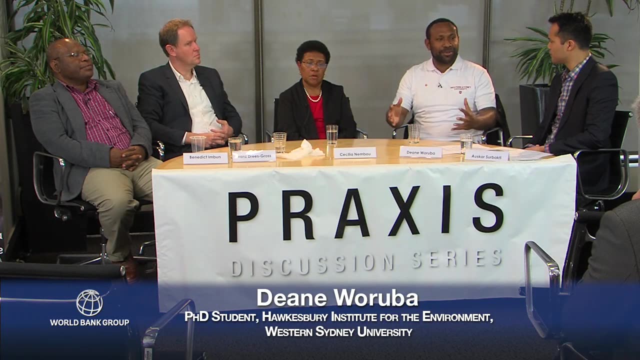 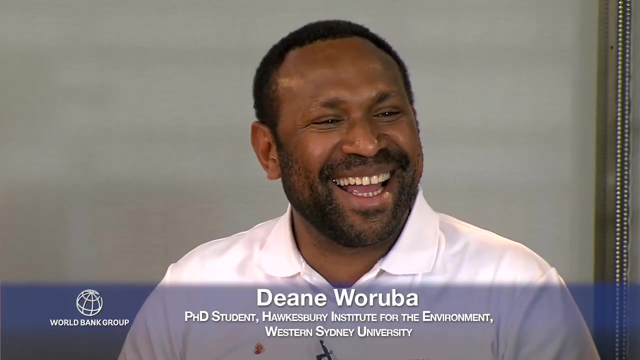 of touched it briefly. I'll say that again, That our agriculture needs to evolve now to appreciate that the basket that we're trying to feed is a lot bigger than what it is. The one-talk system will still evolve. I'm your one-talk And we can start from there. It. 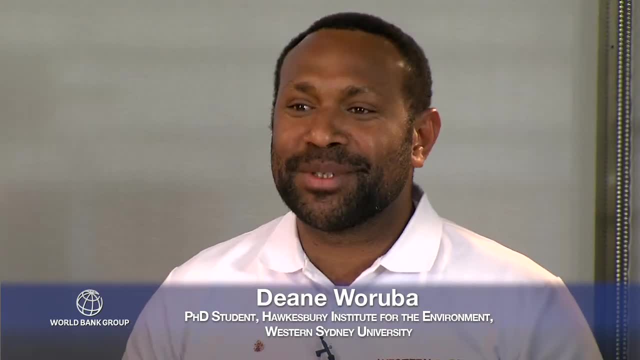 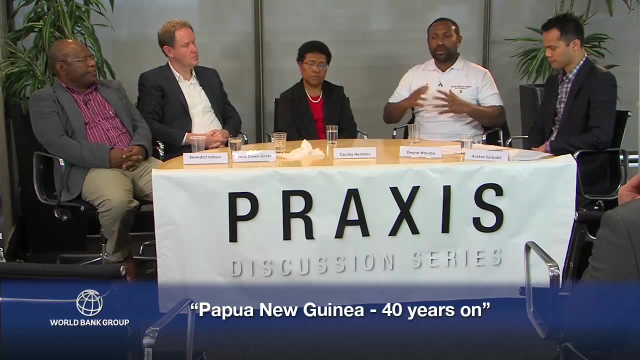 is now not people that are Speaking the same language, which is the traditional meaning of one-talk, because they talk the same language, the one language to people that they know, And communication and social media and everything else that is coming out is putting people together, in touch with each. 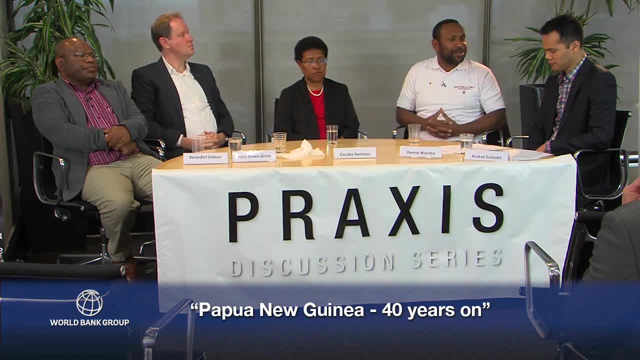 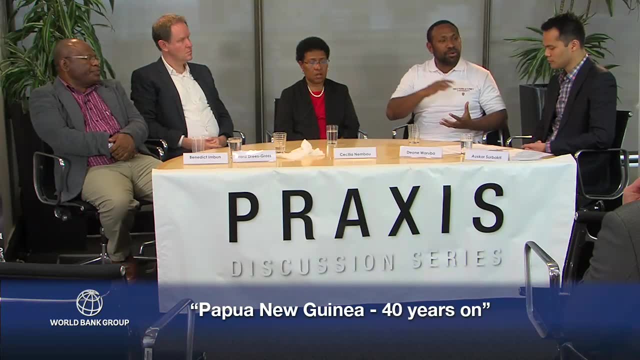 other, more People with common ideals are now one-talks, Now getting them out of poverty using- Oh, not poverty, but impoverishment, or whatever you want to call it. moving forward with agriculture is sort of. I tried explaining. 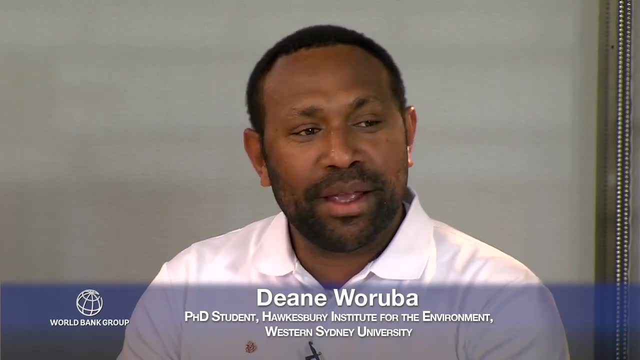 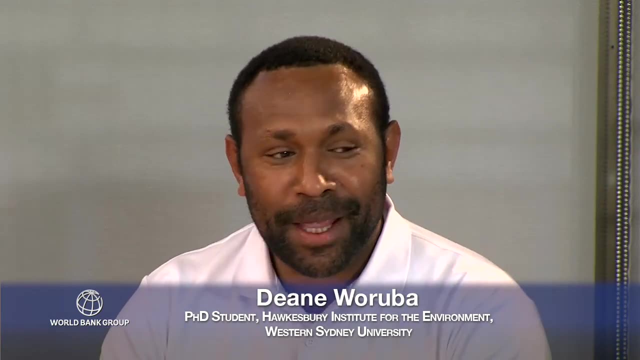 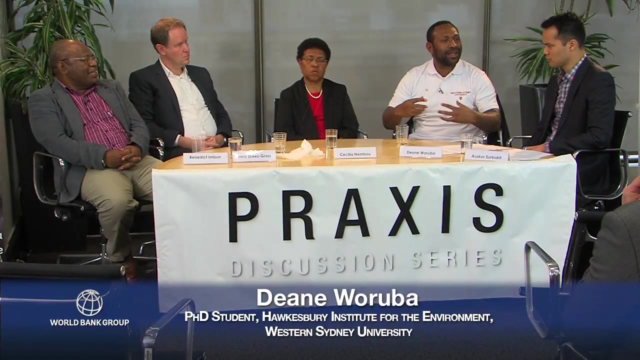 Maybe I'll try to put it this way: What we have here, what we're getting from the extractive industry sector, we're poor, We share this and we'll all be equally poor. We need to get something else in. We need to stimulate our own economy for growth to. 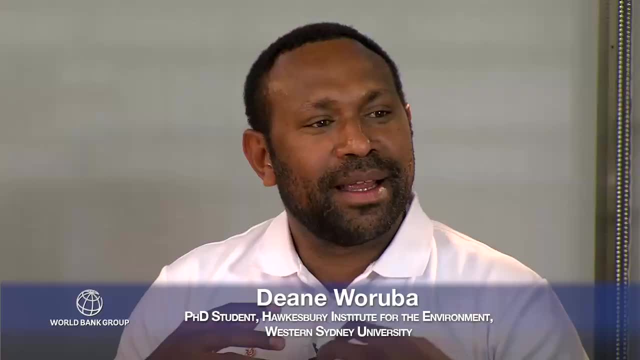 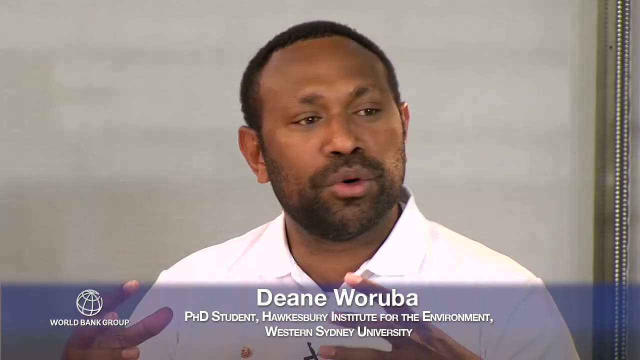 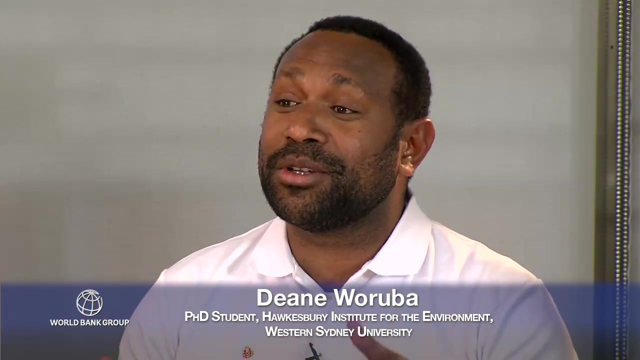 empower people to achieve more, And that is through things like our agriculture and agriculture business lease. This will engage our rural population more- 85% of the people. Now 3% of the land in Papua New Guinea is owned by the government. The rest is traditionally. 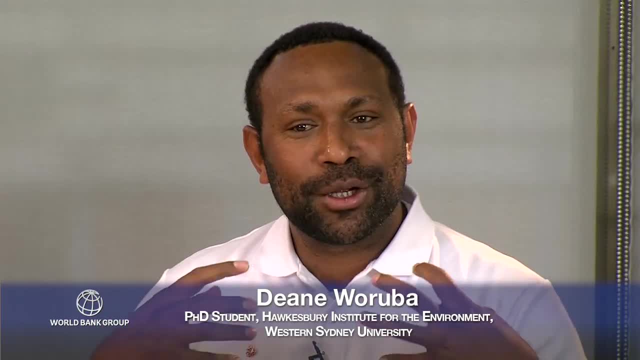 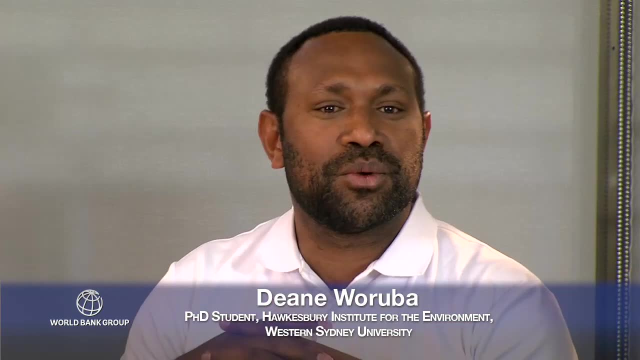 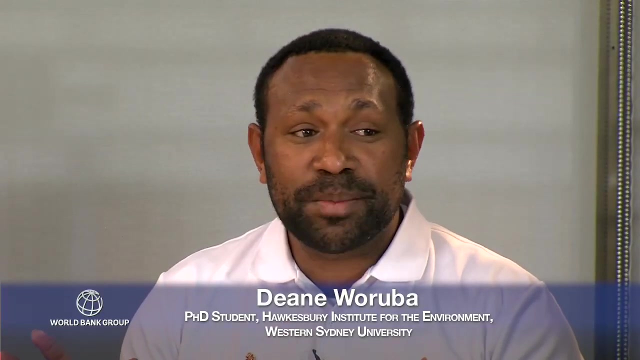 owned. We need to get people to understand the concept of immobilizing land, to be better participants and beneficiaries of this resource that is their land. The concept of the special agriculture business lease: it's a great concept. I don't think it has been understood clearly. 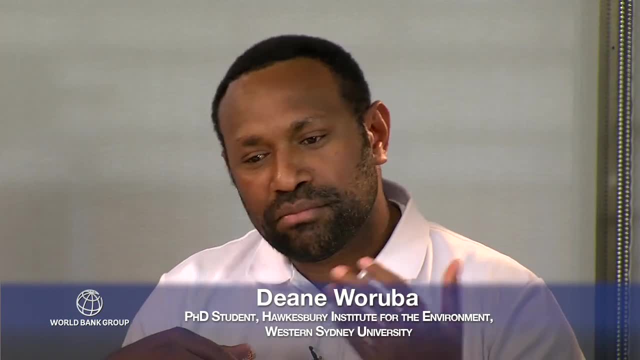 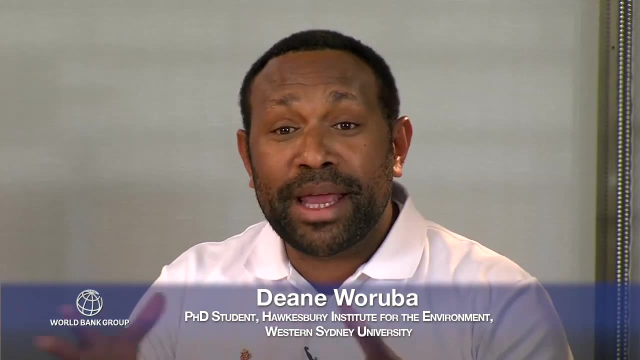 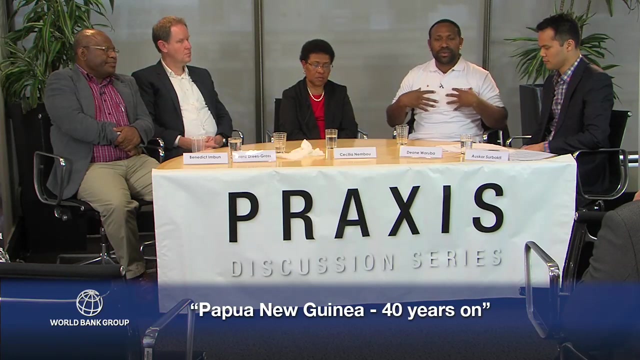 and definitely has been um abused- thank you, abused by people that understand that system and they're using it for other things. if we can manage that, it can easily work and the rural population get a better benefit and the investor comes in with a lot more confidence because we've got land. it's. 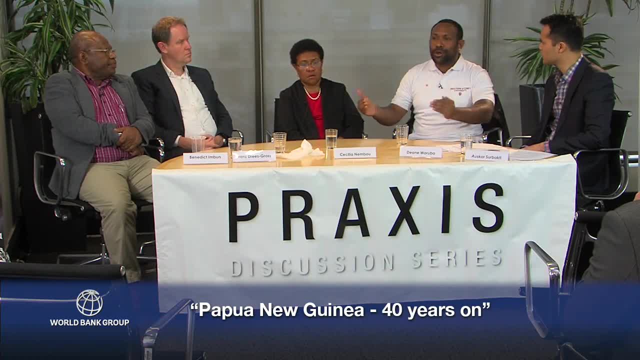 being unleashed to us for a really long period. there's not going to be travel issues and people taking that land away. we can invest more, create more jobs in the rural economy, get more more of those youths involved. the country will grow, but we have to get them to understand all these. 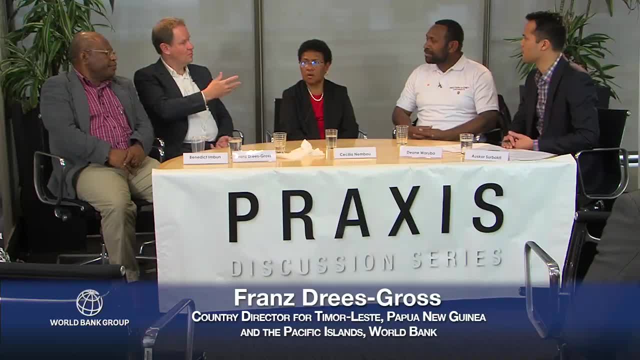 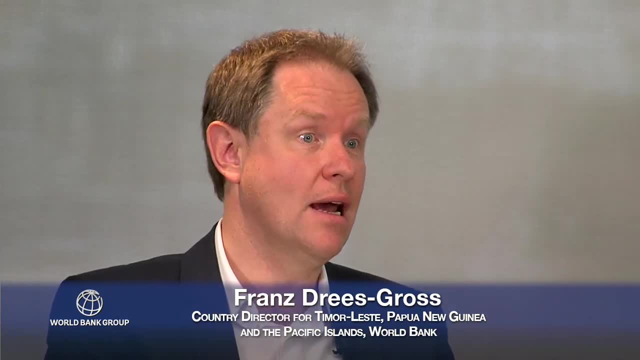 concepts. that's where education comes back in, friends. i could just build on what dean was saying, just in answer to the question. i mean, there are approaches to increasing agricultural yields that work and they work right now in png, i'm happy to say the government has a program. 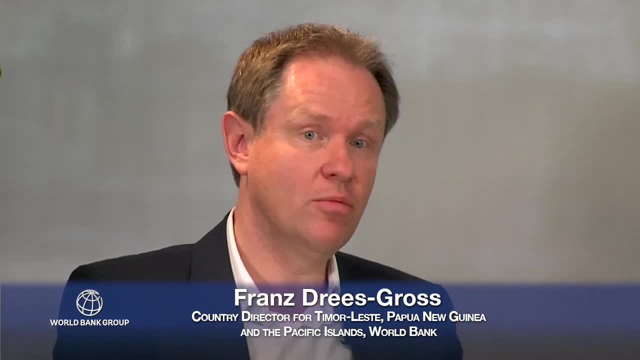 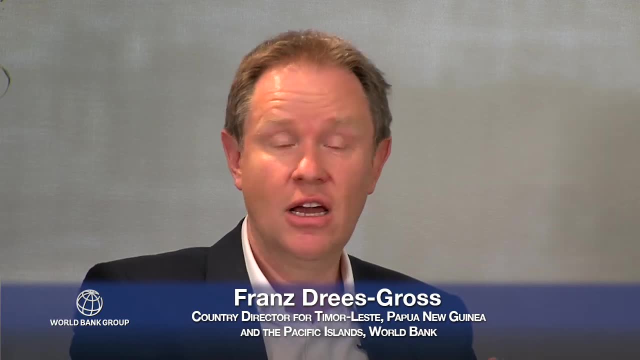 called productive partnerships for agriculture, and we're very proud to be supporting that as the world bank. the basic idea is this: you bring together farmers groups with extension agents- a lot of times with bonds, buyers of whatever those farmers are going to produce downstream, and you basically have 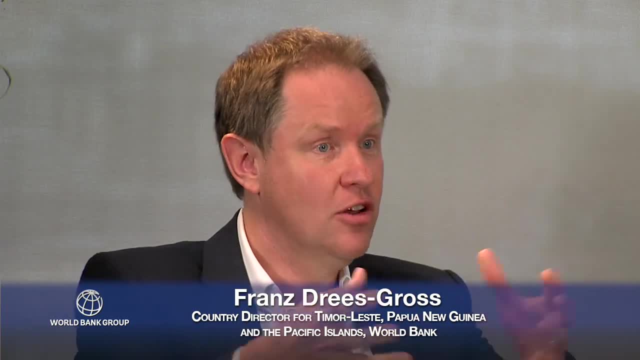 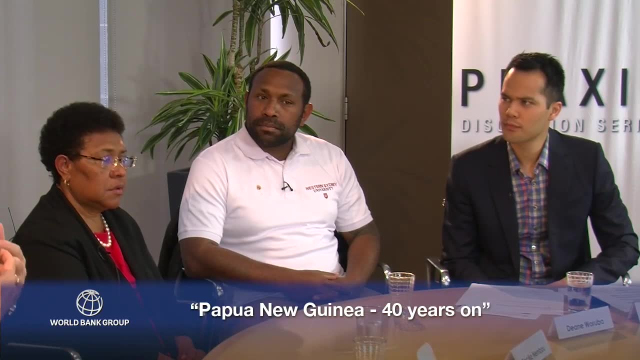 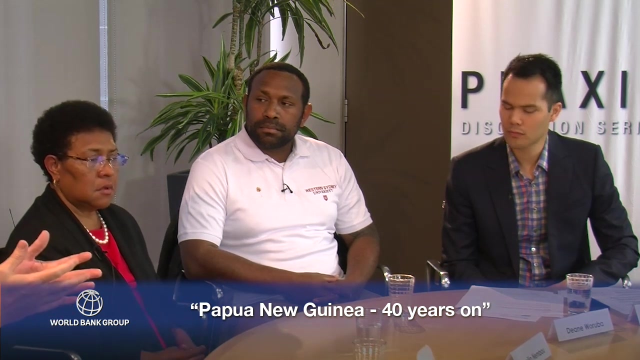 them put forward a proposal, but not just a proposal by any one party, but sort of an integrated proposal of the buyers, the producers, the extension agents, et cetera. And then government uses grants to basically invest in that group. So, for example, make available a grant to them to cultivate new seedlings for cocoa. 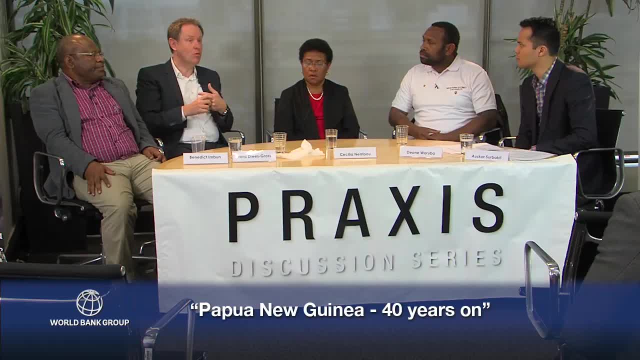 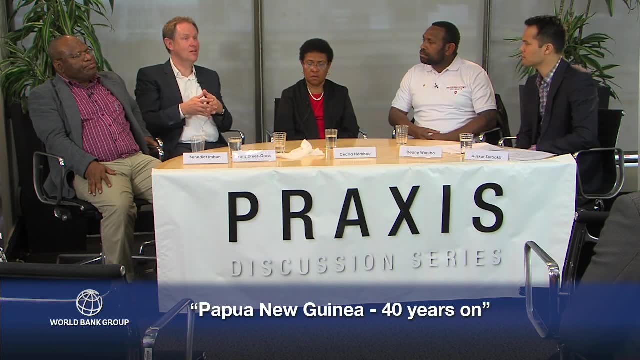 or coffee, or graft new trees, et cetera. That works. There's several tens of thousands of farmers in P&G that are being supported under these grants. The problem is in rural areas. as we've heard, it's 85% of P&G's population. 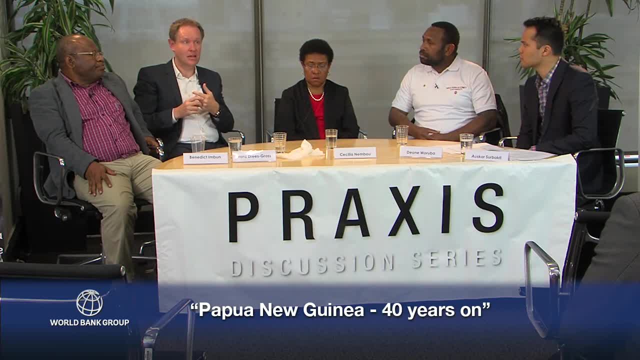 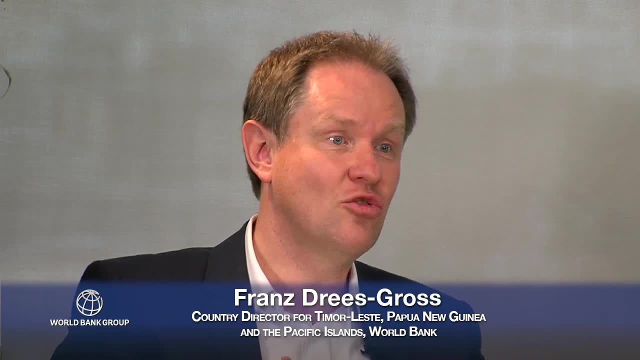 So you need to take that up an order of magnitude to be at real scale. But there are approaches that are working right now and even if you have a tripling or a quadrupling of the population, this is an extremely fertile country in many parts. 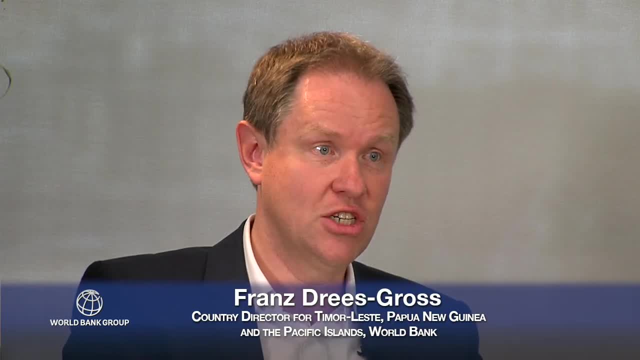 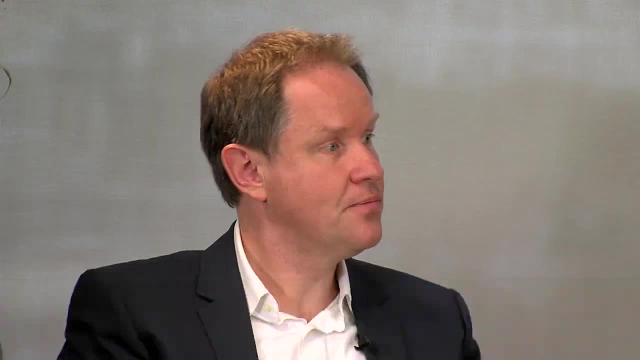 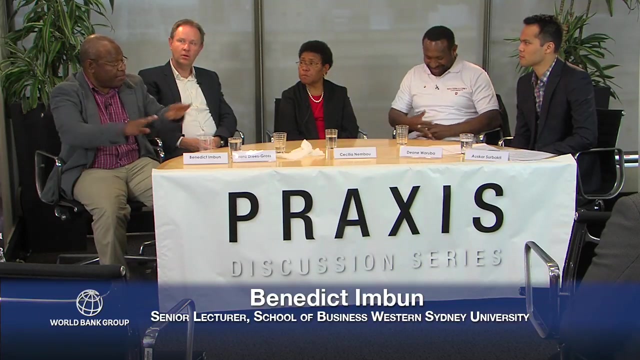 It's very sparsely populated even if you triple or quadruple the population. So the productive potential is there. I think it's really just a matter of Of unleashing it and it can be done. Right, Yeah, If I can just shed some light on the stubbornness of the subsistence farmers to extend their 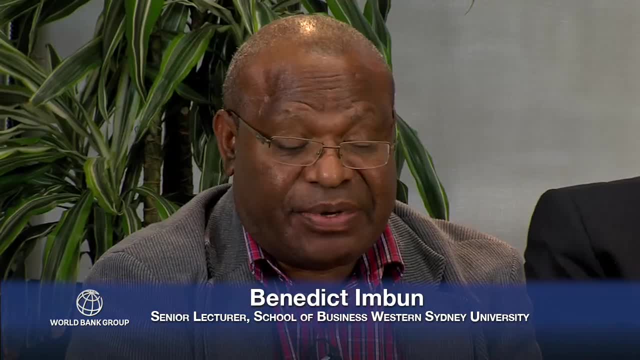 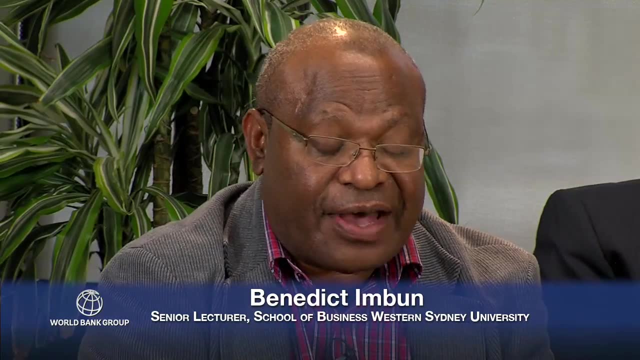 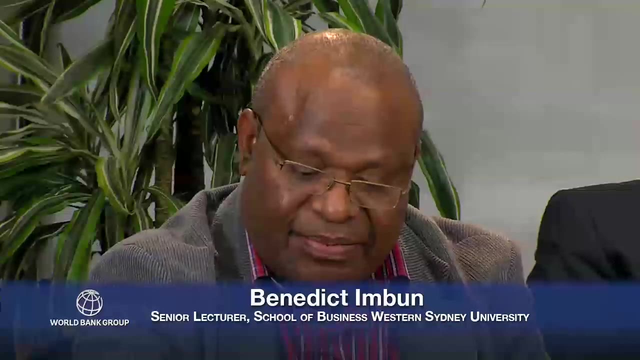 land or to make it more economical is simply because I mean it's tribal land or it's communal land or it's family land. So somebody, or the father who actually owns a plot of land on which the coffee trees are grown, cannot extend it and enlarge it on its own. 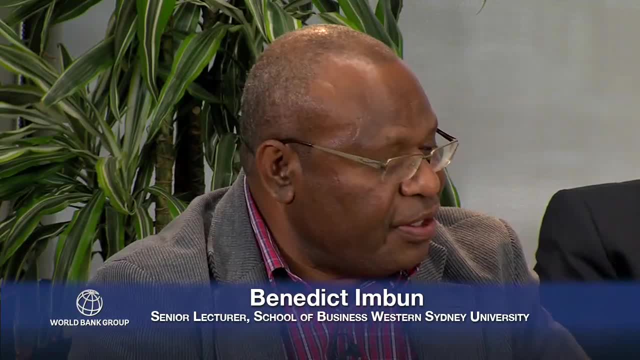 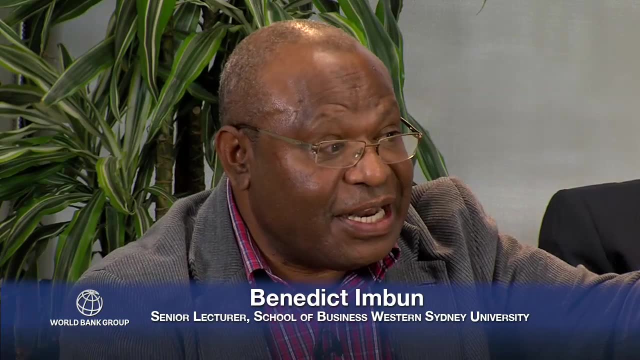 Right And can't use it on the basis of a coffee prices because he needs to consider the family members. They're probably five sons or three sons and they would be getting married and obviously they would settle on the land. So those things are really playing a huge part. 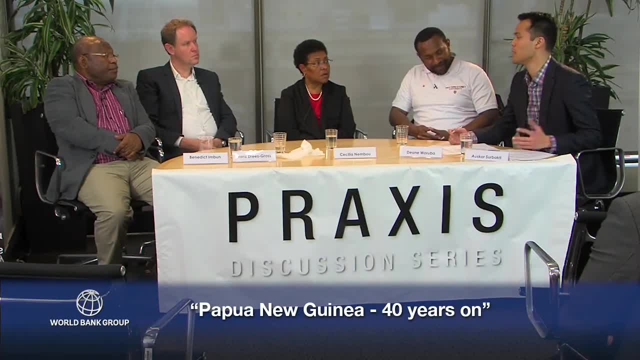 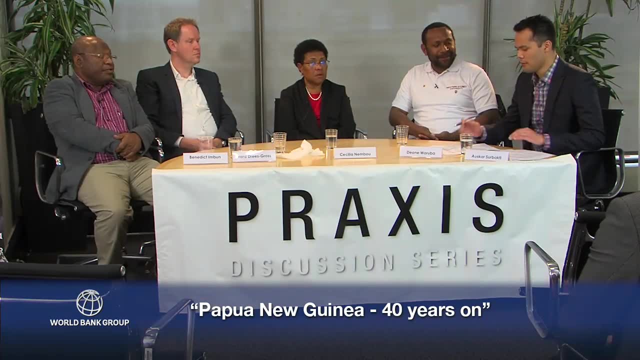 So the divide between cultural imperatives, traditional imperatives, That's right. That's where the challenge is. The macroeconomic Trying to make sense, Yeah, Interesting. Can we go to a question now from Timor Leste and this one's for Cecilia? 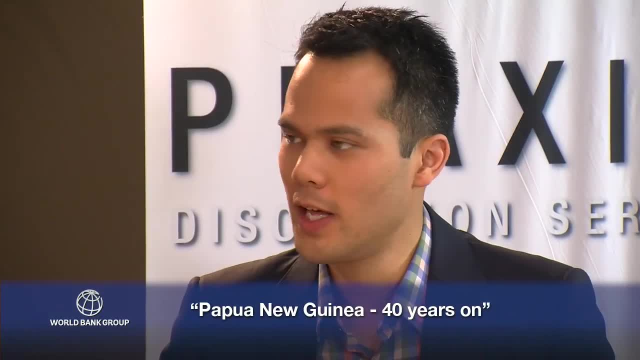 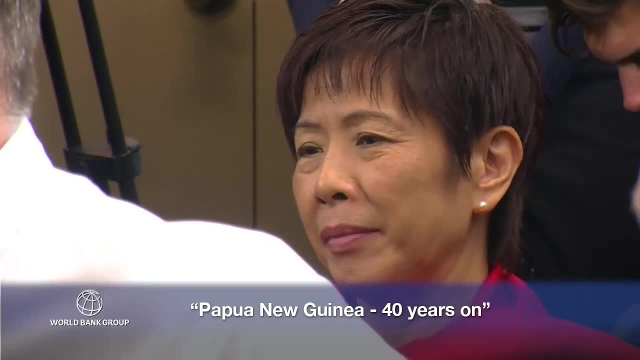 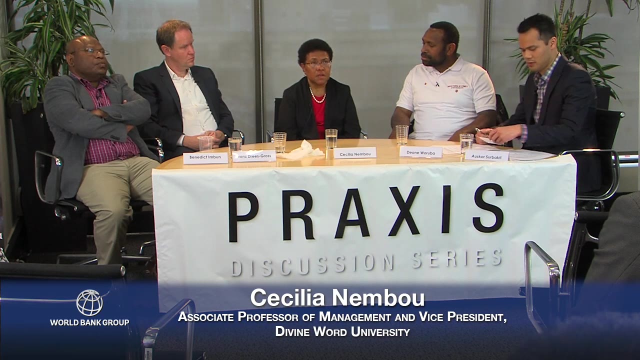 In your view, what is the biggest lesson that Papua New Guinea has learnt that can be applied to other newer countries like Timor Leste. We still have a lot of challenges, but I think for me- I mean, I always come back to this- 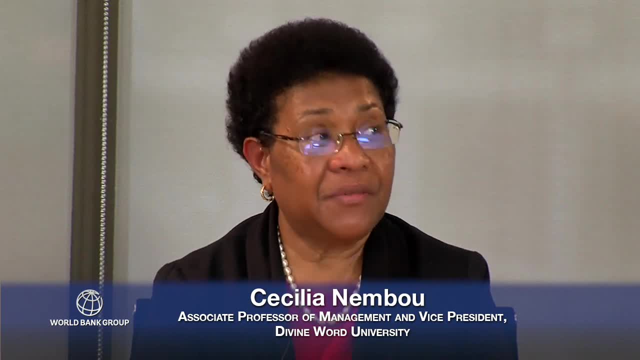 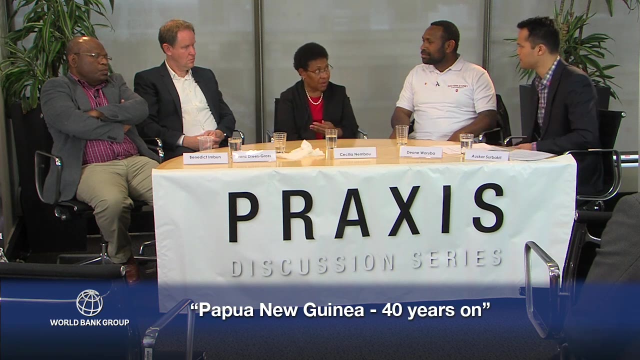 2050 vision, but the fact that we actually have a vision for the future. I mean, I'm also passionate about strategic planning, Yeah, And I think that we actually need to create our own future, And this plan is our attempt to create our own future by saying: this is where we want. 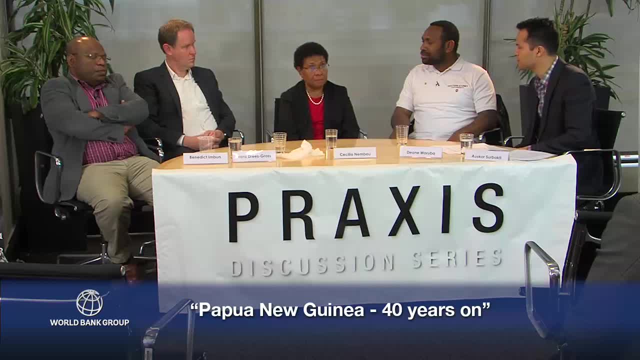 to get in 40 years' time from 2010.. How are we going to get there? These are all the things we have to address in order to get there And, I think, to actually start to plan or to envision our future and then work out what. 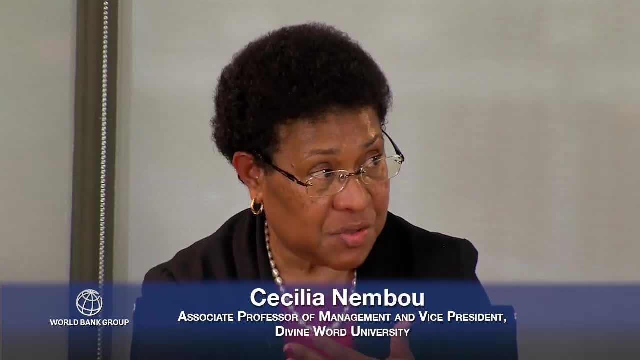 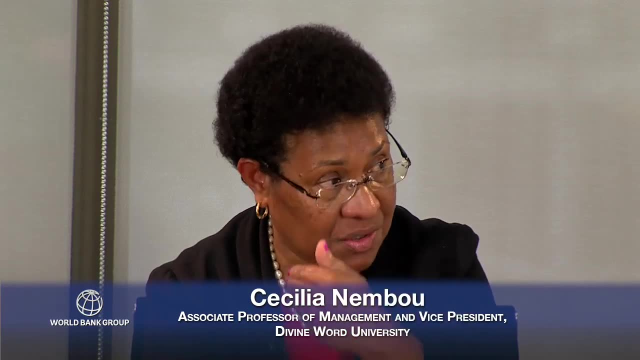 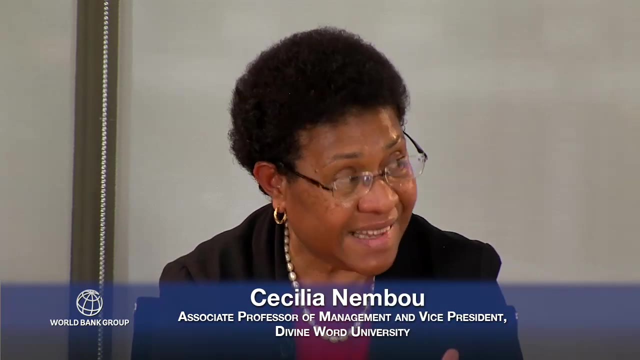 we mean by achieving that future. what does success mean? what we see in the future, that's what we think success is. So we need to work on that success achievement in the future. I think the idea of strategic planning and thinking is a lesson that I would like to. 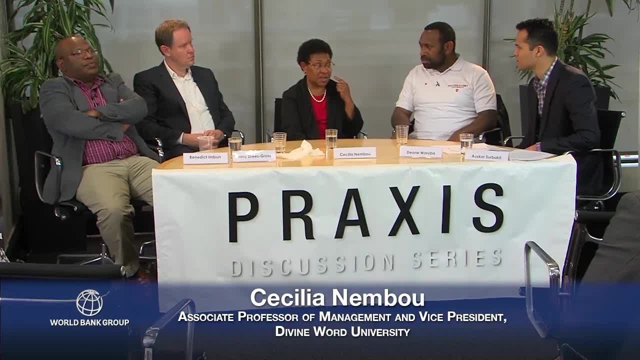 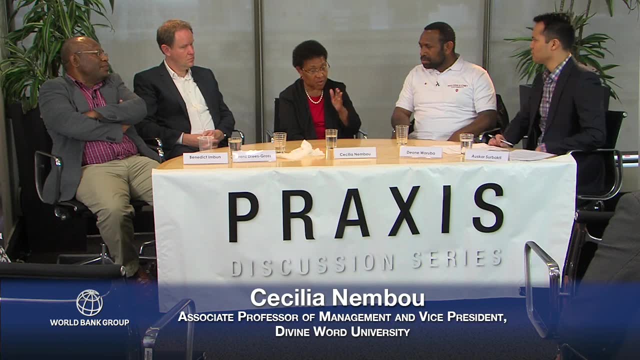 actually recommend to other smaller nations to think strategically, to know what you want and then work hard. So it actually is working hard Right now, PNG. I'm not sure whether we actually know what it means to work hard, but in order. 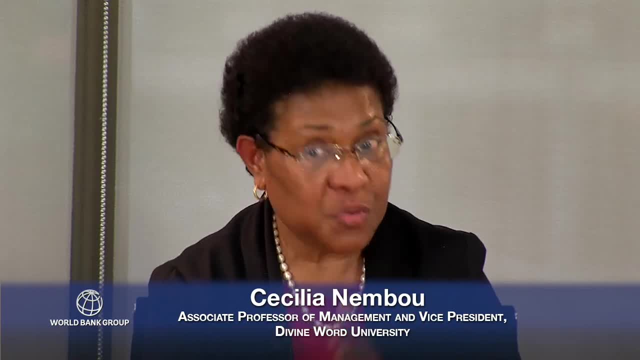 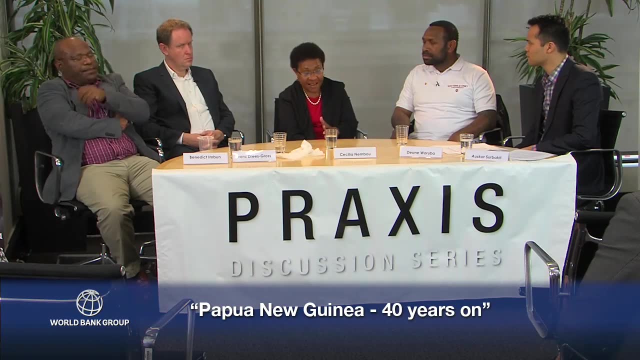 for us to actually achieve our vision, we must work hard. We have to work hard. We have to work hard To be happy and fair and smart, we must work hard, And so there is an element there that we don't mention very often is working hard. 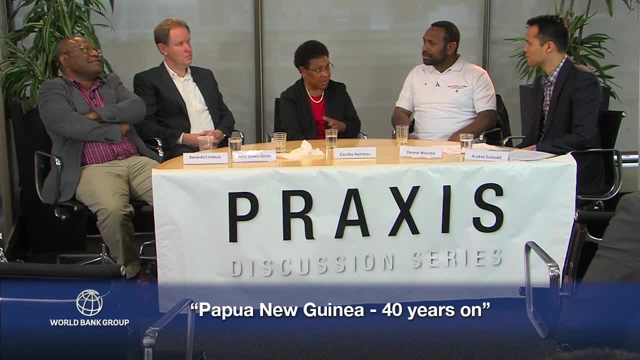 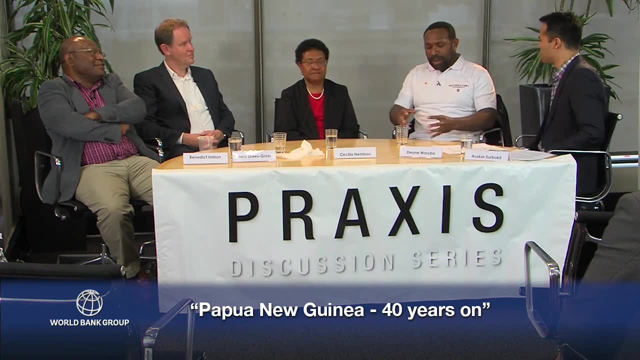 So we're going to teach ourselves how to work hard and teach the younger people how to work hard, and I recommend to the other smaller nations to also teach their people to work hard. Excellent Heading on appreciating Vision 2050. again, that's a long-term goal for the 40 years. We also have a medium-term development plan, which is every five years, So it puts us to try to achieve those goals, and then, of course, the short-term plan, which is every year. By the end of this year we try to achieve this. it'll fit into our five years and eventually, 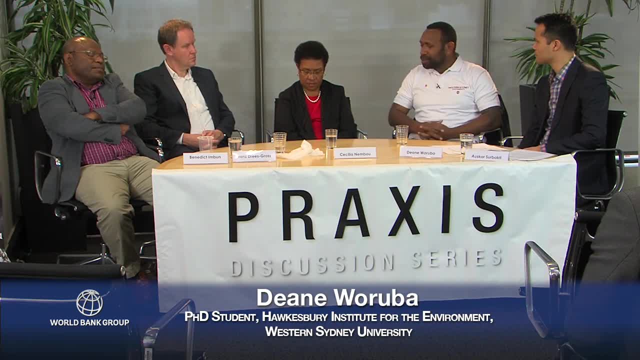 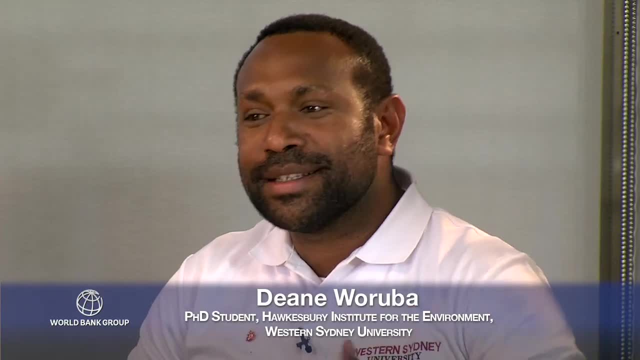 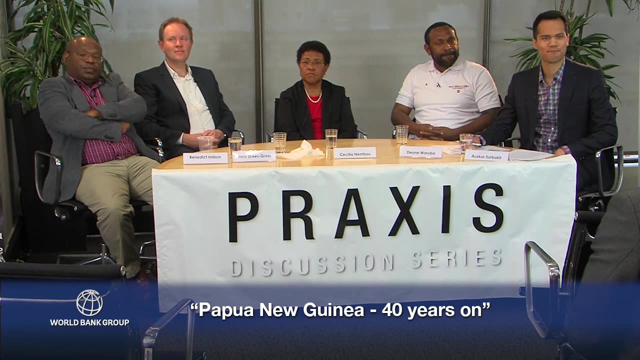 our bigger plan. So I think moving on from advice to our friends in Timor-Leste is having a plan like that, but also putting in monitoring and evaluation indicators in between to see where you're going all along. Sound advice, Okay. Is there another question from Sydney? 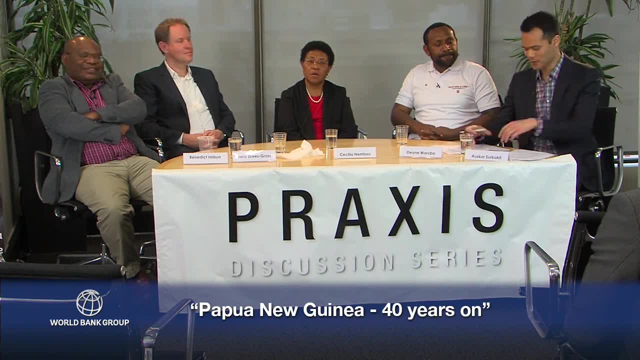 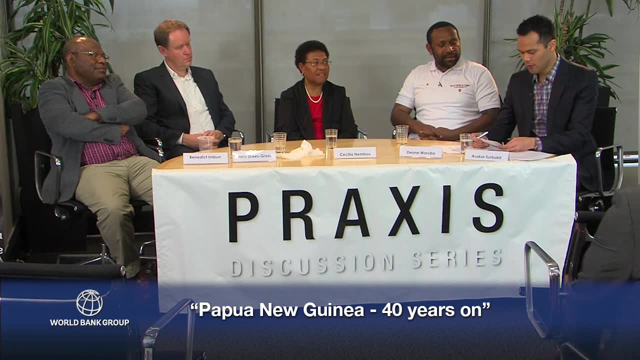 No, Thank you. No, That's okay Because we've got many from overseas. We've probably got time for a couple more. So there's another question here from Port Moresby. This is open to anyone in the panel, but we might just get one person to answer it. 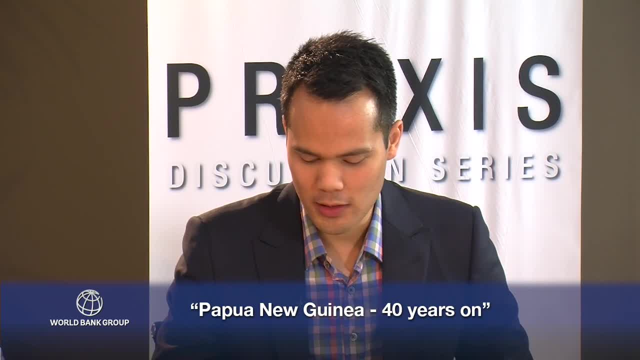 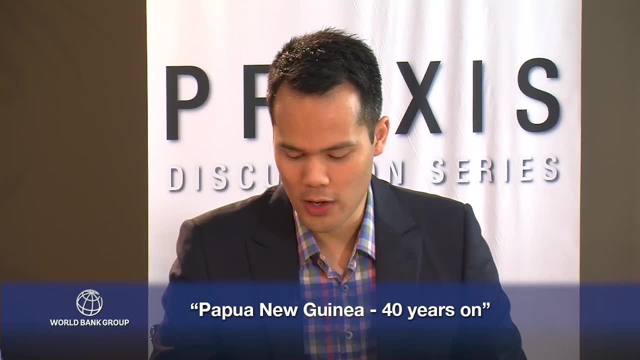 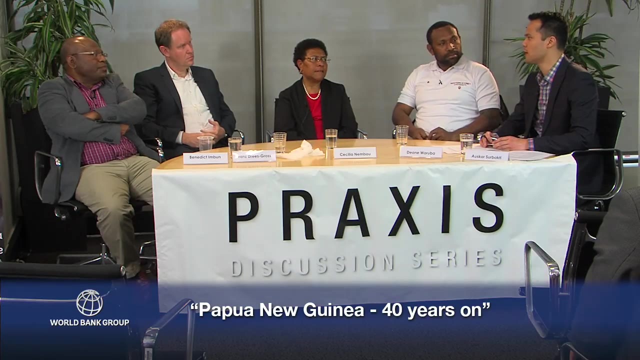 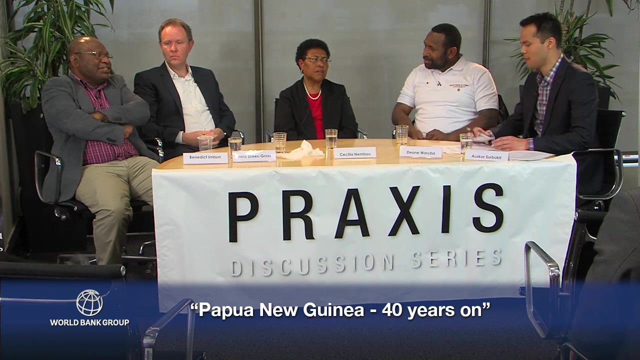 So development partners have been pouring aid into PNG to develop various sectors. Now, 40 years after independence, there's no evidence of an adequately trained workforce. Why do you think that is? I guess that's your area of expertise. So, despite the development agencies and the aid that PNG received, is there a workforce? 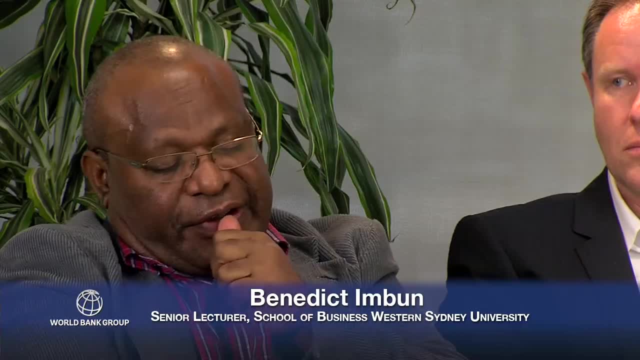 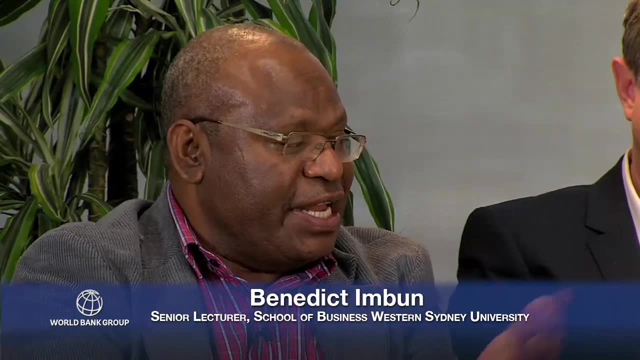 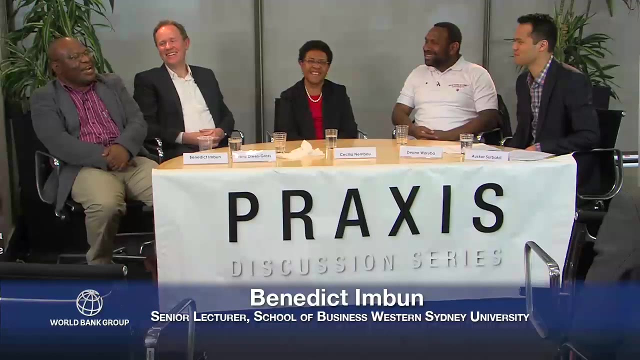 to reflect that investment. Obviously, the aid donors have actually come in a big way and they continue to support us: Australia Aid, European Union, World Bank- I'm not sure you guys are donors. Yeah, Yeah, Yeah, There is a place for them. 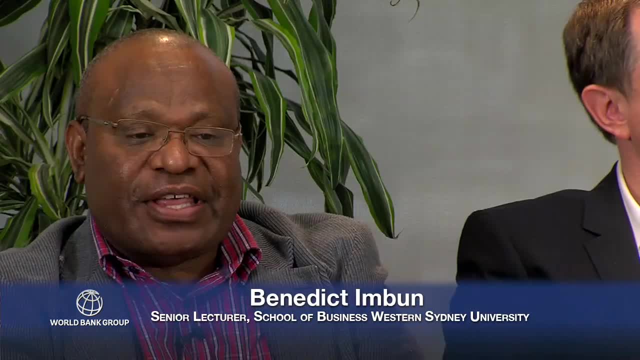 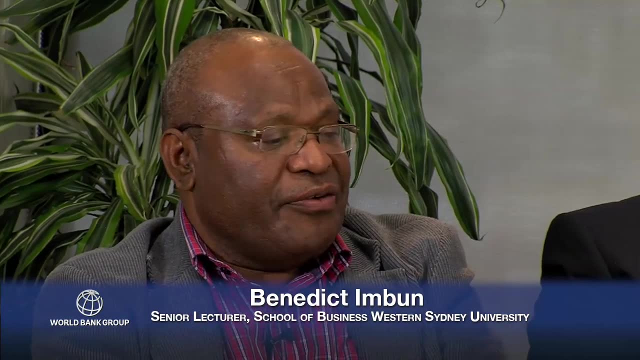 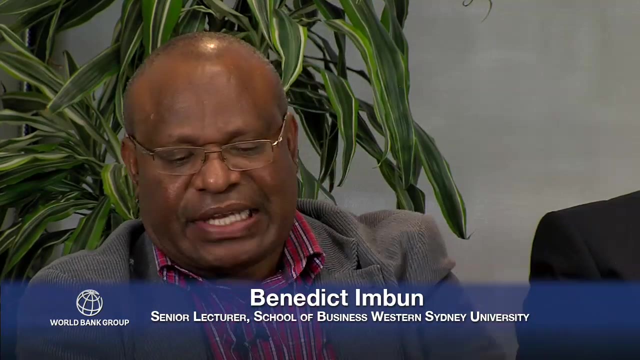 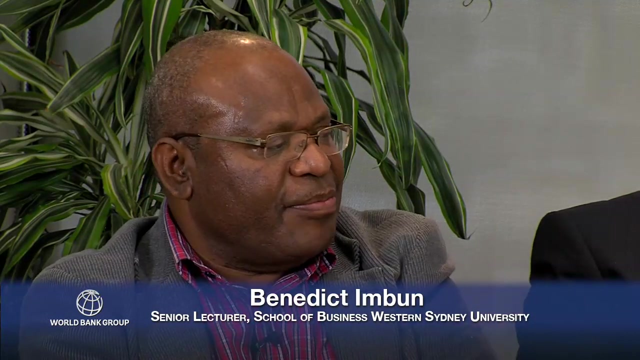 I mean the Vision 250, we cannot achieve without donors, So they continue to relieve the PNG government of its major responsibilities. Having said that, there's been a lot of criticisms on their donors as well, of bringing in consultants, and a third or fifth of the expenses are paid on them. 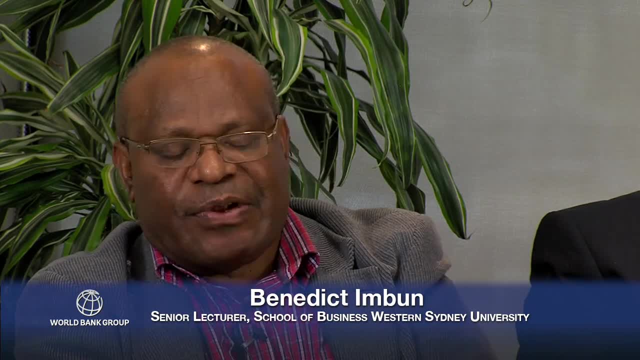 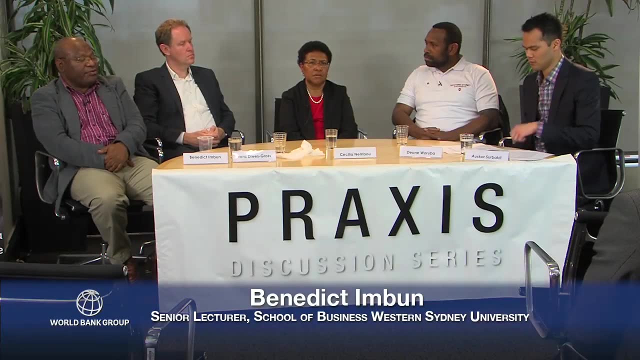 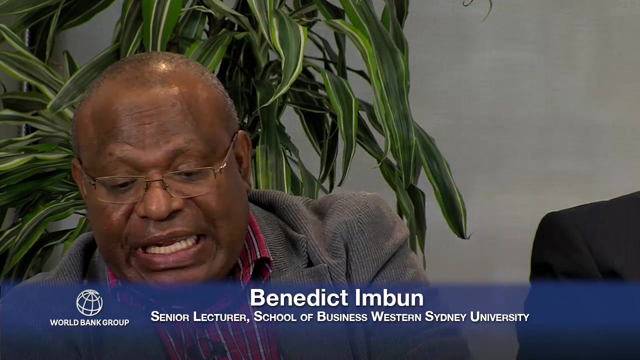 And those things go on, But we cannot develop the country without them. So obviously they are absolutely necessary to partner the PNG government in achieving those goals. But yeah, their contribution has been tremendous When the government has failed in terms of providing markets for women and children to 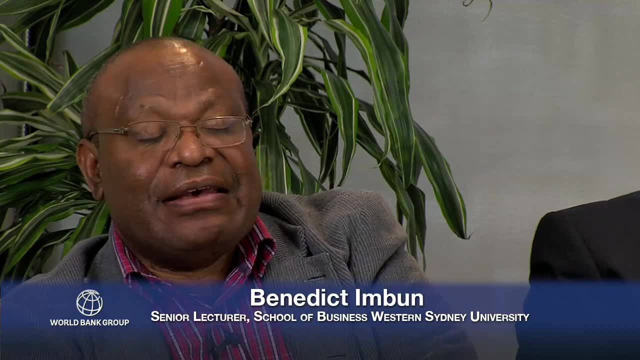 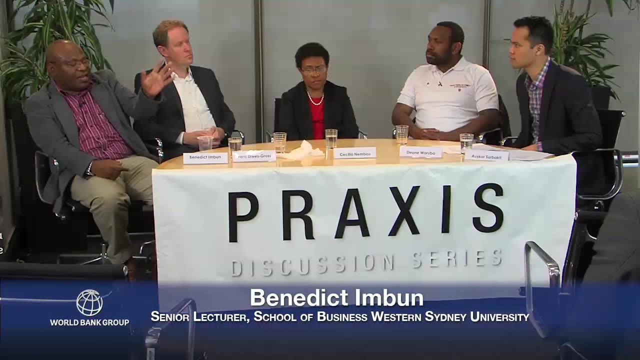 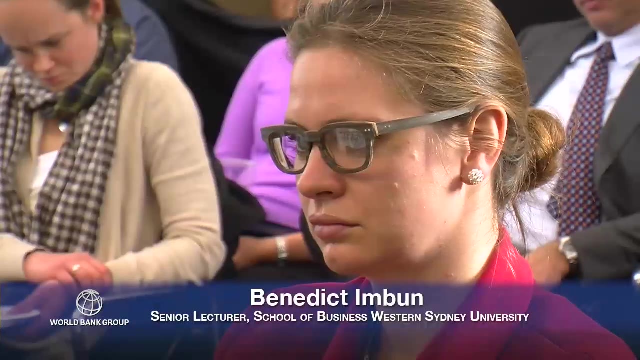 sell their produce- those of you who have been to Mount Argonne. there's a big market in Australia. They're the biggest in the country, I mean, put up by Australian aid. So the PNG government concentrates on other bigger things And these are things where, in terms of funding the HIV and AIDS programs, the donors have 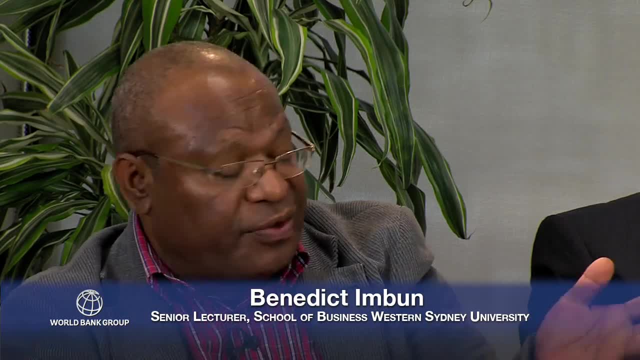 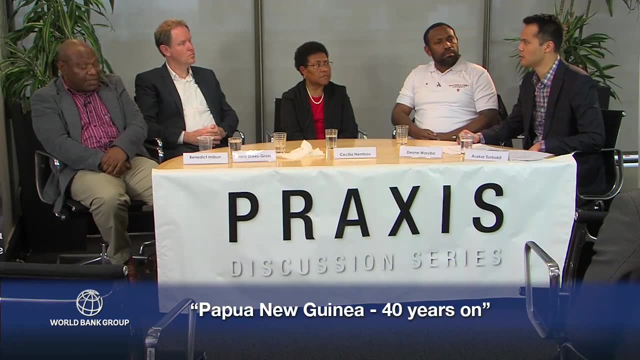 actually come in a big way, And if it wasn't for them, obviously we wouldn't progress the way we have. So there's still very much room for development partners and donors. That's right. Yeah, A big room, Bigger room. 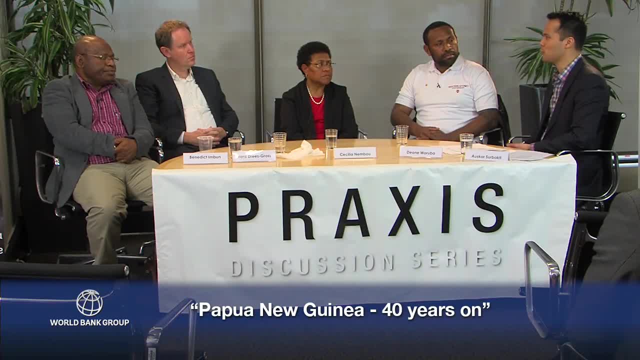 Bigger room. Can I just ask each of you briefly what's your outlook for Papua New Guinea? Is it a good one, a bad one, in between? Can I start with you, Dean? Thank you, Obviously it's going to be a good one. 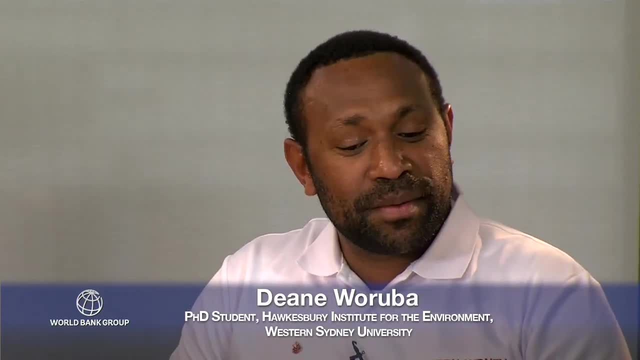 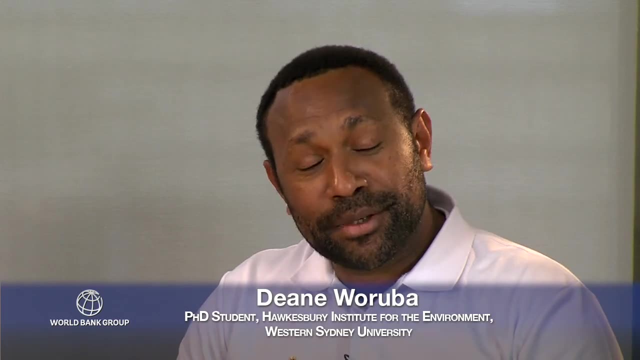 I'm excited to be part of it. I see a lot of positives. Obviously there have been negatives, but that only means that we have a lot of room for improvement. I really believe the best is yet to come, Cecilia, Yeah. 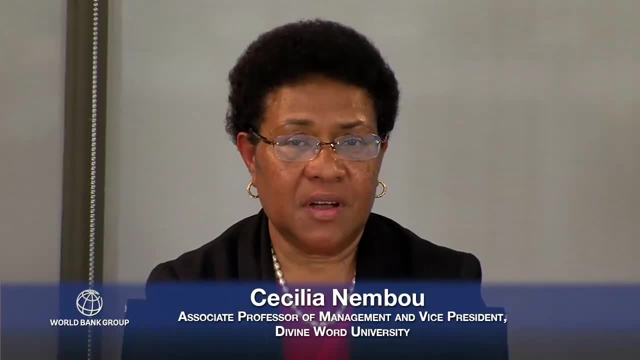 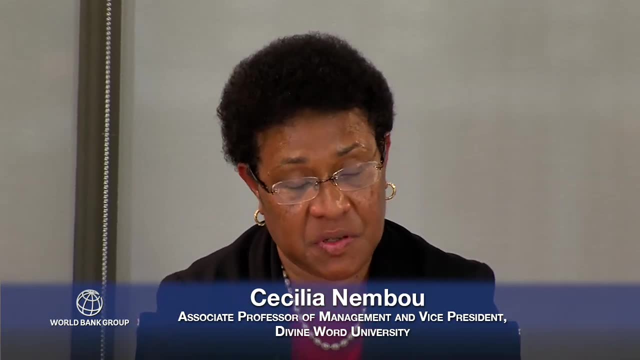 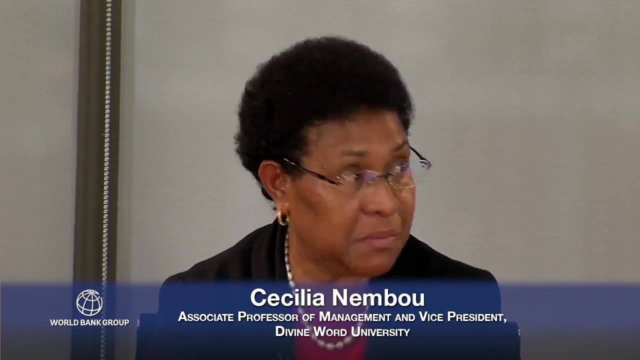 I am very positive about the future of PNG. Yeah, I believe that we have already started, but I believe that we will be the leader in the Pacific region just by the mere fact that we are big. We have more people, We have more challenges, but we are able to overcome our challenges. 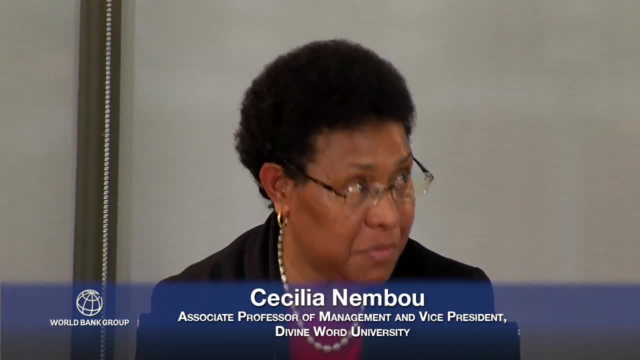 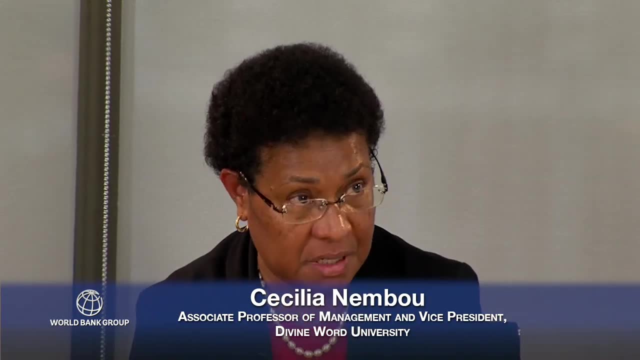 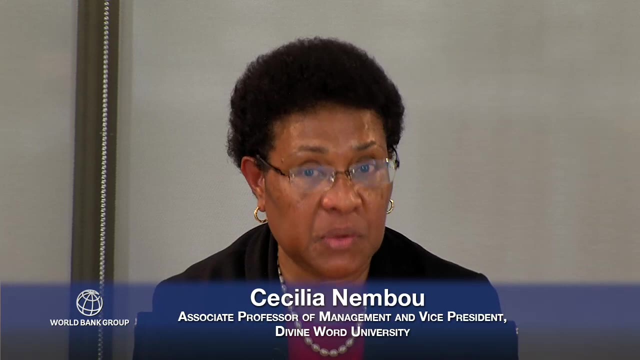 We can teach the smaller nations a thing or two about development issues, But we have a bright future. We have resources. We have our people. We have more than 7 million people and growing. If we can educate all of them, Papua New Guinea has a bright future ahead and we will be. 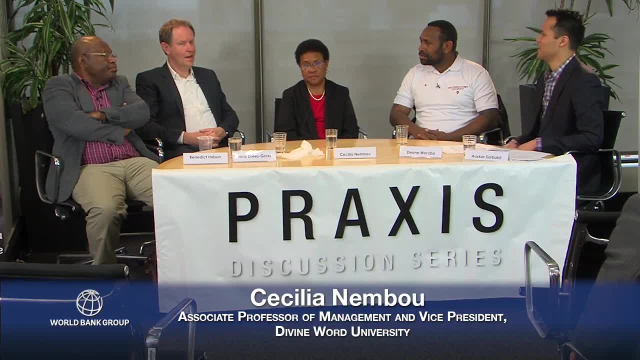 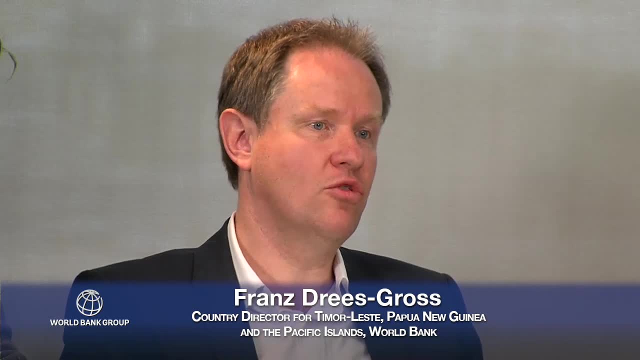 the leader in the Pacific region, Brent, I think Papua New Guinea is perched on the edge of an opportunity. I think for the next 40 years Papua New Guinea could, if it plays its cards right, really take off, And I think the amounts of money that it could spend to take off aren't necessarily even. 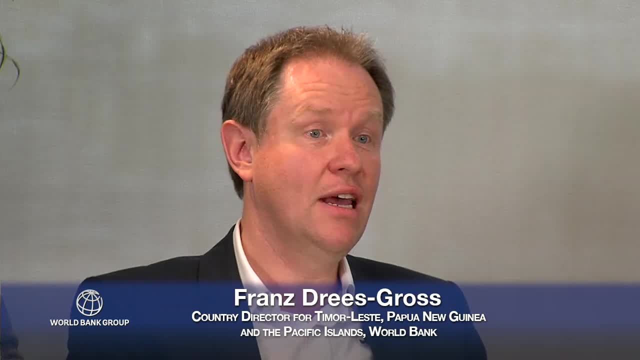 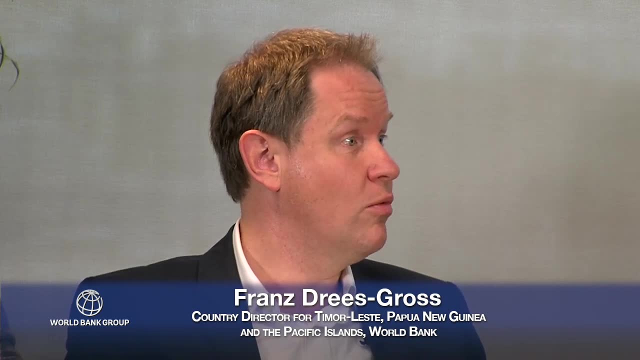 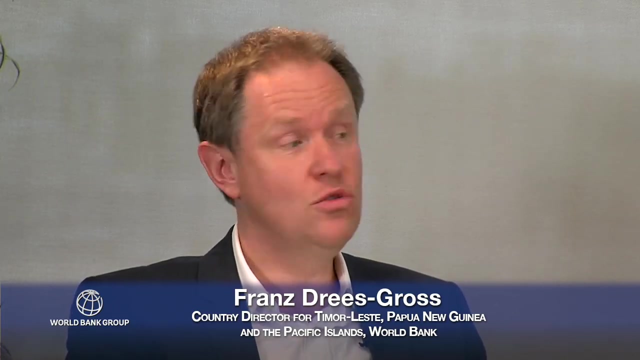 that big. Let me just give you one example Right now, if you take internet connectivity, that's something that's been a big enabler of development in many countries. It's exploded recently, but it's all basically wireless. So in 2009,, only 20% of Papua New Guineans lived in an area where they had 2G mobile. 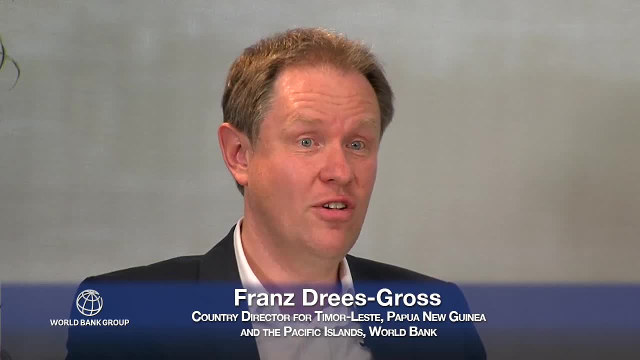 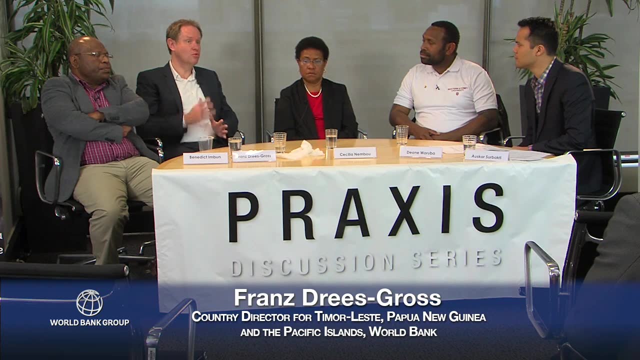 connectivity. Now it's 90%. That's six years of development. It's not 40 years, It's just the last six. The big thing is that fiber optic cables, for example, only reach Port Moresby and Madang right now for less than $100 million, which, relative to the size of the economy, isn't. really a huge amount of money. You could reattach Papua New Guinea to the world. The existing cables are aging. You could run a cable along the entire coast. You could collect Papua New Guinea, Ley, Insular, PNG, New Britain, New Ireland, et cetera. 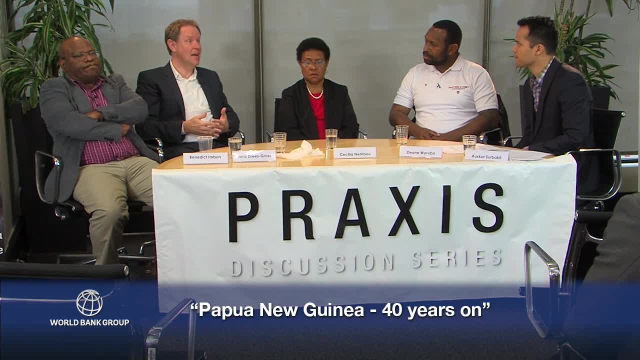 You could do it for a relatively affordable amount and get broadband cable to huge fractions of the population, And doing that would just open so many opportunities in terms of businesses that could open and market themselves on the web, educational opportunities that are suddenly available in the interior. 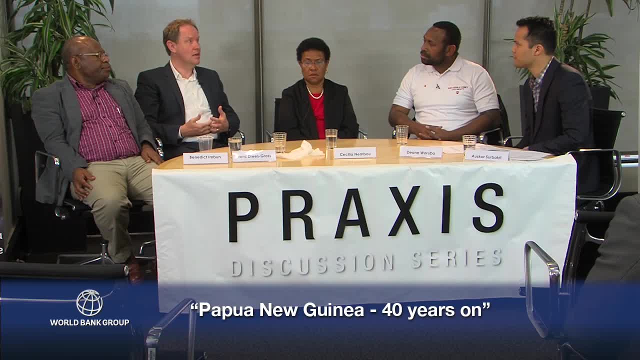 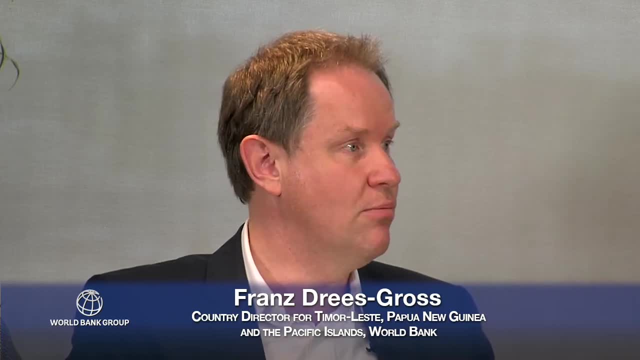 And it doesn't even take that much money. So I think you know, with good technical advice, we're happy to be part of that technical advice. There's certainly many others that can help provide it. I think PNG is really poised with great opportunities. 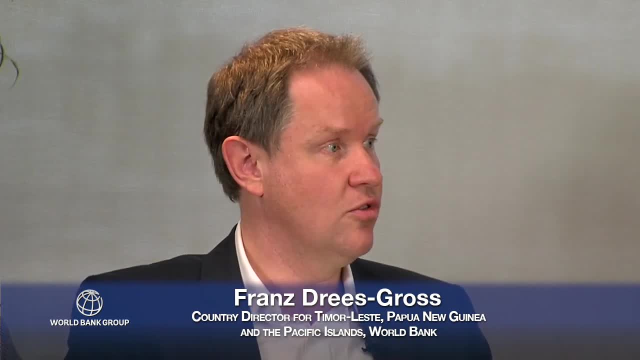 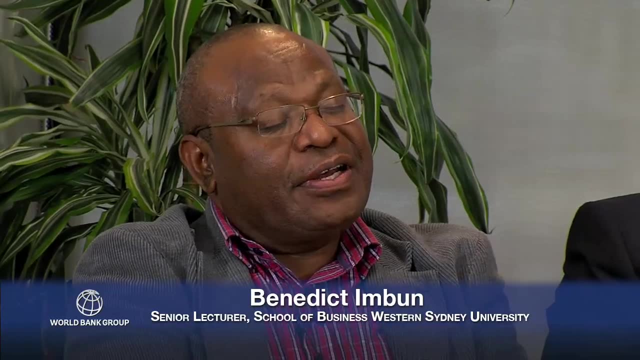 And I guess our commitment is to help them make the most of those opportunities. And, Ben, where do you see Papua New Guinea? I equally share the view of PNG having a robust, bright future, But obviously the missing link, provided that we have good leadership. 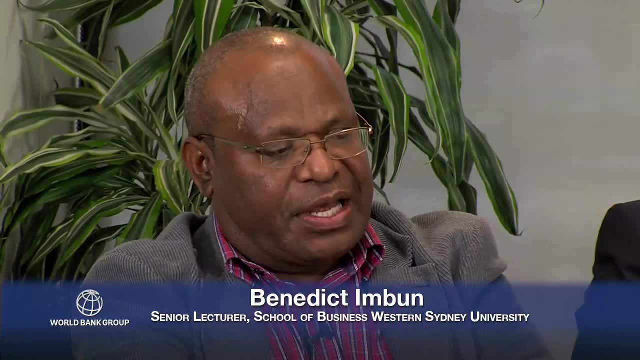 You know the development, and the development is very important And I think it's a very important thing for us. I think there is a great opportunity for many developing countries. Singapore is already a developed country now, but Malaysia and others are singularly endedly. 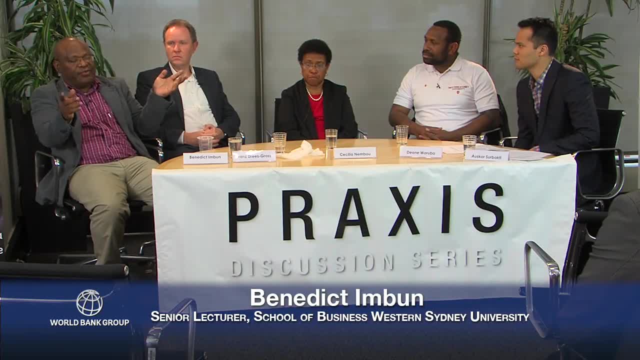 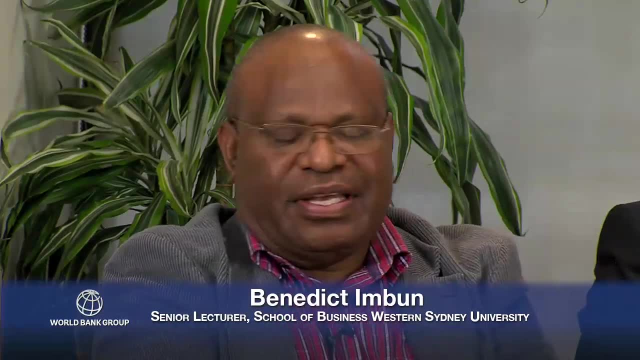 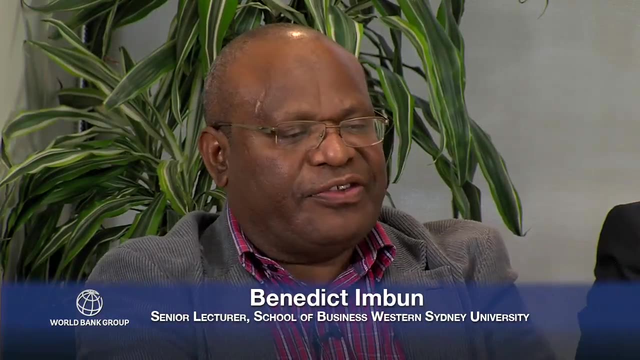 being put up by people with that, that we've seen 250 similar arrangements, but with decisive leadership, pragmatic leadership, Speaking to the people, Obviously probably in the 85%, oblivious to what happens around with bureaucrats with vision 250.. So what we need is some dynamic. 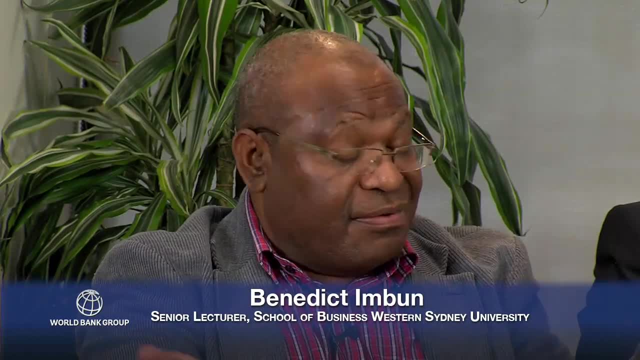 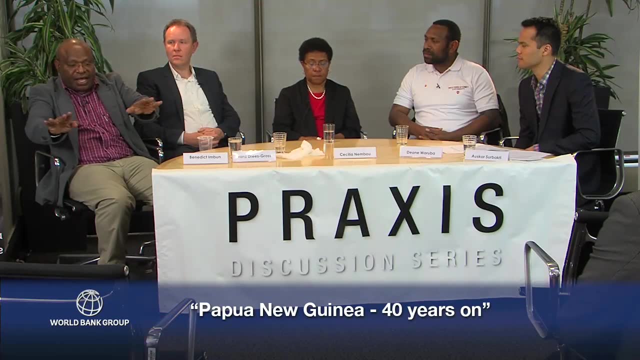 So that lead some good leadership. So that lead some good leadership, good leader, understanding the measures of the people where they live, in villages I mentioned, of the agriculture plot, where those mentalities need to be broken down, where people need to be absorbed into the more broader, you know, economy, formal economy That's. 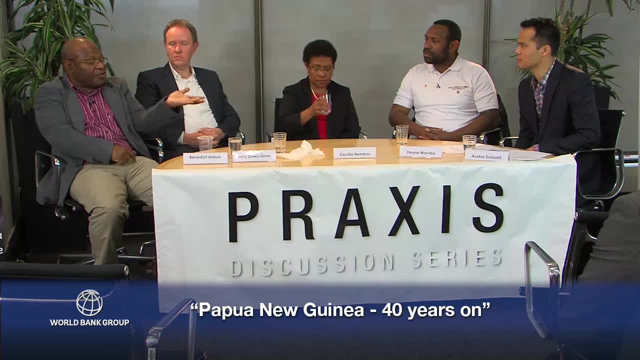 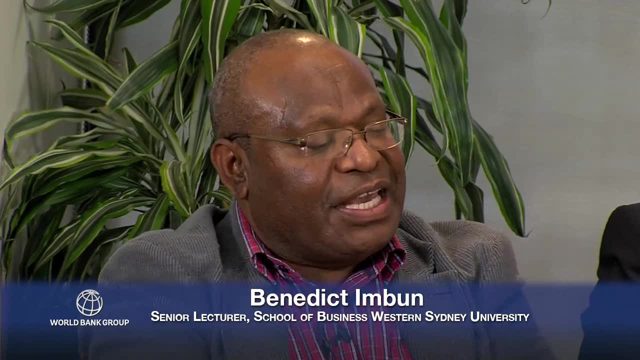 where the stumbling block is. Unless somebody taps into that and understands the people and preaches to them about how it means to be educated, means to earn a living and then bring up the kids and go forward, then I do not. after 40 years, probably there would. 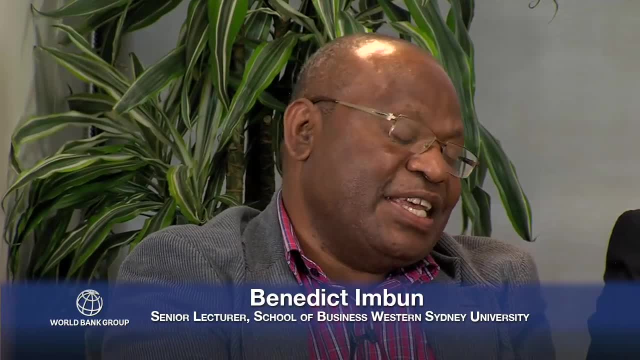 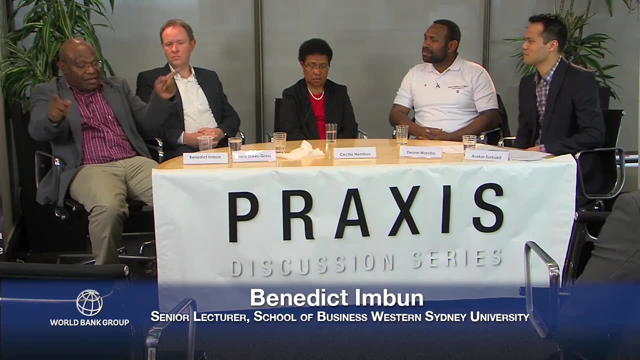 be another session here talking about what have we achieved in the last 80 years. So leadership is number one. I mean number one meaning we need to have some of those notable leaders that have turned their countries around. Papua New Guinea needs, by now, to come up with. 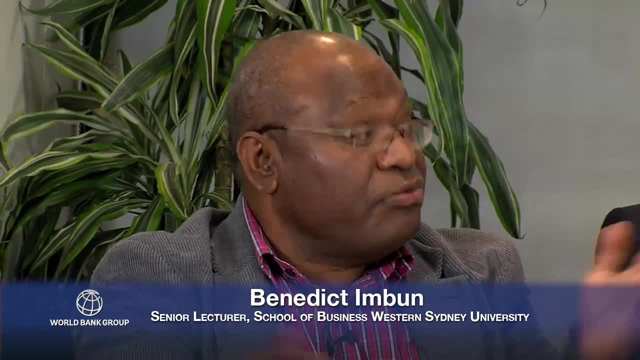 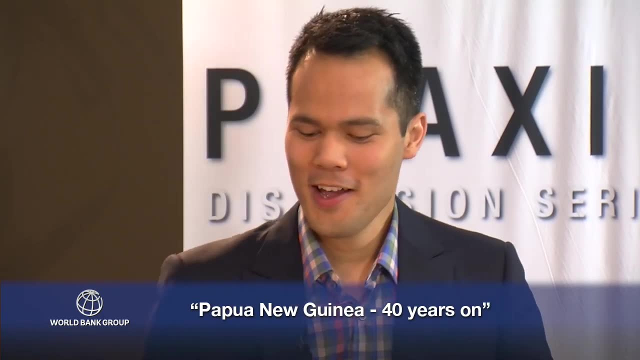 somebody single-handedly or a group of people to do that. Okay, Interesting times. Maybe we will have a discussion 40 years from now to see how it all went, Thank you. Thank you, But for now that does bring our discussion to an end. Can we please thank our panellists. 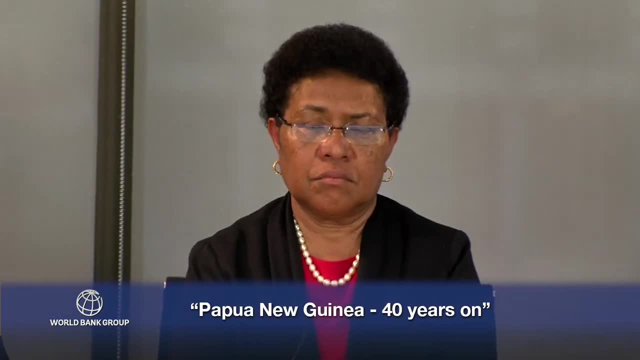 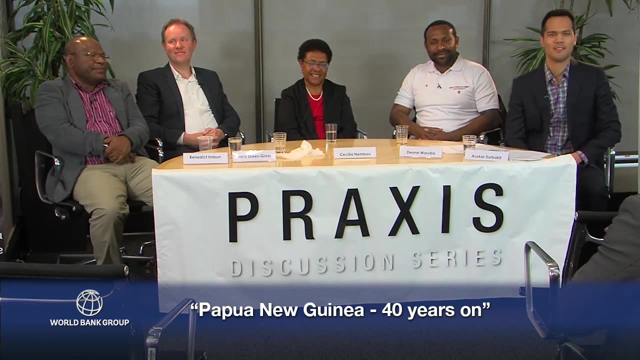 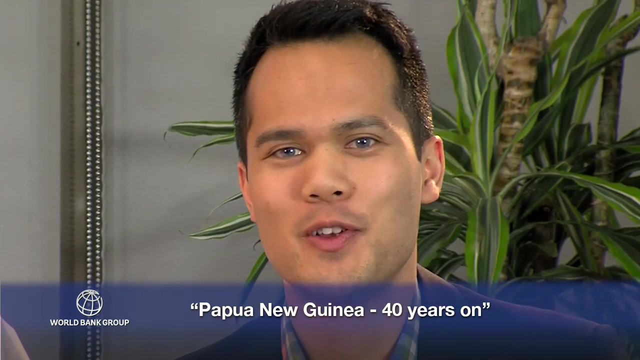 Benedict Imbun, France Dries-Gross, Cecilia Nembu and Dean Waruba. I'd also like to thank everyone joining us either here in Sydney or from afar, And remember you can view this or any of the other Praxis discussions at worldbankorg forward slash. 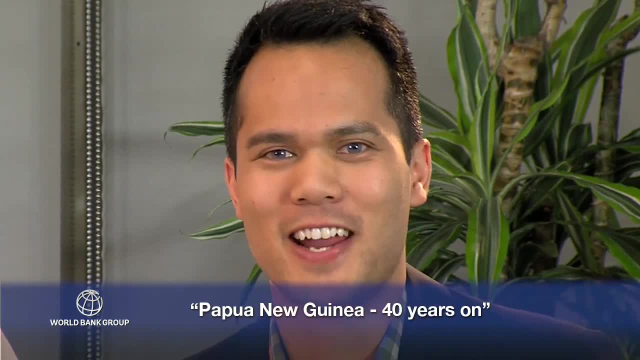 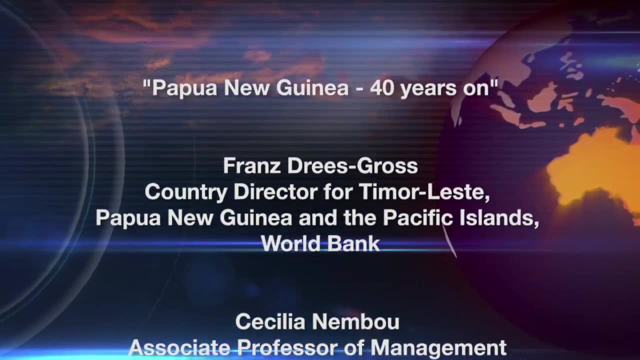 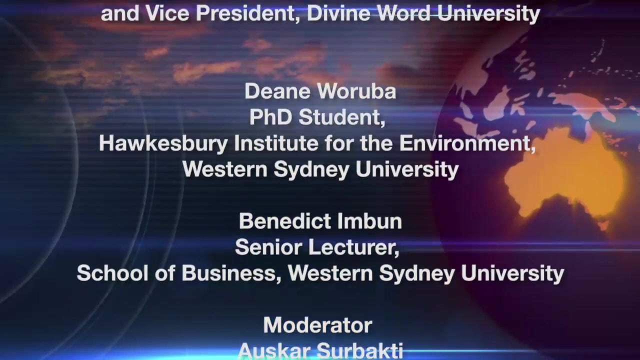 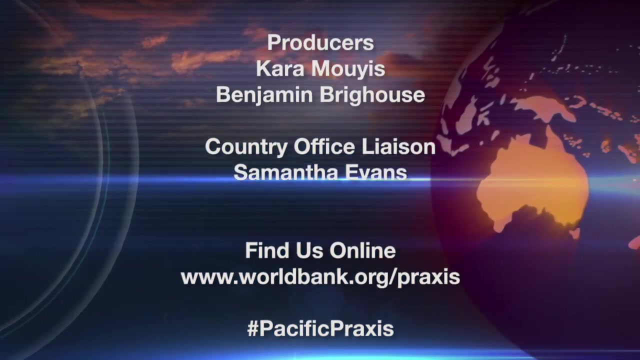 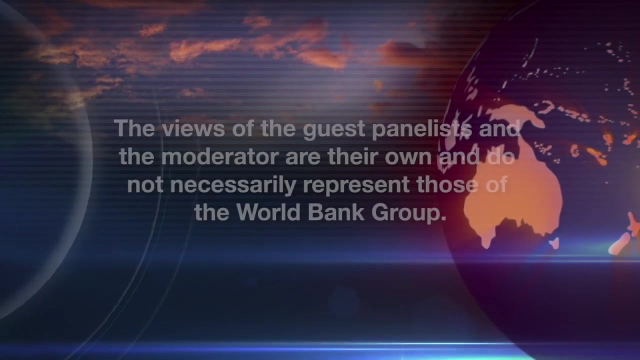 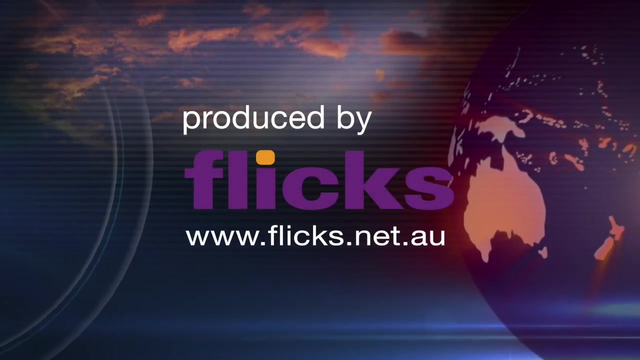 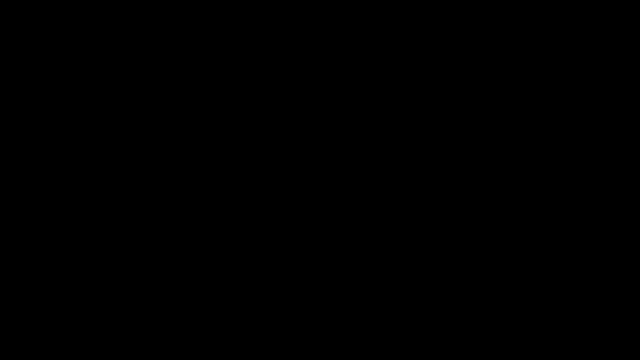 Praxis Until next time. I'm Oskar Sabakti. Thanks for your company. Bye for now. Bye, We'll be right back.